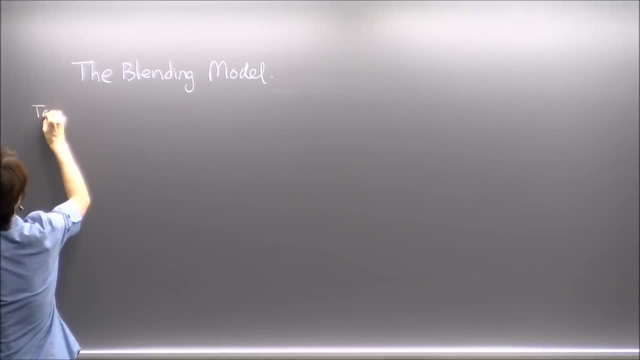 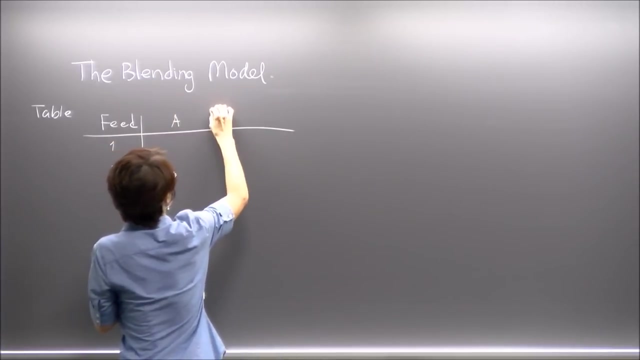 OK, so I'll just set up the table very briefly. probably I didn't have to do that, So OK. So a farmer is going to feed his stocks with two types of feeds- We call it 1 and 2. And they contain three different types of nutrients. 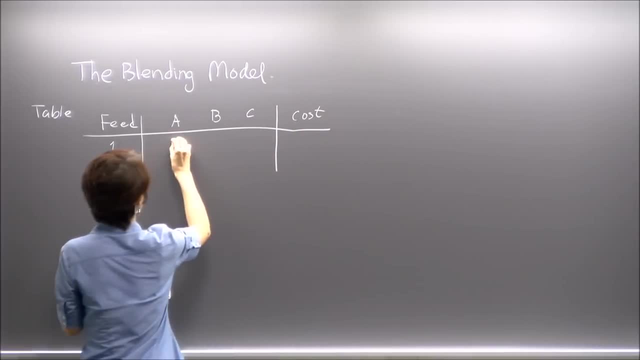 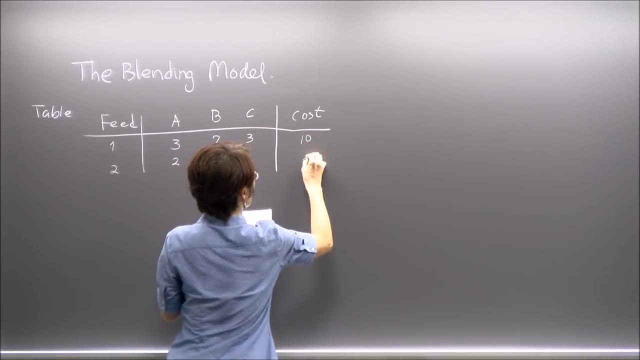 And each has a cost right. So we have this table: 3, 2, 7, 2, 3, 6,, 10, 4.. The cost is in cents And all these units, these are whatever unit per pound. 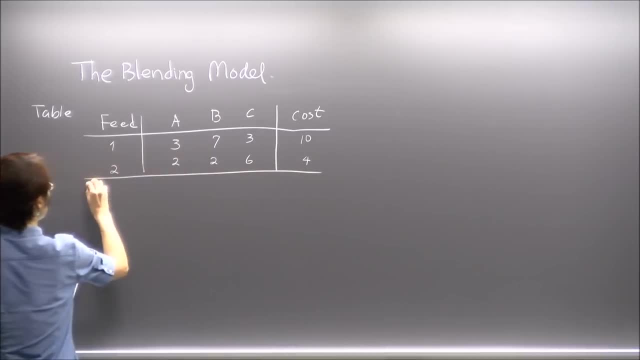 whatever, OK. And then there is a minimum value to be met for all the nutrients. So let me put this up: OK, so for each type of nutrients the daily minimum value has to be met. And then we have a problem model we set up. 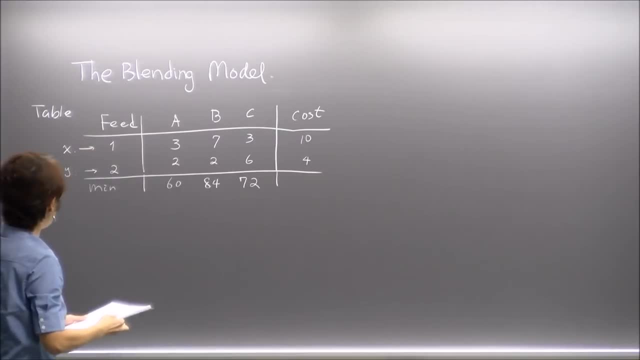 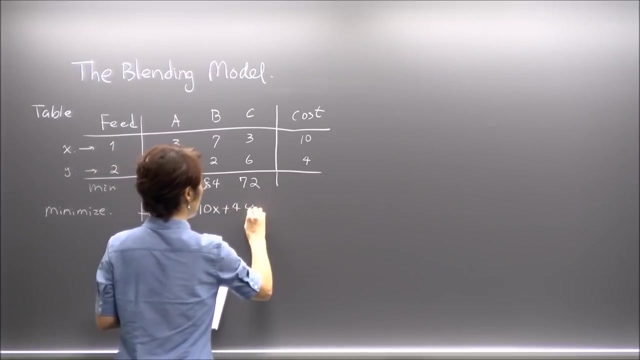 We call this x and we call this y. So our problem is the following: Minimize the cost f of x, y equals to 10x plus 4y, subject to the following constraint: We have three constraints coming from each column. 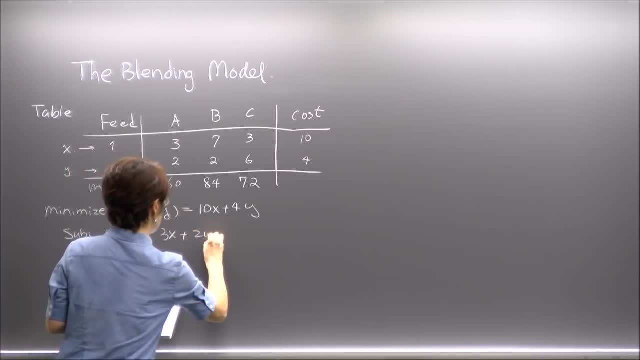 Let me write it up: 3x to y bigger than 60.. Sorry, 7x 4y Plus 2y bigger than 84.. 3x plus 6y bigger than 72.. OK, And also the non-negativity constraint. 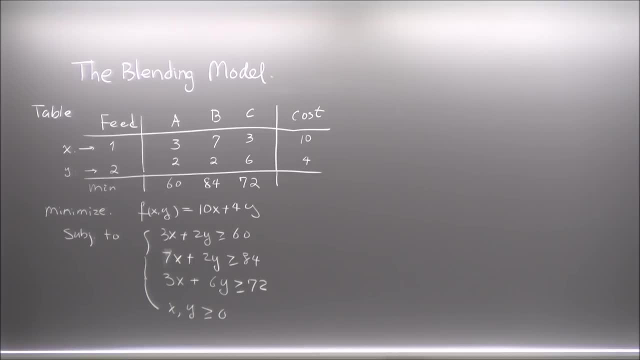 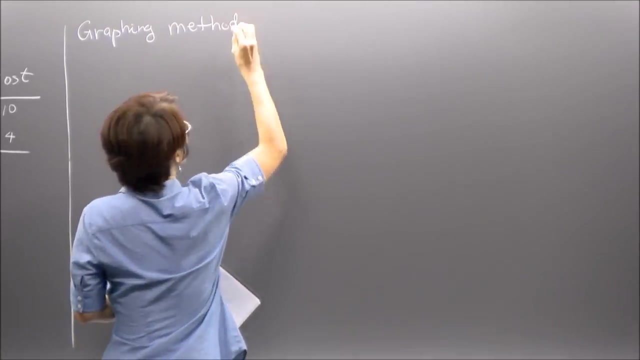 Can you see down there? OK, After the semester you have very good sitting posture. Always talk, Talk. OK, So we're going to solve this using graphing method. OK, We, and we will learn. we solidify our skill. 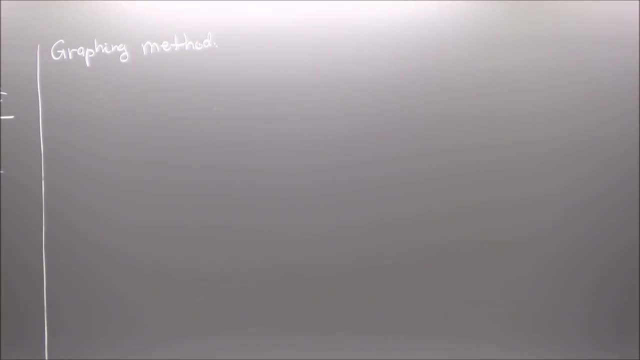 of this graphing method And probably something new we can learn from this example. OK, So we know these three constraints. We need to find the so-called feasible regions. OK, region. let me label these constraints as constraint A, B and C. Okay, so let's. 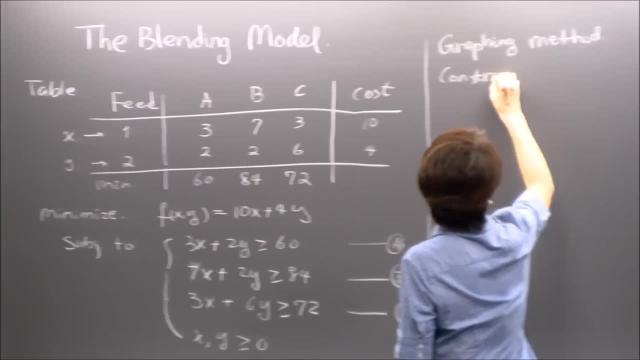 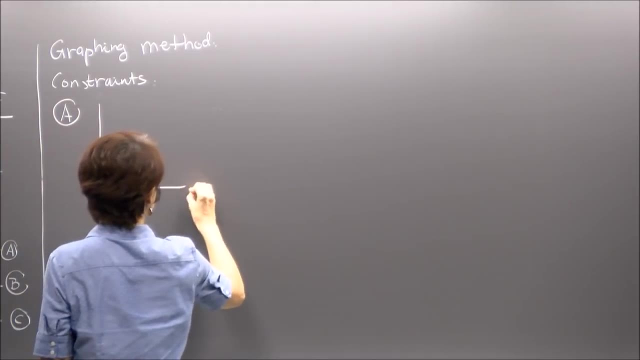 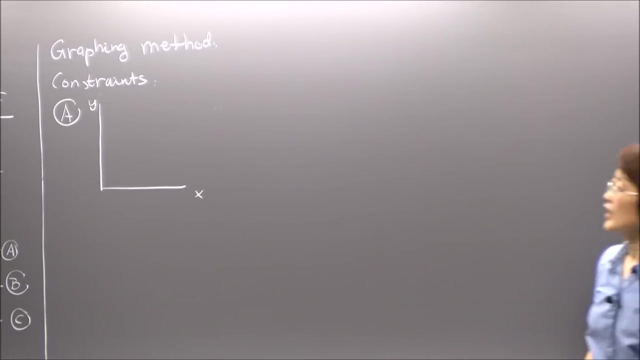 find feasible region for my constraints. So for A, let's draw. So I have X and Y, And you know I only consider the first quadrant, right, It's where they're positive. Okay, so it's the same thing What you have to do. well, you find the line for the. 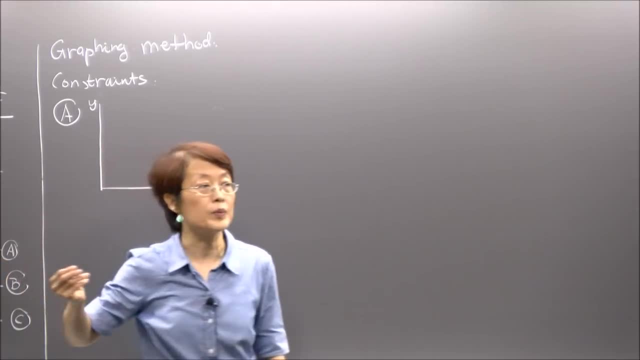 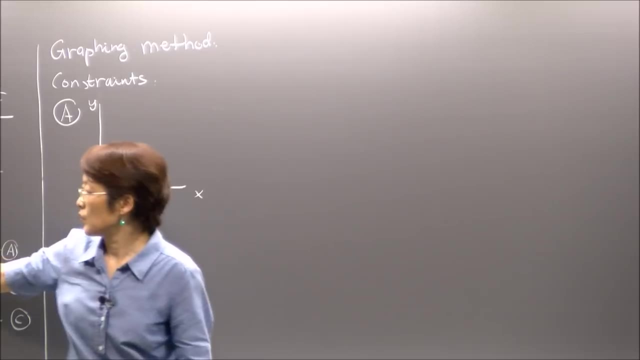 boundary of it, where you have the equal sign and the upside will be the region you want right And you find the two intercepts. Is that right? So the X intercept will be 60 over 3, whatever is in front of X, And the Y intercept will be 60. 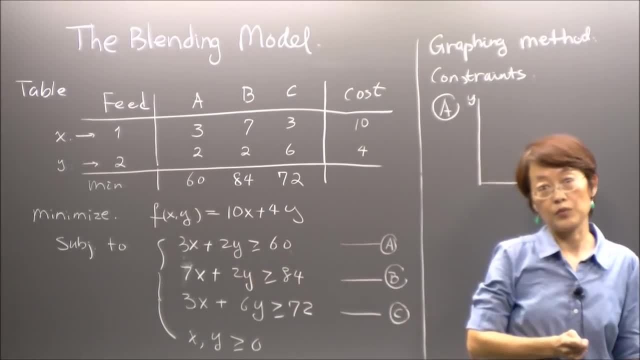 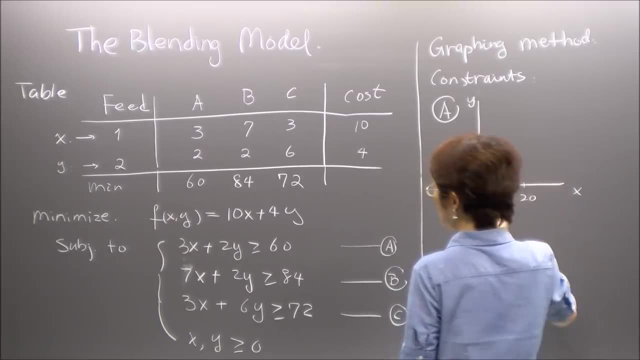 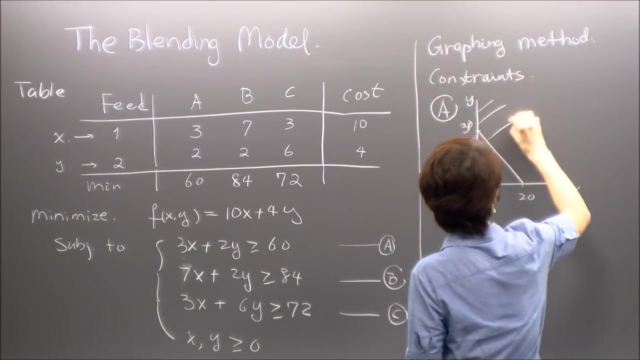 over 2, the coefficient in front of Y. Is that clear? So once you know that, it's quite smooth. So you have 20 here and 30 over there And then you draw a straight line and the region above. Is that okay? 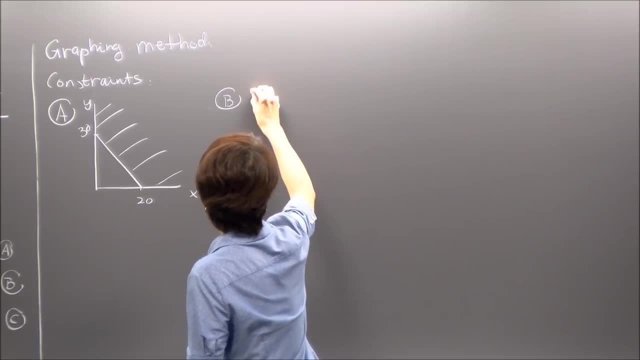 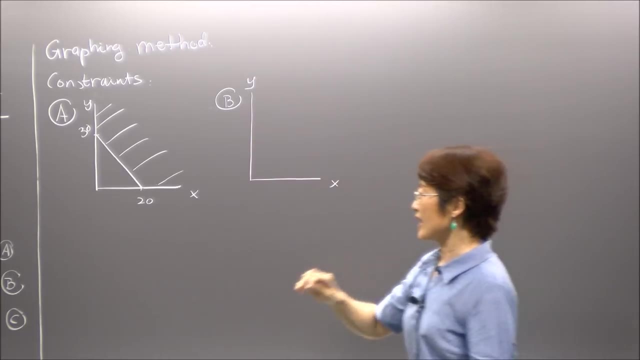 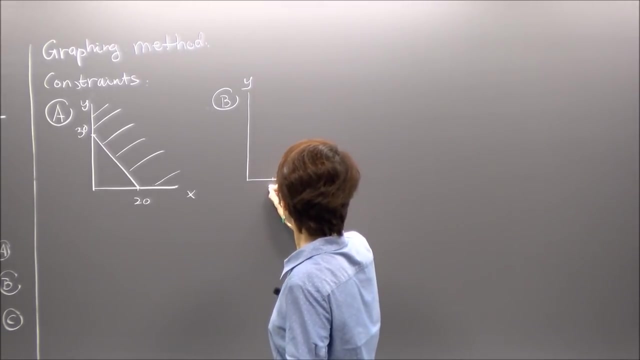 Okay, that's constraint A, And let's see constraint B. How would that be? So this is X and this is Y. So the X intercept will be 84 over 7, which is 12.. And the Y intercept is 84. 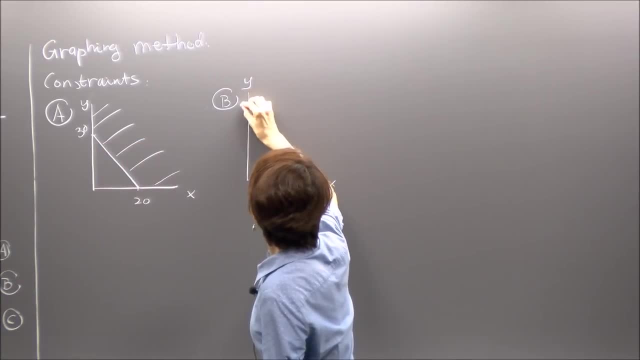 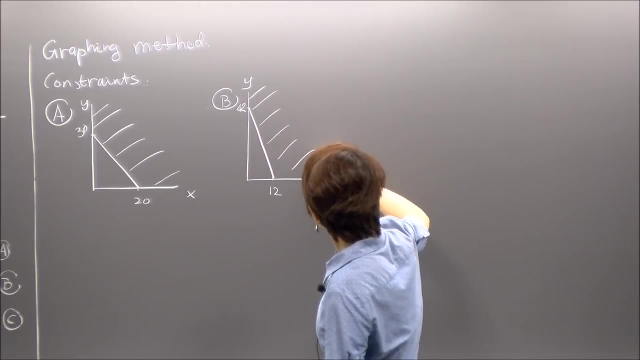 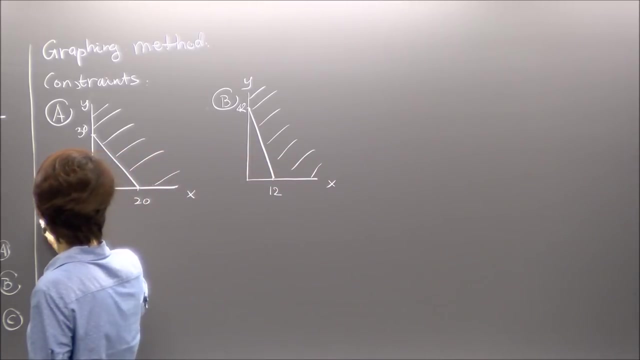 over 2. That gives me 42. Is that right? And I connect this and I have a straight line And the region above satisfies my constraint. right Number B, Is that okay? And then C: Okay, it's repetitive now. Okay, so. 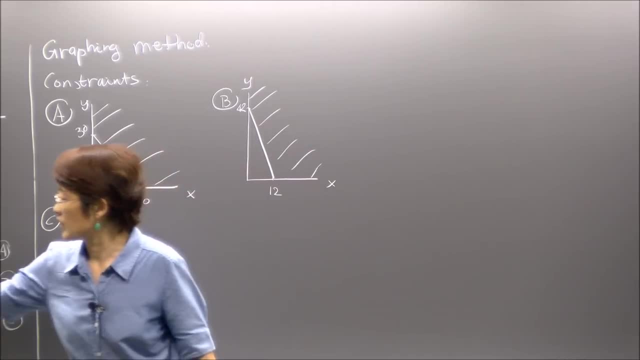 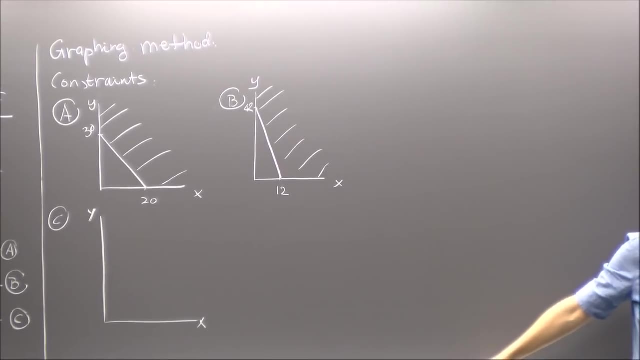 the X intercept will be 72 over 3.. What does that end up with? What's 72 over 3?? You guys play this card game called make 24 with four cards- Not enough. I played so much in my childhood that 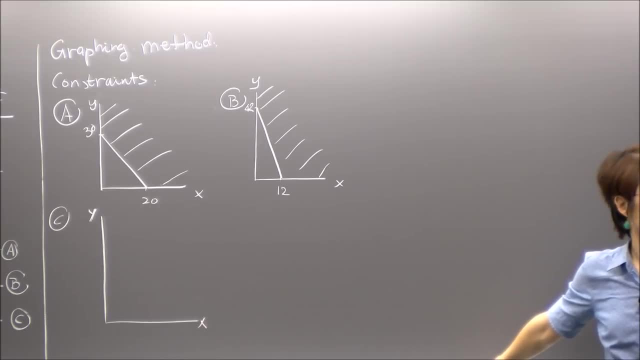 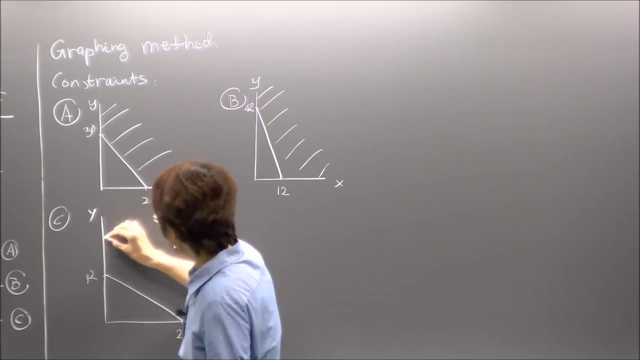 I'm very sensitive to any number that ends 24.. Okay, it's 24.. Is that right? And the Y intercept 72 over 6,, which is half of that, is 12.. Okay, so I connect these two and I have. 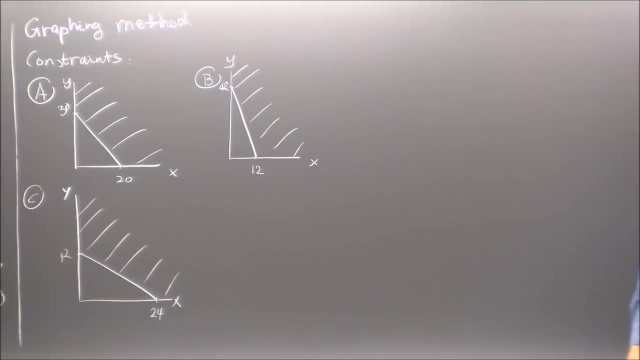 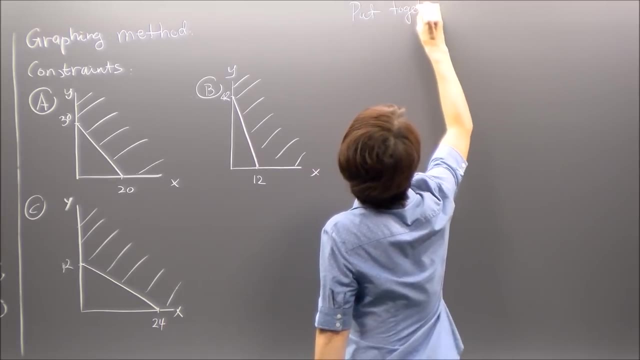 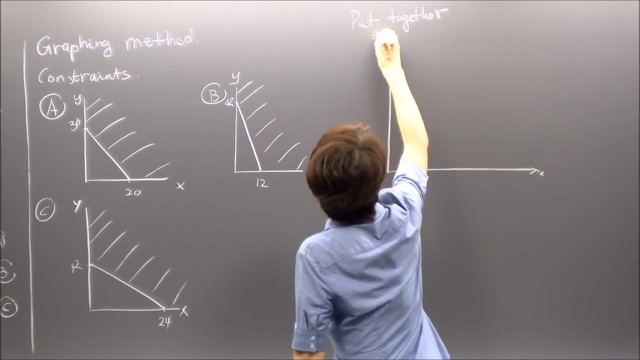 this region, Then I need to put them all together. Is that right? So, put together, I need to find the feasible region. So let's put this together: This is X and this is Y, So I have three different values, for X is 12,. 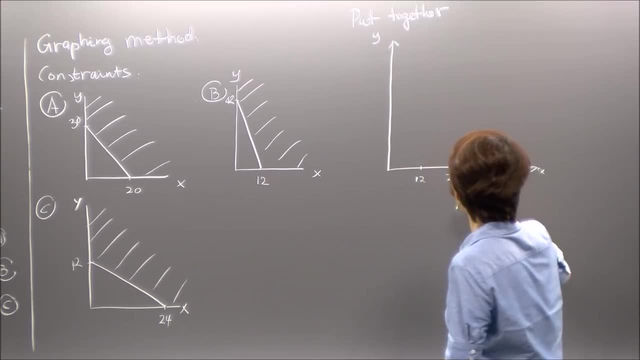 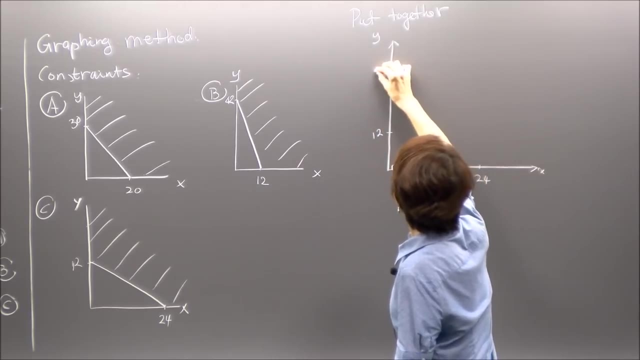 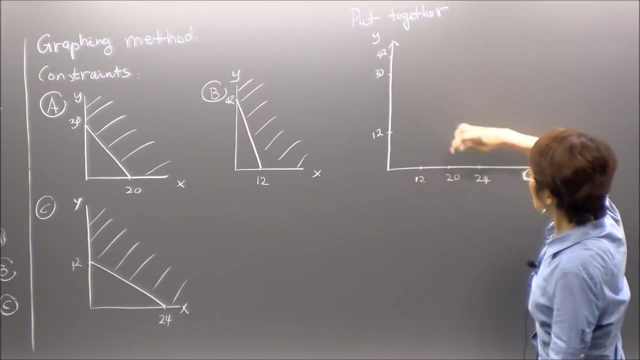 20, 24.. Not really up-to-scale, but okay. So I have 12,, 30,, 42.. Okay so, let's draw For the constraint A. I have from 30 to 20.. So 50, 2.. 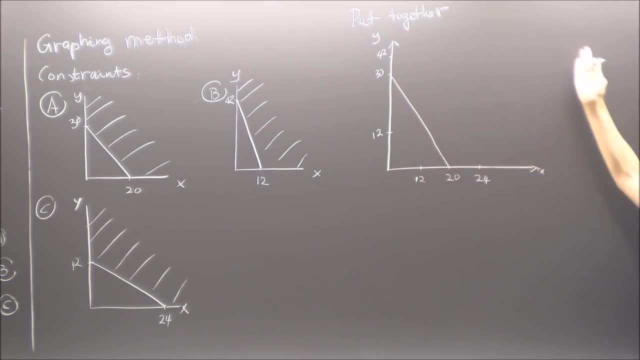 so that's, that's the boundary, it's the part above it. and then for constraint B, I have 42 to 12. I will draw that line, so it's the part above that right. and then, for constraint C, I have from 12 to 24. okay, this is really not good the part. 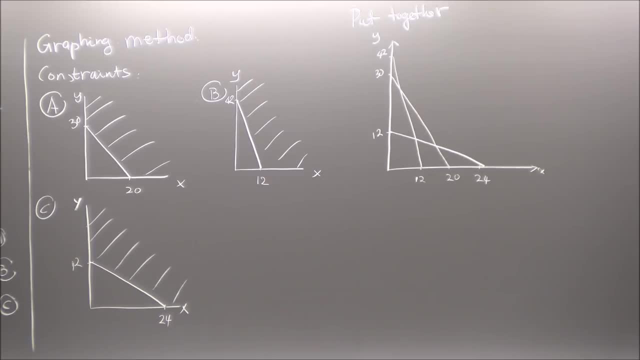 above that line. so what will be my feasible region? how do I find out? the feasible region should satisfy all these three constraints, right? how would I figure out in this region, what will it be? it means it has to be above each of these lines, right? so you start from here. 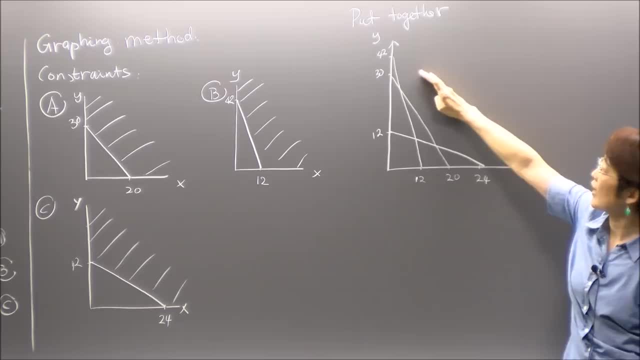 right, so you start from here. right, so you start from here. of course I'm above all those lines. and then you, of course, I'm above all those lines, and then you, of course I'm above all those lines, and then you go down each direction, you go as. 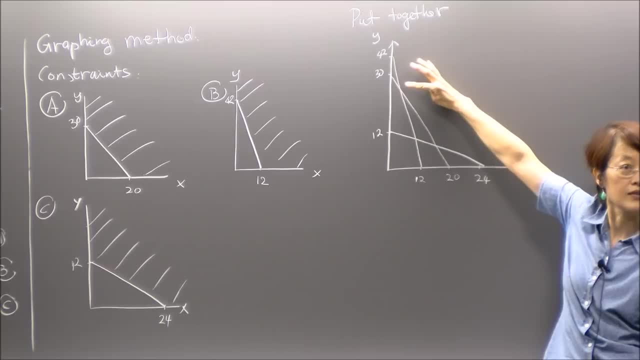 go down each direction you go, as go down each direction you go as soon as you hit a line you can't cross is soon as you hit a line you can't cross is soon as you hit a line you can't cross. is that clear? so what will the boundary? 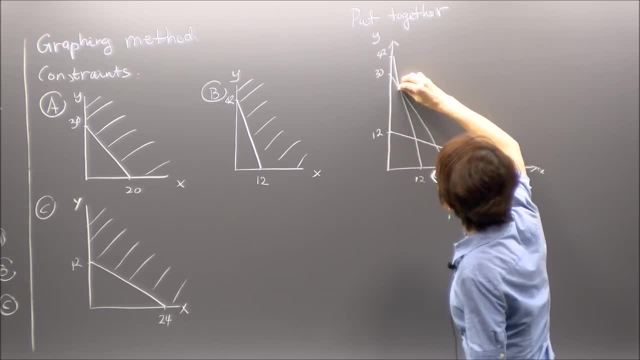 that clear. so what will the boundary that clear? so what will the boundary of this region? be well, this part right as of this region. be well, this part right as of this region. be well, this part right. as soon as you hit a line, you can't. soon as you hit a line, you can't. 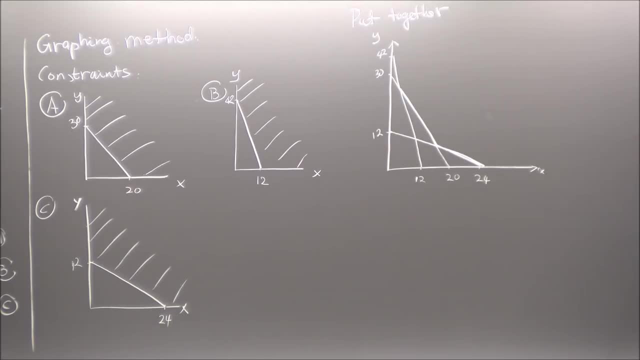 soon as you hit a line you can't cross, because then you will violate some cross, because then you will violate some cross, because then you will violate some constraint. okay, so it's this region. so constraint. okay. so it's this region so constraint. okay, so it's this region, so let's shade it just above here, okay, so? 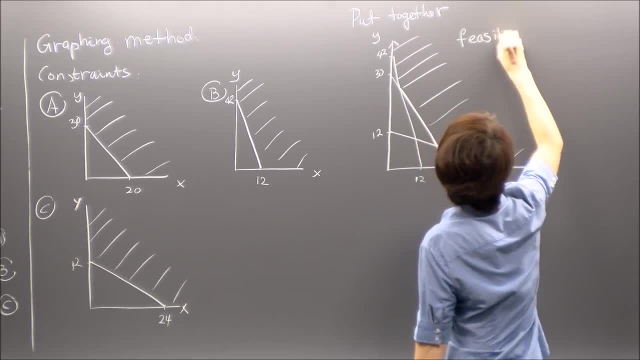 let's shade it just above here, okay. so let's shade it just above here, okay. so that is fine feasible region. is that that is fine feasible region? is that that is fine feasible region? is that clear, mm-hmm, clear, mm-hmm, clear, mm-hmm. shall we be able to find feasible regions? 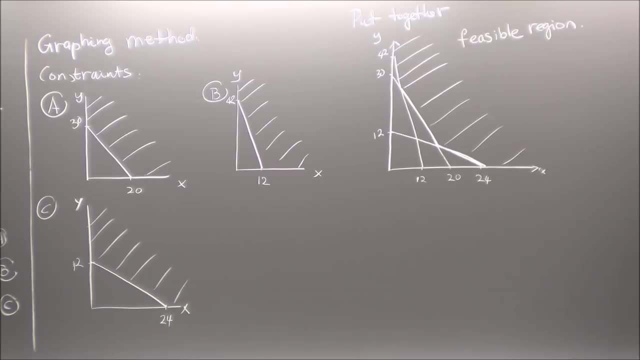 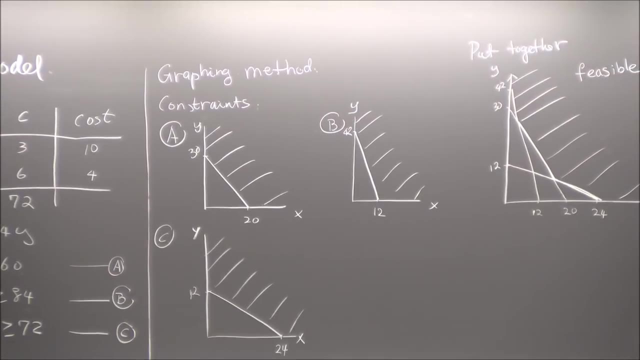 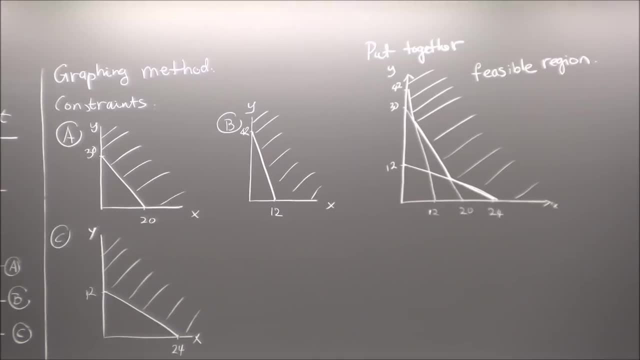 aim at solving this problem. so that's the aim at solving this problem. so that's the feasible region. remember the example feasible region. remember the example feasible region. remember the example we had last time we made some observations we had last time we made some observations we had. last time we made some observations, we found out that the, the, 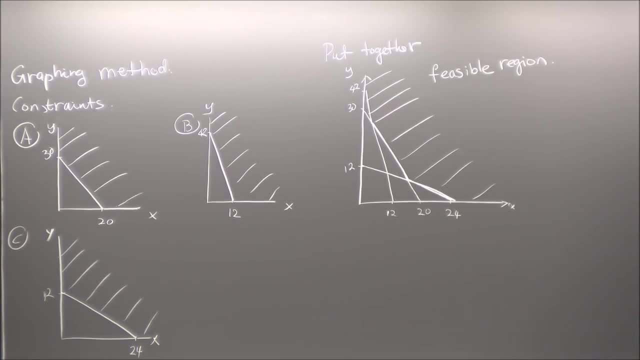 we found out that the the we found out that the the minimum was attained at the corner right. a vertex minimum was attained at the corner right. a vertex minimum was attained at the corner right, a vertex of that feasible region. probably of that feasible region. probably of that feasible region. probably that is true here also, we are expecting it. 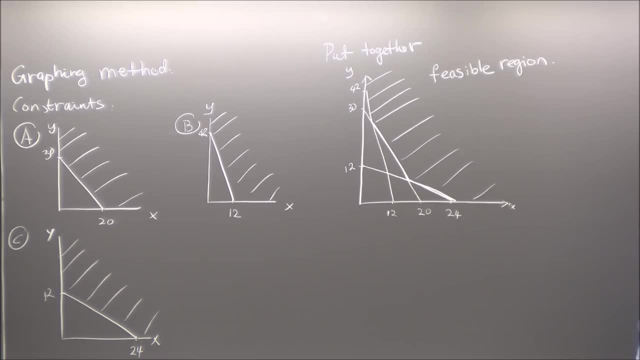 that is true. here also, we are expecting it. that is true here also, we are expecting it. so it makes sense to locate all those. so it makes sense to locate all those. so it makes sense to locate all those vertexes, all those corners right so, vertexes, all those corners right so. 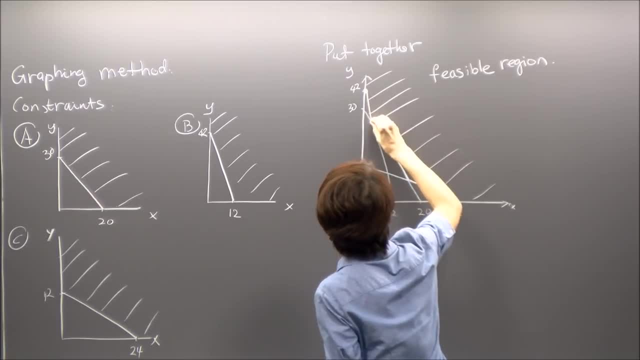 vertexes, all those corners right. so let's say I did the work, I found out the. let's say I did the work, I found out the. let's say I did the work, I found out the coordinate of all these corners. are we coordinate of all these corners, are we? 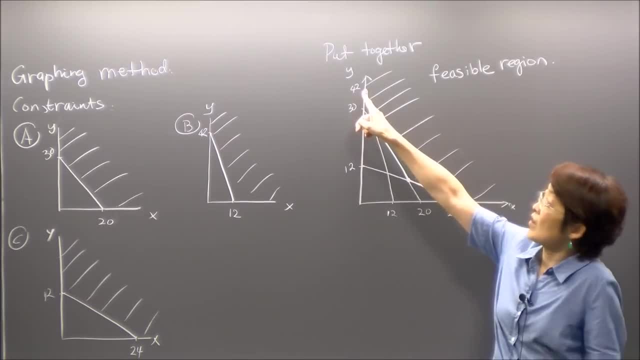 coordinate of all these corners. are we able to do that? this one is obvious. able to do that? this one is obvious. able to do that. this one is obvious. that's the intercept. so this point will. that's the intercept. so this point will. that's the intercept. so this point will be: X is 0, Y is 42 and this point is. 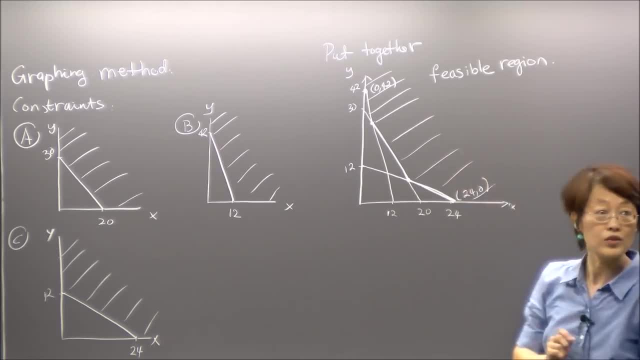 be X is 0, Y is 42 and this point is: be X is 0, Y is 42. and this point is also obvious: X is 24, Y is 0. right to also obvious: X is 24, Y is 0. right to also obvious: X is 24, Y is 0. right to find the corner here you need to solve. 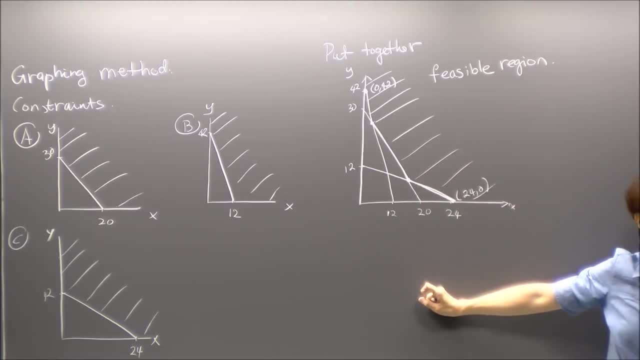 find the corner here you need to solve, find the corner here you need to solve the equation of this line and that line. the equation of this line and that line, the equation of this line and that line simultaneously, is that right to unknown simultaneously? is that right to unknown? 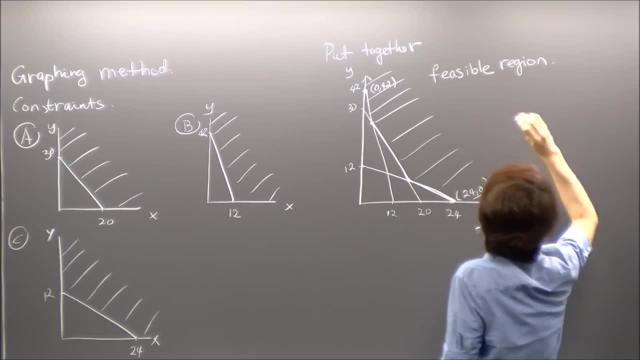 simultaneously. is that right to unknown to equation? we know how to do it, so it to equation. we know how to do it, so it to equation. we know how to do it, so it involves some work. so okay, so let's say: involves some work. so okay, so let's say: 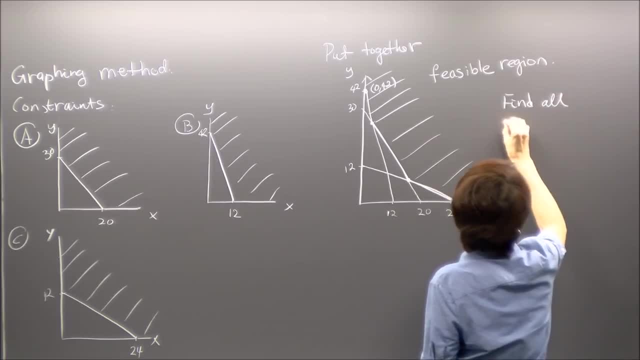 involves some work, so okay. so let's say: I did this work, I find all corners okay. I did this work, I find all corners okay. I did this work, I find all corners okay. so this part I did so let me label so. so this part I did, so let me label so. 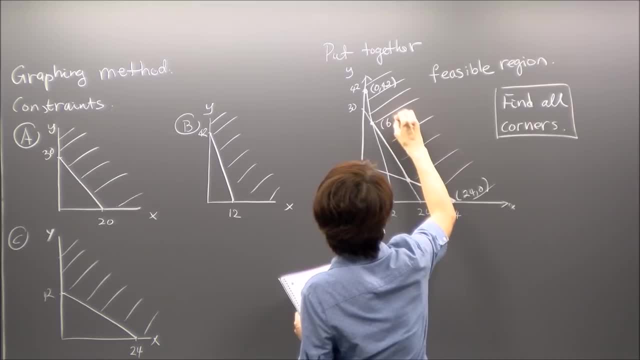 so this part I did. so let me label. so what I have here is 621, and this one is what I have here is 621, and this one is what I have here is 621 and this one is 18 and 3. okay, so I have four corners. 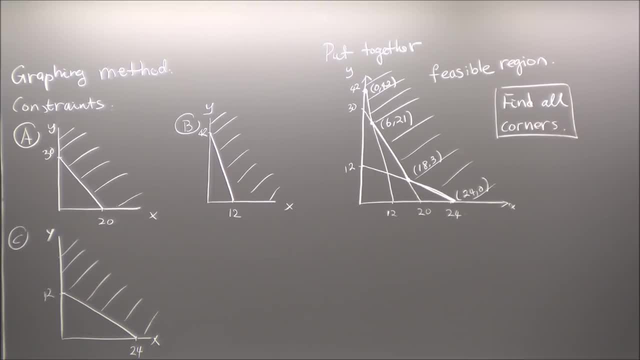 18 and 3. okay, so I have four corners. 18 and 3- okay, so I have four corners. okay, so where would the cost function? okay, so, where would the cost function? okay, so, where would the cost function reach its minimum? so let's look at the. 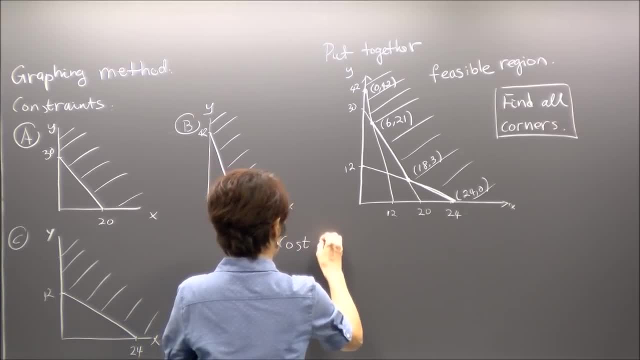 reach its minimum. so let's look at the reach its minimum. so let's look at the cost. cost function is a linear function. cost function is a linear function. cost function is a linear function. his 10x plus 4y, and then we know I need to. 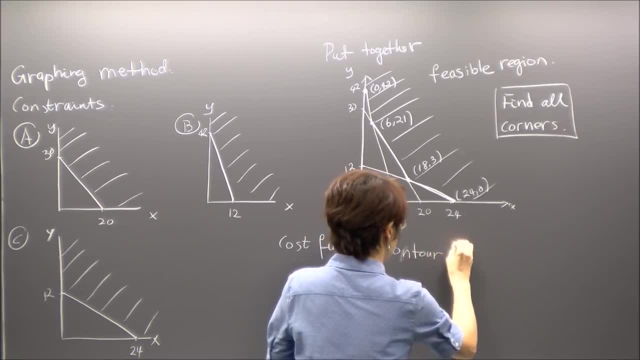 his 10x plus 4y, and then we know I need to his 10x plus 4y, and then we know I need to find out the contour lines. is that find out the contour lines? is that find out the contour lines? is that right? so these are the lines where um. 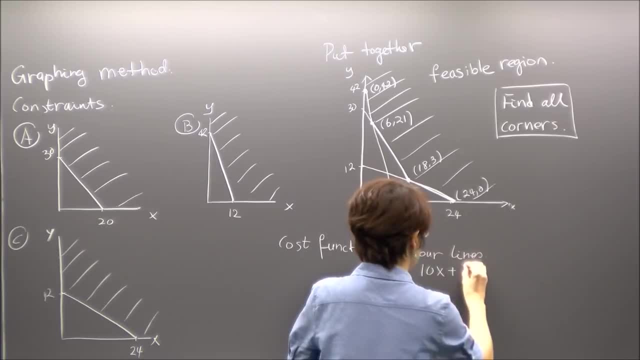 right. so these are the lines where um right. so these are the lines where um the cost function equals to a constant. the cost function equals to a constant. the cost function equals to a constant. for what? let's say K is a constant. so for what? let's say K is a constant. so. 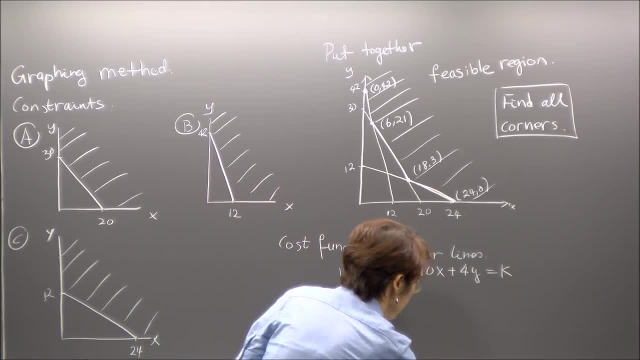 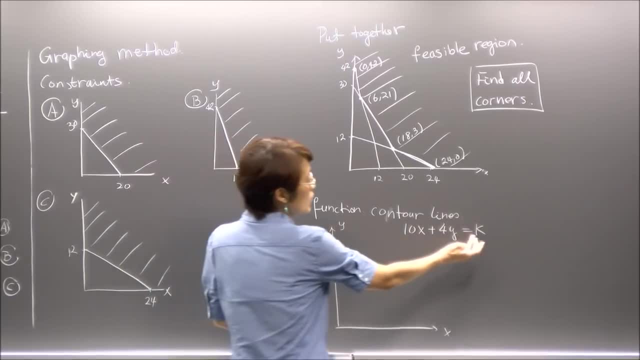 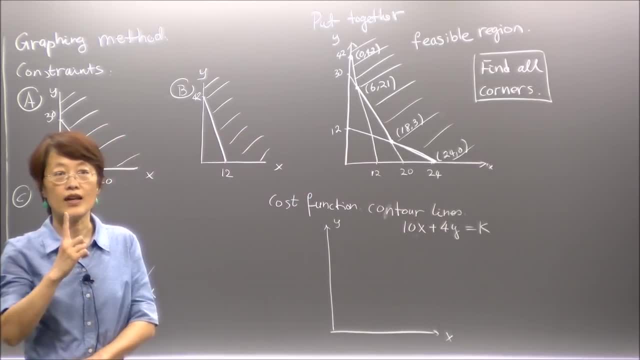 then you will have X: intercept will be 4y intercept will be 10. that will be one. 4y intercept will be 10. that will be one. 4y intercept will be 10. that will be one of the contour lines right. so 4 here, 10. 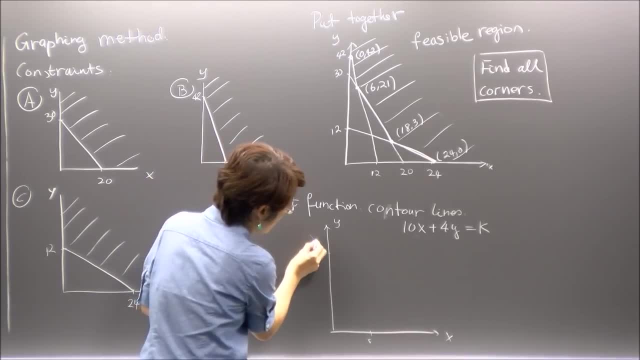 of the contour lines, right, so 4 here, 10 of the contour lines, right, so 4 here, 10 here. so what's important, you know it's here. so what's important, you know it's here. so what's important, you know it's the slope, so it's a straight line going. 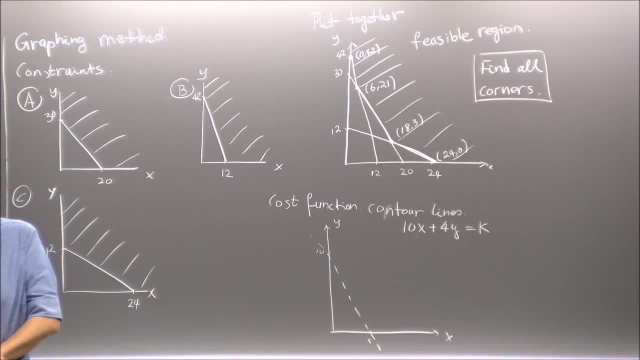 the slope. so it's a straight line going the slope, so it's a straight line going through these two points. and you know, through these two points, and you know, through these two points, and you know all of them shall be parallel to each, all of them shall be parallel to each. 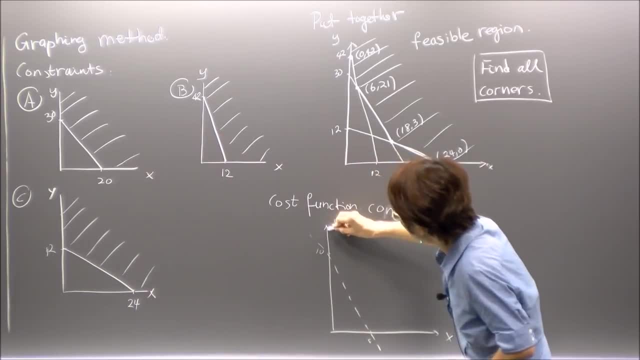 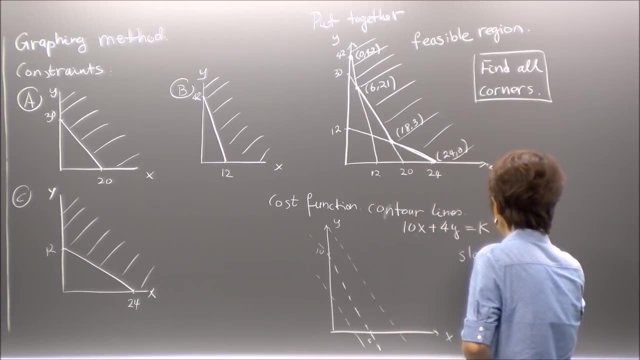 all of them shall be parallel to each other. right that situation is unchanged. other right that situation is unchanged. other right that situation is unchanged. so I will have a bunch of parallel, so I will have a bunch of parallel, so I will have a bunch of parallel lines. so I know the slope of all these. 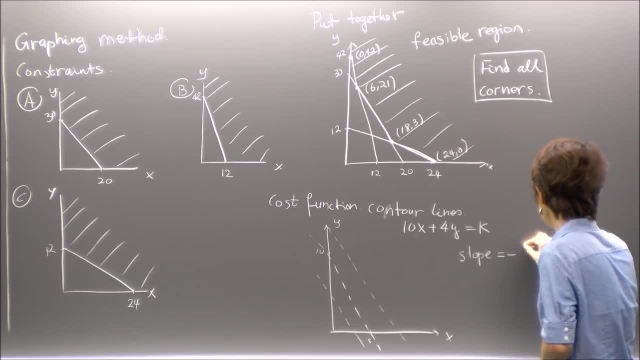 lines. so I know the slope of all these lines. so I know the slope of all these should equal to negative 10 over 4. is. should equal to negative 10 over 4 is. should equal to negative 10 over 4. is that right? and then you need to figure. 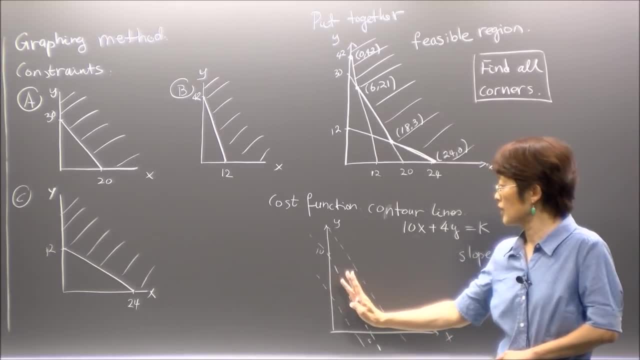 that right, and then you need to figure that right. and then you need to figure out: as I move from one control line to out, as I move from one control line to out, as I move from one control line to the other, will the K increase or the other? will the K increase or? 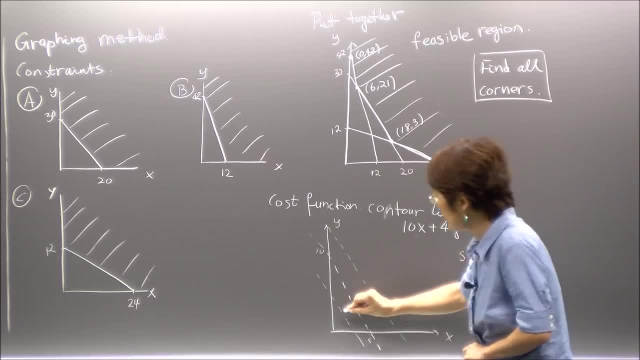 the other, will the K increase or decrease, right? so let's say: if I move, decrease, right. so let's say, if I move, decrease right. so let's say, if I move like up, like that from this line, I move, like up, like that from this line, I move. 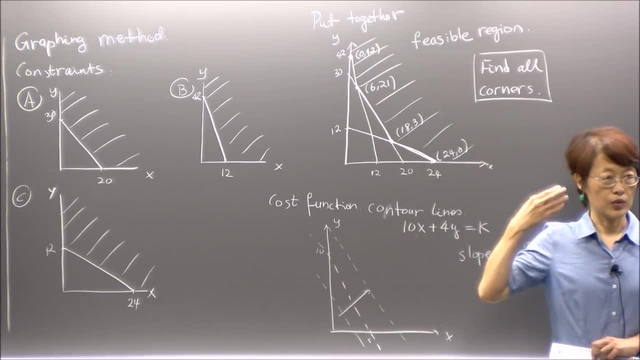 like up, like that: from this line I move to the parallel line that's above it, in to the parallel line that's above it, in to the parallel line that's above it. in that direction, will the K increase or that direction? will the K increase or that direction, will the K increase or decrease? so if I move in this direction, 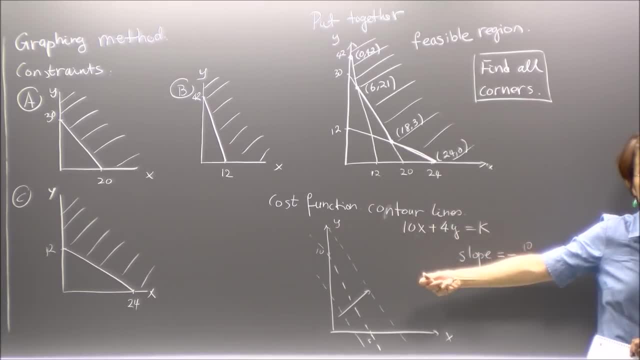 decrease. so if I move in this direction, decrease. so if I move in this direction, X and Y bless you will both increase. X and Y bless you will both increase. X and Y bless you will both increase. is that right? and the Sun shall grow, is it? is that right and the Sun shall grow, is it? 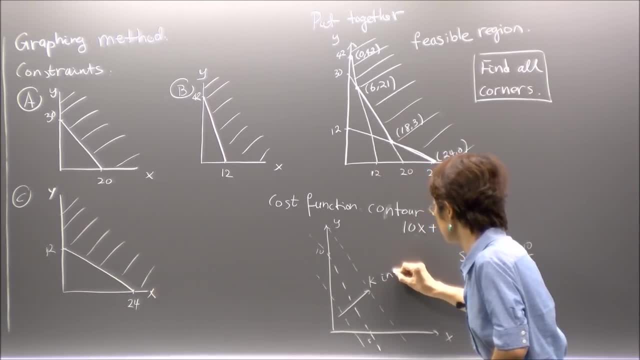 is that right? and the Sun shall grow. is it clear? so in this direction, K increases clear. so, in this direction, K increases clear. so in this direction, K increases. okay, so, okay. so K is increasing in that, okay, so, okay. so K is increasing in that, okay, so, okay. so K is increasing in that direction. and keep in mind for this. 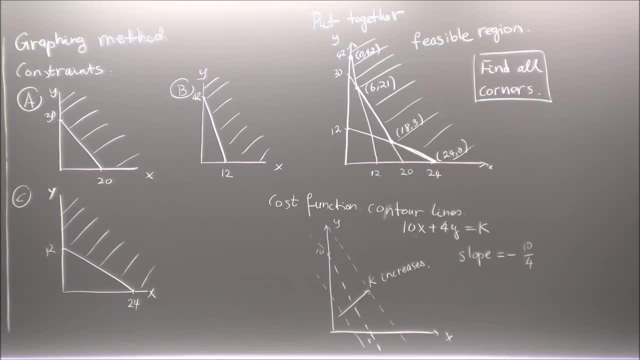 direction and keep in mind for this direction and keep in mind for this problem. we are trying to minimize that problem. we are trying to minimize that problem. we are trying to minimize that value. so we will try to stick to the value. so we will try to stick to the. 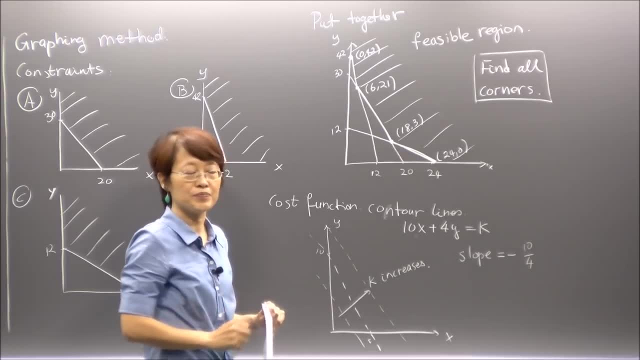 value. so we will try to stick to the lower part if possible, not moving up too lower part, if possible, not moving up too lower part if possible, not moving up too much right. as much as possible, so a way. much right, as much as possible, so a way. 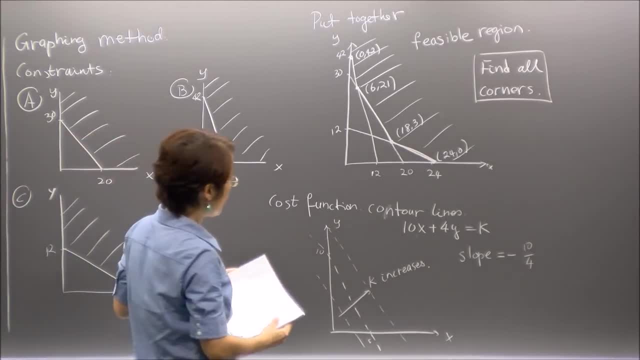 much right, as much as possible. so a way of solving this, of solving this, of solving this will be so you know all these contour will be. so you know all these contour will be. so you know all these contour lines are parallel lines you could take. lines are parallel lines you could take. 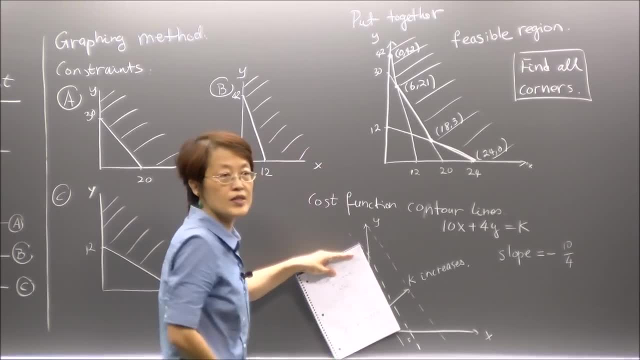 lines are parallel lines. you could take a ruler: copy this shape and the slope. a ruler: copy this shape and the slope. a ruler: copy this shape and the slope here of this line and then you come here of this line, and then you come here of this line and then you come here with this slope from the lowest. 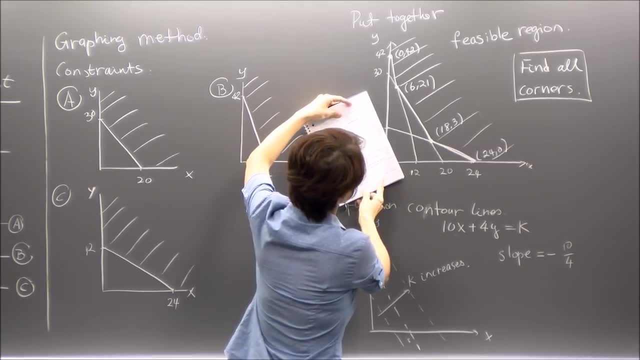 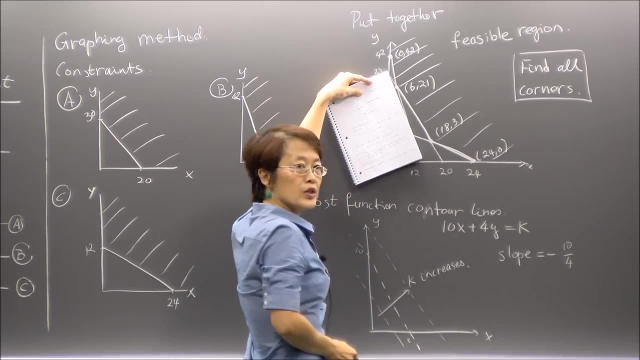 here with this slope from the lowest, here with this slope from the lowest possible point, and you, you move it possible point and you, you move it possible point and you, you move it parallely up until somewhere you touch parallely, up until somewhere you touch parallely, up until somewhere you touch the feasible region. there you find your. 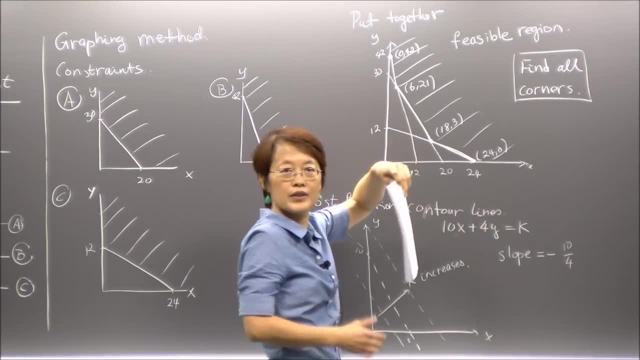 the feasible region. there you find your the feasible region, there you find your minimum. do we see that minimum? do we see that minimum? do we see that? we agree mm-hmm. because once you touch we agree, mm-hmm. because once you touch we agree, mm-hmm. because once you touch the feasible region, then that point will. 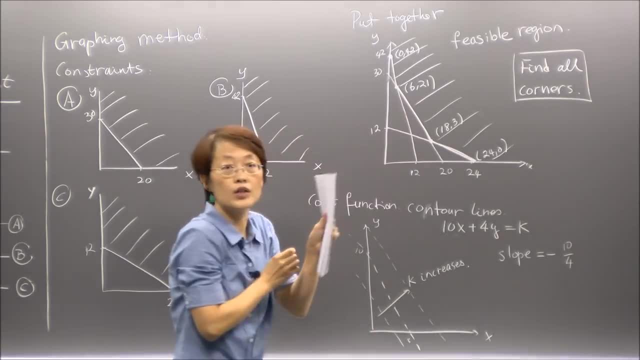 the feasible region, then that point will the feasible region, then that point will give you the minimum, because if you move give you the minimum, because if you move give you the minimum, because if you move further into it, K will increase and it, further into it, K will increase and it. 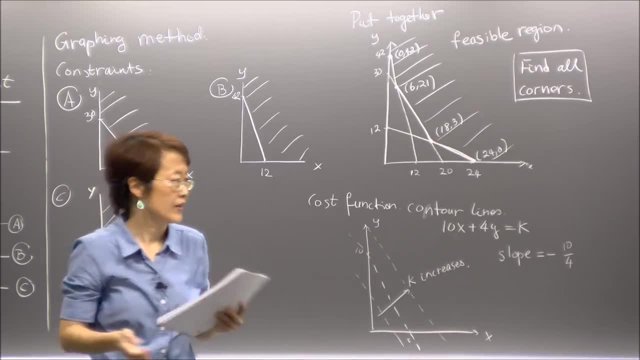 further into it, K will increase and it gets bigger. that's not the minimum does gets bigger. that's not the minimum does. gets bigger. that's not the minimum. does that make sense? so let's draw a couple that make sense. so let's draw a couple that make sense. so let's draw a couple of parallel lines. so if I do that, I start. 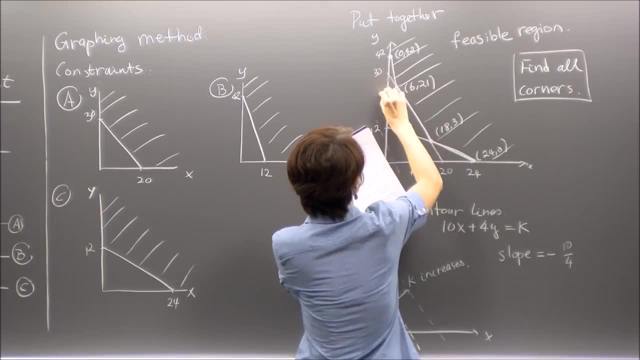 of parallel lines. so if I do that, I start of parallel lines. so if I do that, I start from here, that's a parallel line, and from here, that's a parallel line, and from here that's a parallel line, and then move further up, and then I move. 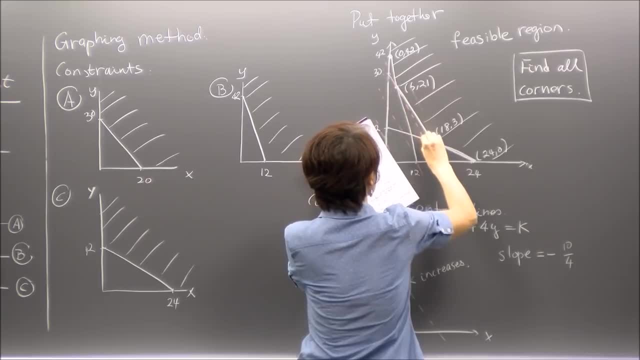 then move further up, and then I move, then move further up, and then I move further up and I find out this will be further up, and I find out this will be further up, and I find out this will be the first one with the smallest K value. 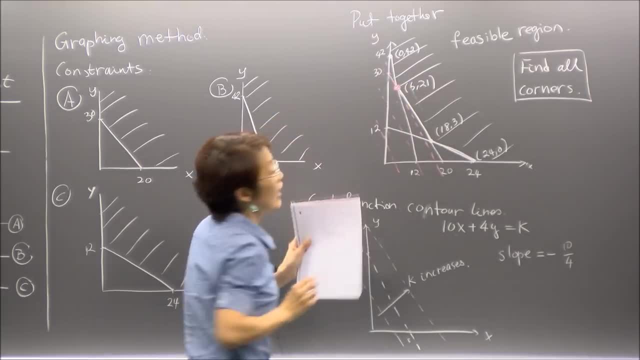 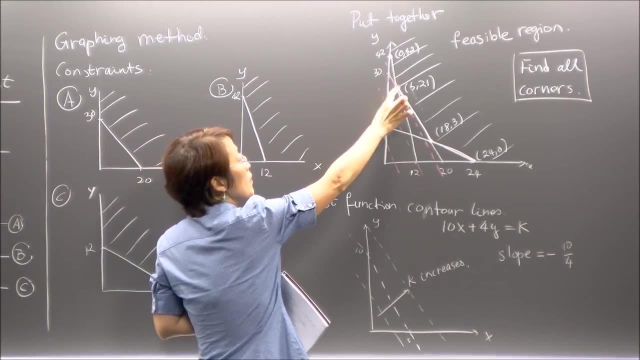 the first one with the smallest K value. the first one with the smallest K value that touches the feasible region at that? that touches the feasible region at that. that touches the feasible region at that point. is that clear point? is that clear point? is that clear? so at this point, my cost shall be the: 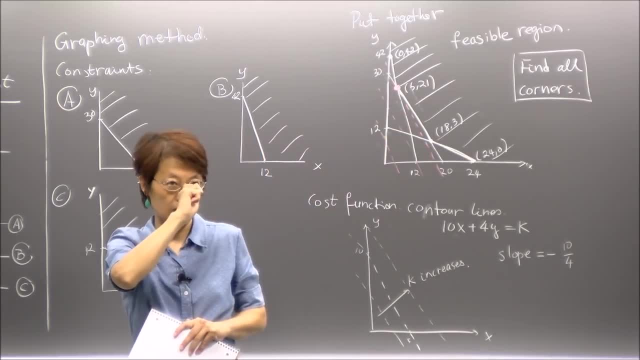 so, at this point, my cost shall be the. so, at this point, my cost shall be the minimum. and the point is still in the minimum and the point is still in the feasible region. Is that okay? Okay, so that is what we. let's write it out. So we find out that 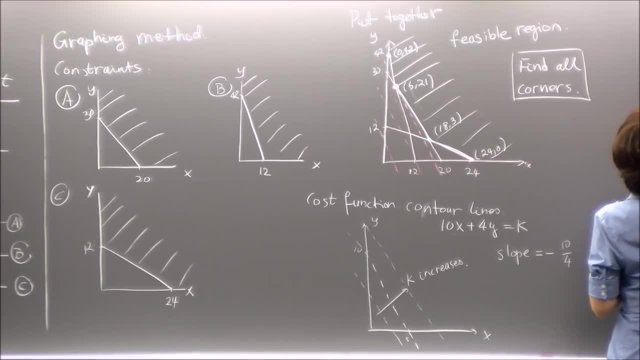 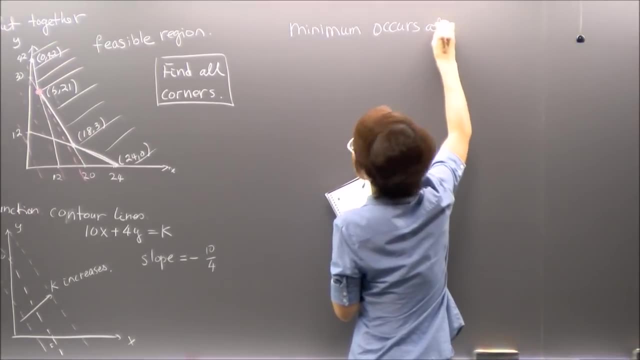 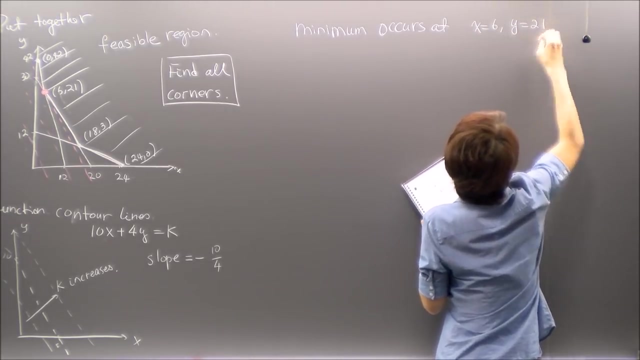 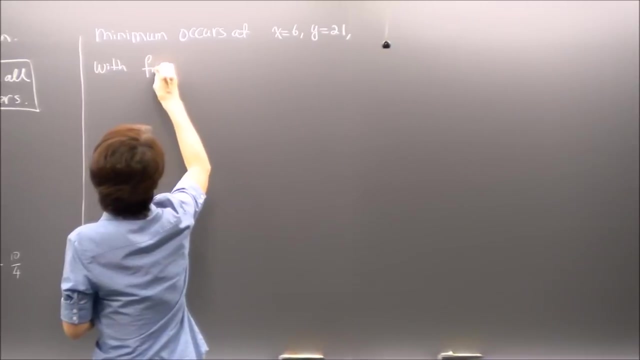 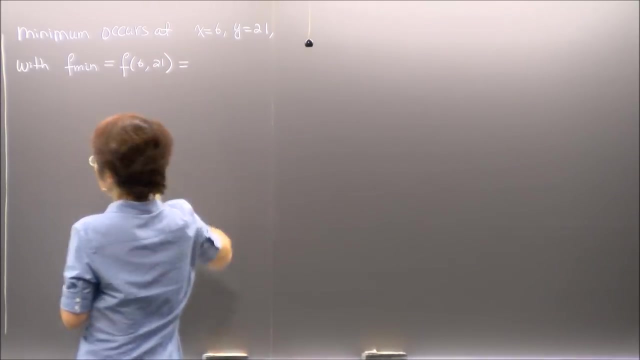 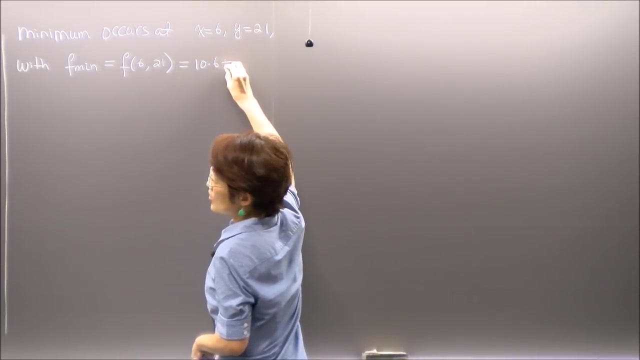 the minimum occurs at that point where x is 6,, y is 21,. and what is the minimum value? So f min equals to f at 6. And 21.. And if you put in those two numbers and figure out so 10 times 6 plus 4 times 21,, 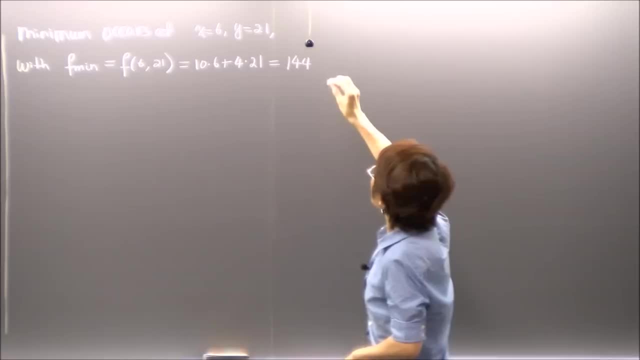 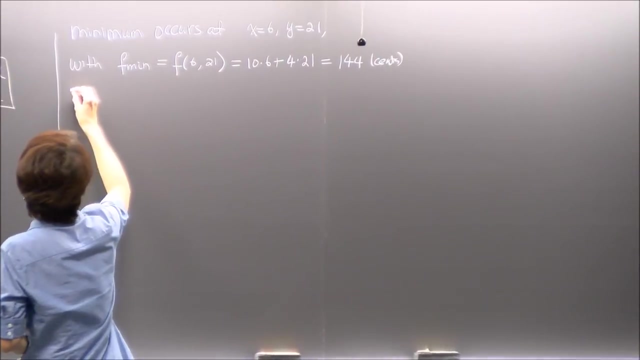 and this gives you some number. Okay, So this is a cost. so we know the unit is cents. Okay, so we solved this problem. So how do we translate it back? What do we tell? Okay, so we solved this problem. So how do we translate it back? What do we tell? 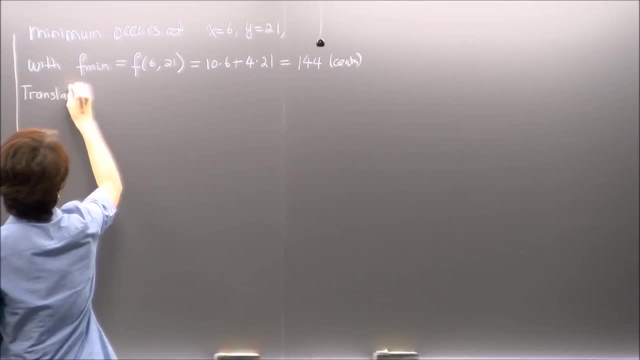 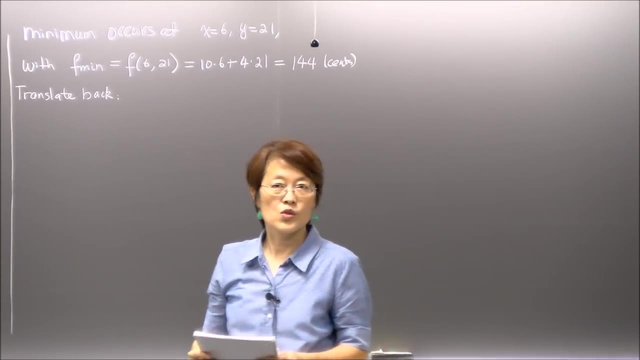 Okay, so we solve this problem. So how do we tell, Okay, so we solve this problem. So how do we tell, Okay, so we solve this problem? So how do we tell The farmer What he has to do to minimize his cost? 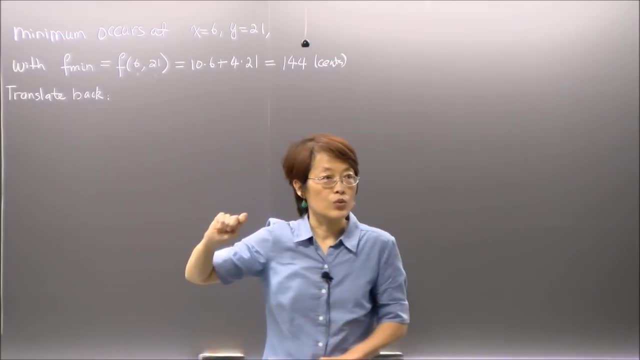 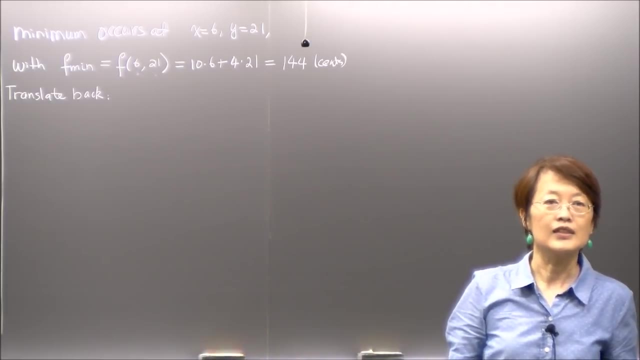 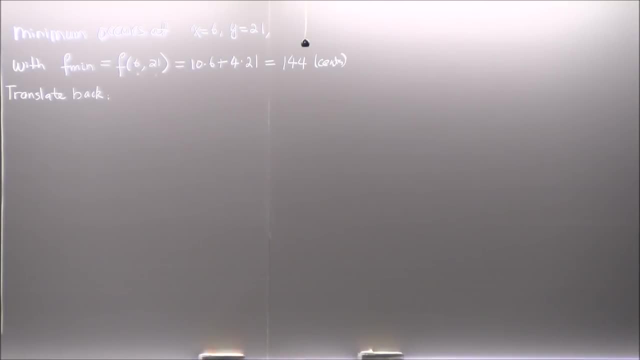 one unit of feed, two, and then we'll tell him that's minimizes your cost and the minimum cost will be 144 cents. is that right? okay? so let me write it. okay. so your best choice: use six. did I say pounds as unit? okay, whatever. six pound of feed, one and 21. 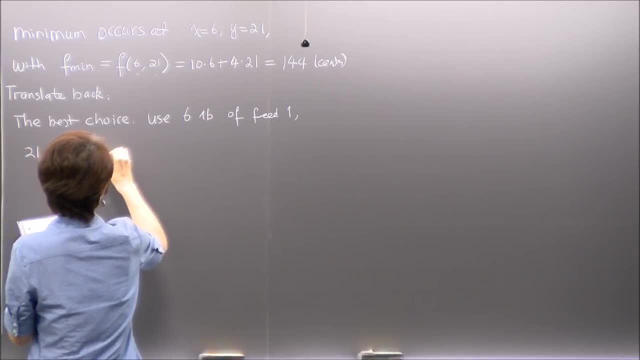 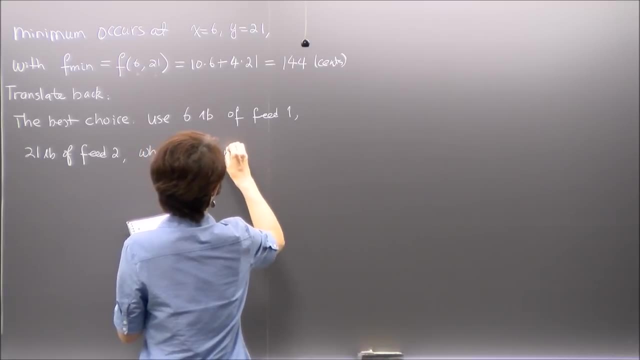 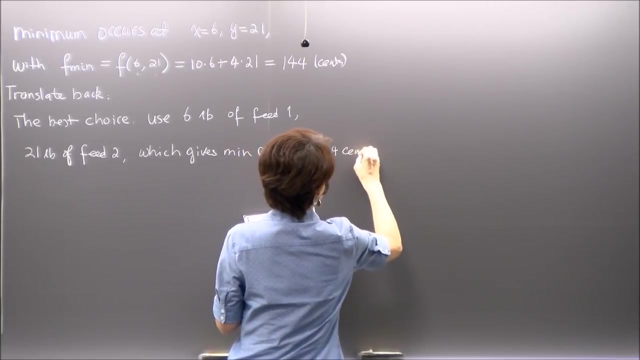 pound of feed, two, and which gives minimum cost of you, you, you, you, you, you, you thought, thought you, you, you. is that okay? any questions of how this is being worked out? can we handle similar problems? mm-hmm, okay, so if we look at this problem, look at the. 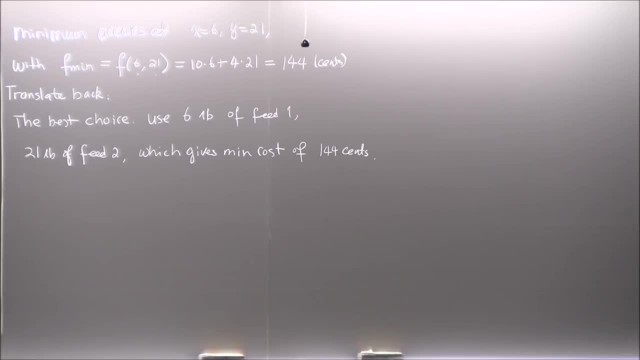 solutions we found and recall that last time, the conclusions or the observations we made for the previous example. so what were the observation we had there? we had that the constraints are linear, so we have straight lines as boundary, so the feasible region is a polygonal boundary shaped polygonal line shape, the boundary region. all those 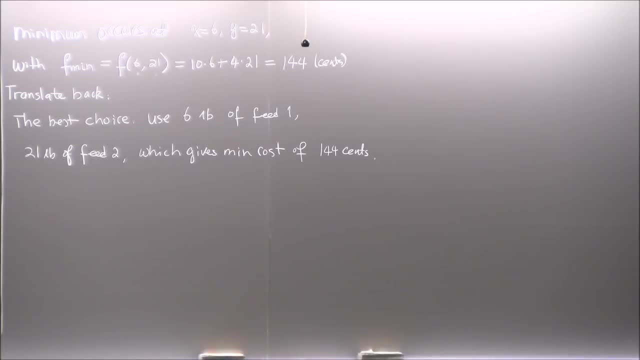 holds and the minimum is found at the corner as well. is that right? so all the observations there again is true here, okay, so let's put that as a remark. so all the observation from last examples: let's just say that they all hold. so probably that's. those are general properties. 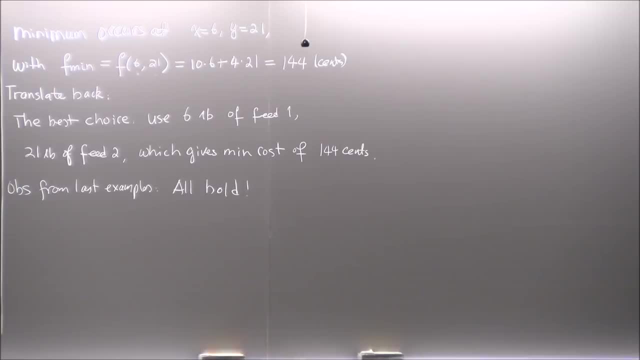 mm-hmm, in particular that the minimums occur at the corner. some corner is that right? so in particular I want to point out this one. so we know that minimum occur at a corner. now we are not proving it, so let's say, assume this is correct. 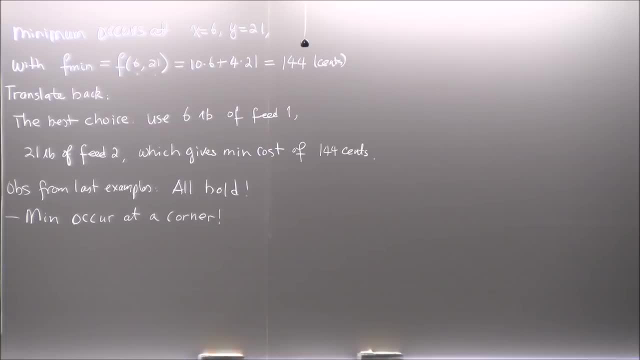 from two observations. later on we'll prove this. it's all right. so let's say that the minimums occur at a corner. so let's say almost true. so, assuming that is correct, do you get ideas, some idea that um, give you an algorithm of finding the minimum? hmm, can you think about it? so this: 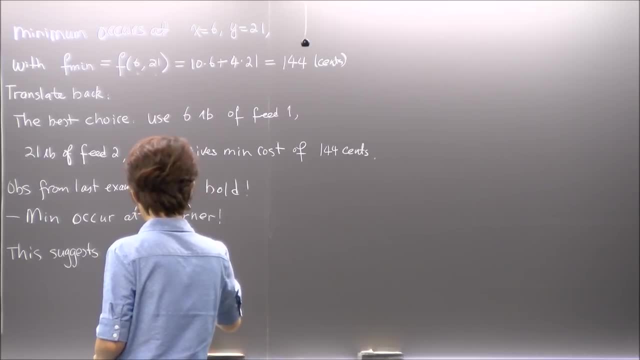 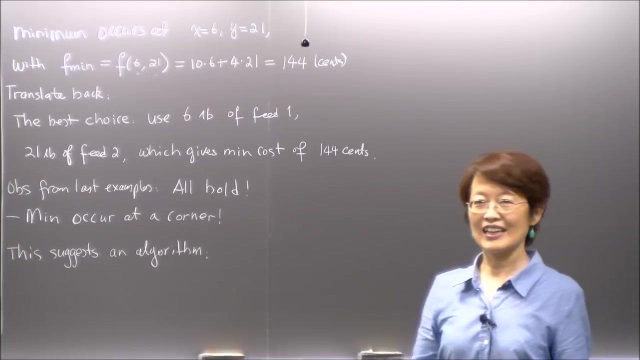 suggests an algorithm. if you know the minimum is always going works all right. so if I remember that here, but let me do this at this camera, I just something here if you need that, if you're looking for at that, aside from thecznieil, with a regression fx we have, because of independent properties of both, the вниз in to the area we see here. 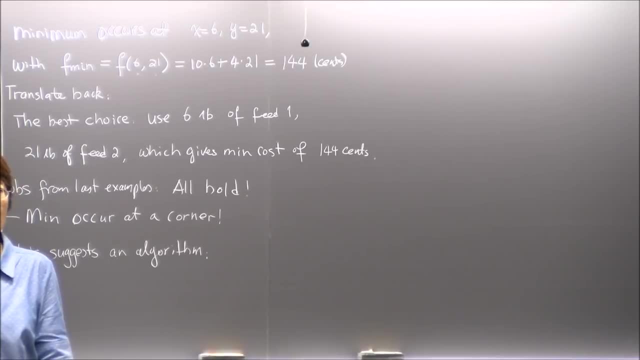 and find the minimum there just at a few points. Does that make sense? So let's try that out. Okay, so this suggests that we only need to check the corners. So you still have to find the feasible region and find the corners of your feasible region. 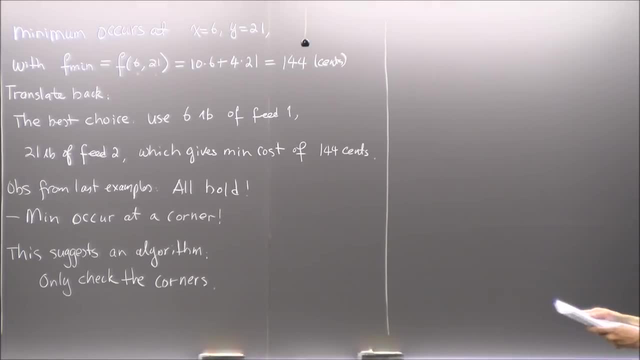 and then you can just evaluate the cost function at those corners. So let's set that up. We can do it in a nice little table. Okay, so the corner points. We're going to list the points. We have four points right. 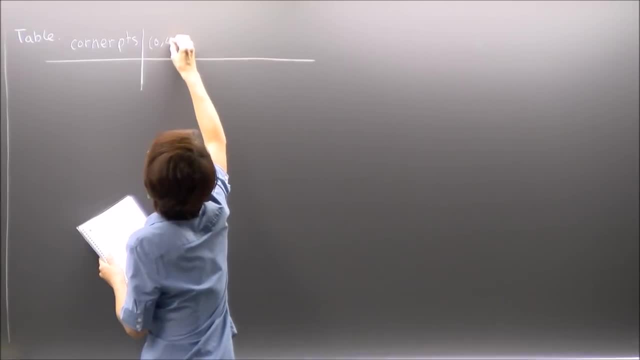 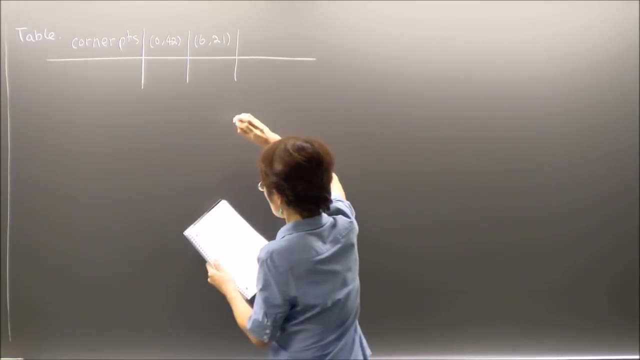 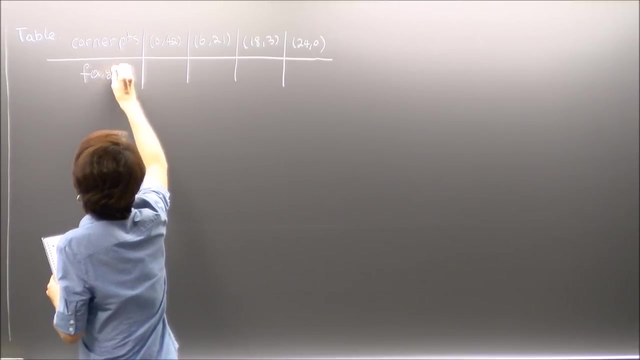 So 0,, 42,, 6,, 21, and 0,, 18,, 3,, 24,, 0.. Okay, and then I will compute the function f, the cost function, at those four corners. So you're just putting those x and y value and evaluate. 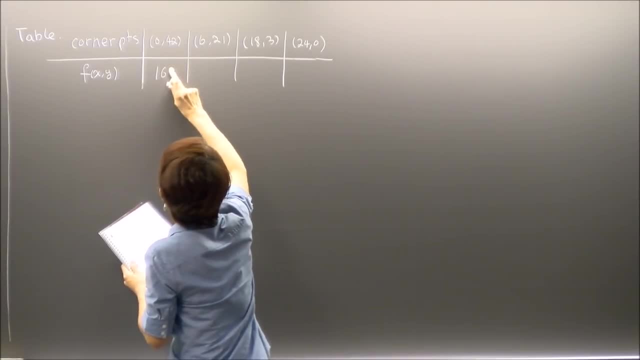 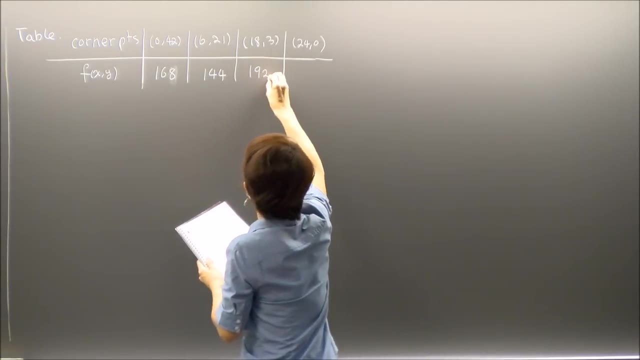 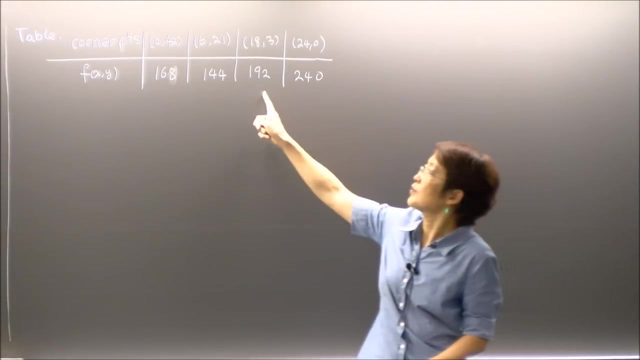 It's easily verified: 168.. Let me write 8, nicely, 144.. 192,, 240.. So only those four numbers, the function value at those four corners, are meaningful for me. I just need to find which one has the smallest value. 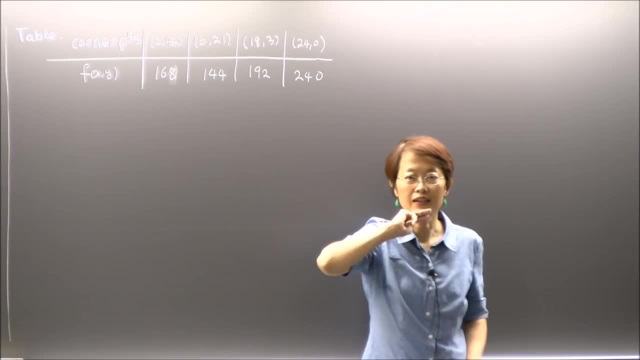 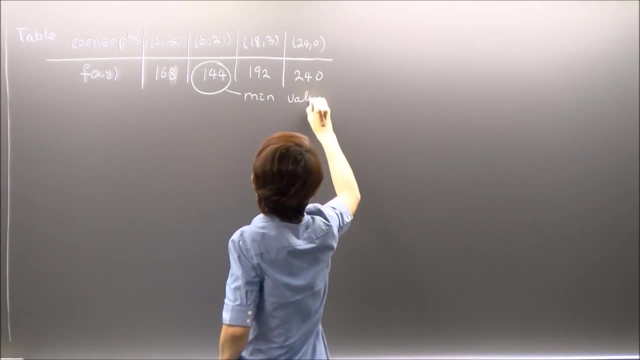 and that will be the minimum. Is that clear? So we found out that this guy is the minimum value. So you say the minimum value is that occurred at that corner, Is that okay? Okay, Well, this algorithm one can use, provided that observation is a general property. 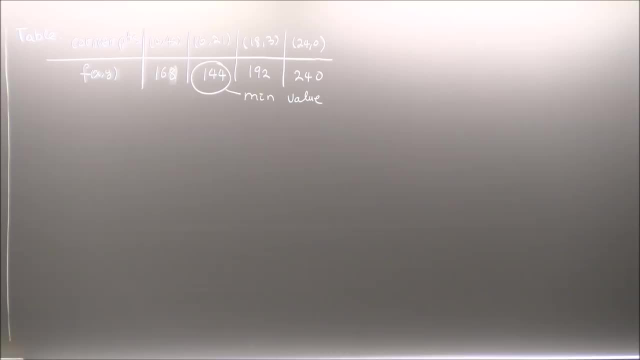 Right, We haven't proved that yet. Well, it almost is true. So, okay, let's look at some situations that it actually is not exactly true, Okay. So okay, let's talk about it first as a flexibility of the method of this algorithm. 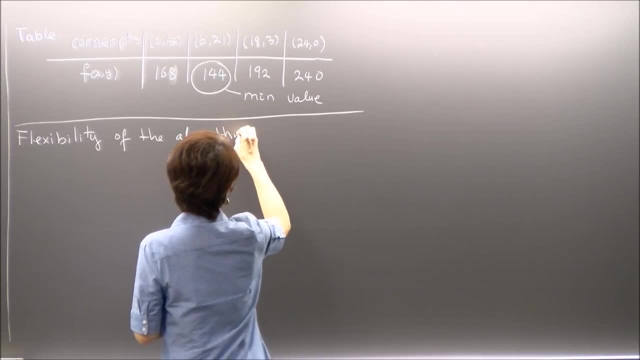 So assume now something has changed in the situation. For some reason the market has changed and the price for the two feeds- feed 1 and feed 2, are slightly modified. Okay, For some reason market changed, And how would you adapt? 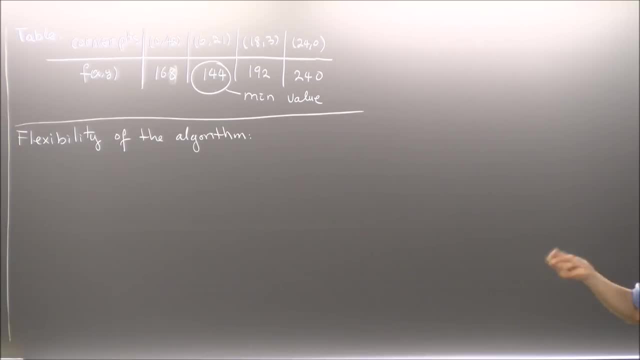 You might have a different strategy If feed 1 becomes much more expensive than feed 2, you might not want to buy too much of feed 1.. Is that right? Okay? So let's say, if this is that is the case. so if now. 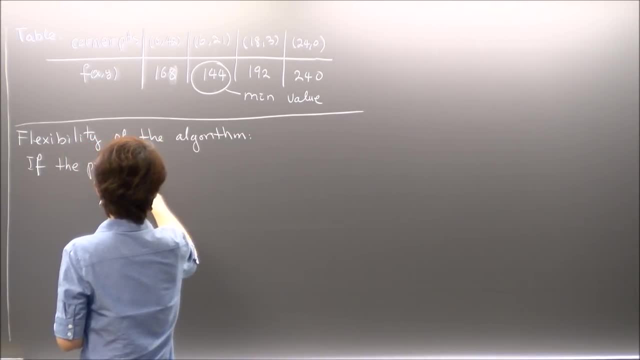 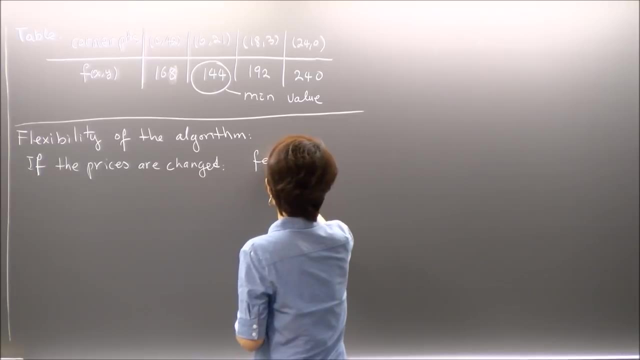 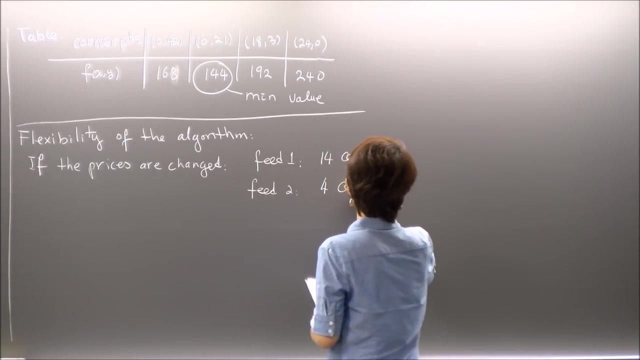 the price. the prices are changed to the following: okay, so feed one, let's say i change it to fourteen cents per pound, and feed two, i change it to four cents per pound. how should the farmer adapt to this change? how would the problem be different? so do i need to change my constraints? 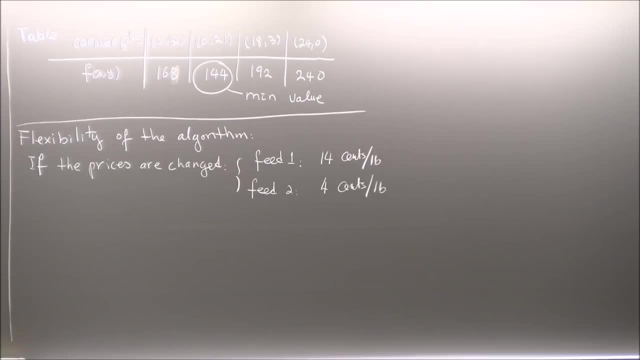 there's no change in the constraints. is that right? the constraints are the same. what shall be changed in this table are these two numbers, which means my cost function will be different. is that right? so i'll have a new cost function. let's write it out new. 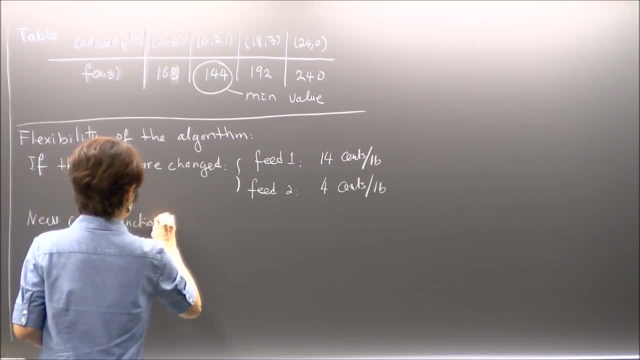 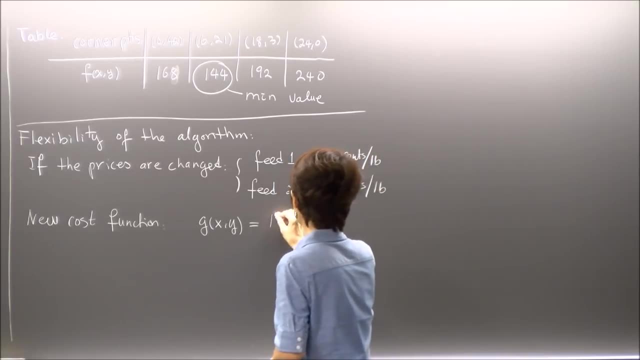 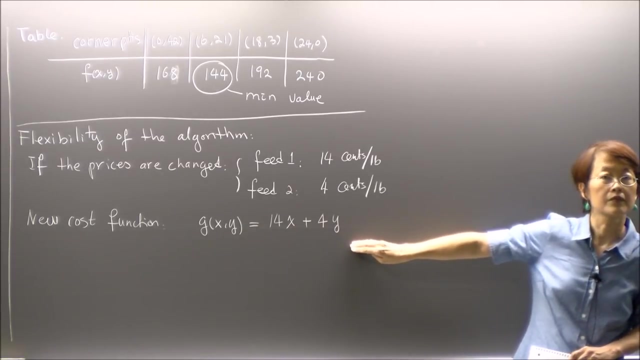 cost function. okay, let's call it g depends on x and y, so it's slightly different. so i'll have fourteen for feed a feed one and four cents for feed two. so is it clear how i get this function? fourteen is the price for feed one. four is the price for feed two. 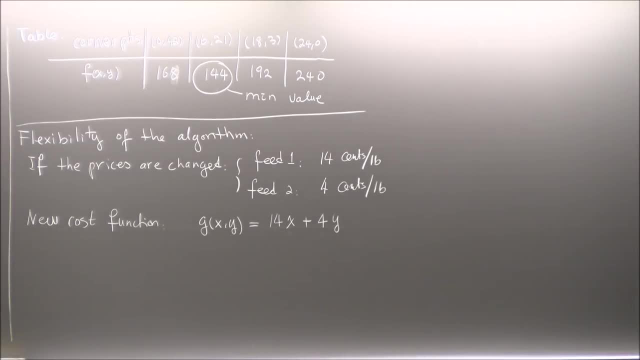 right. so let's use our new algorithm. let's say i'm going to check those four corner points, since i did all the work, and find out the feasible region, so let's set in this table and look at it. so on this. so the table will be the function for g. 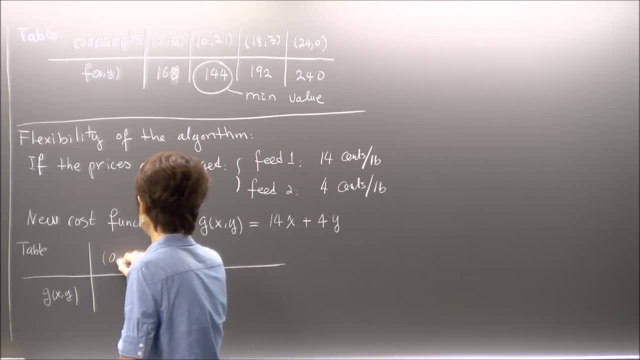 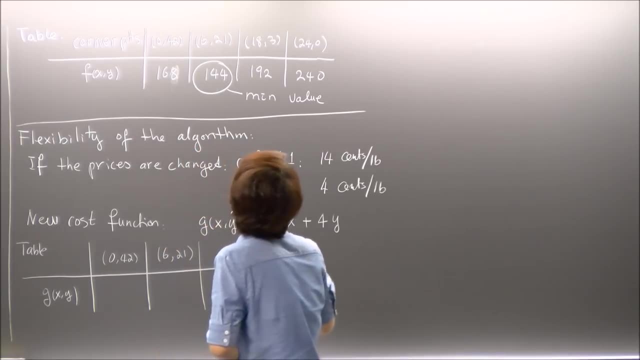 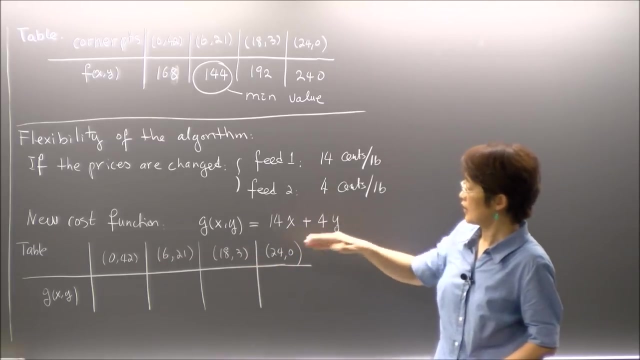 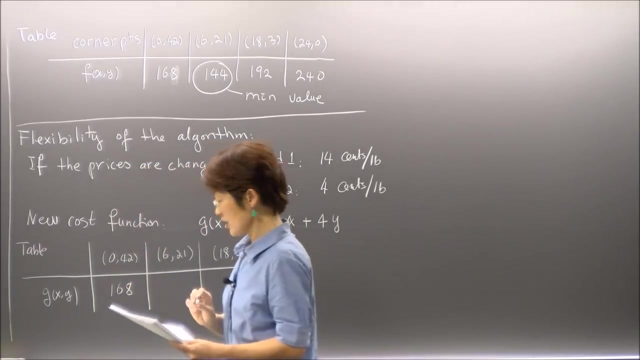 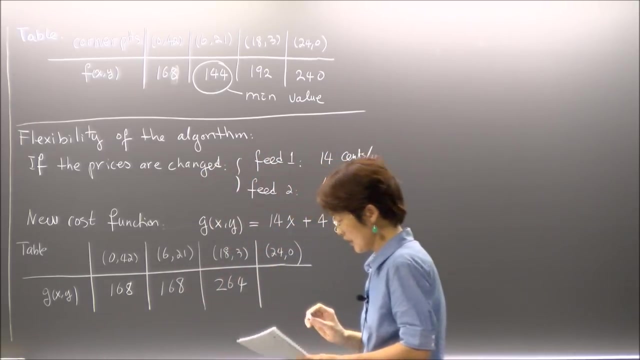 g of x and y and i want to evaluate it at the four, four corners. so if more, let me go here. okay, so you just plug in the xy value here and add up and evaluate. so if I do that, I have the following: I get one six eight, one six eight. oops, two, six, four and three. 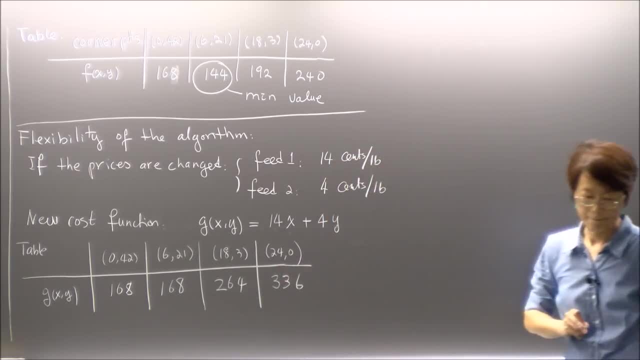 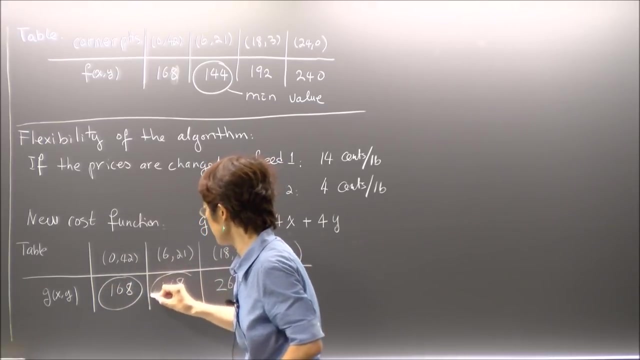 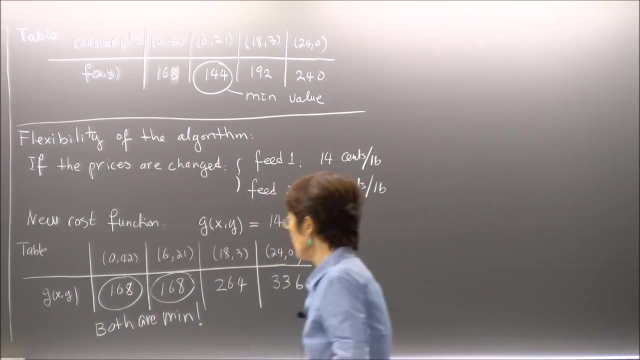 three, six. something a little bit strange happened here. where do I find the minimum here, these two values? they are the same and they are the smallest here. is that right? both are minimums, so both are minimums. okay, so can you try to think a bit and 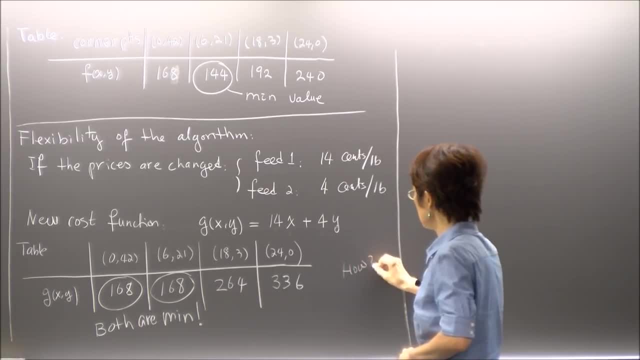 say: how is that possible and why is this happening? what does it mean? that meaning that I find the minimum at two points, and what's causing it? let's go back to the picture. so where are these two points? I found out that one is this point. it's a. 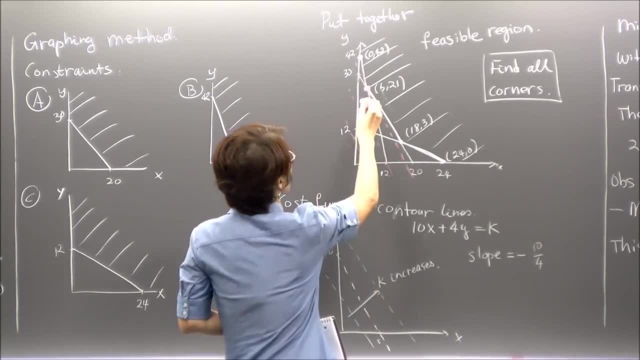 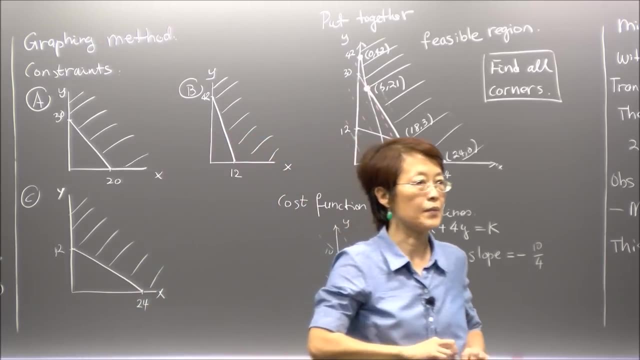 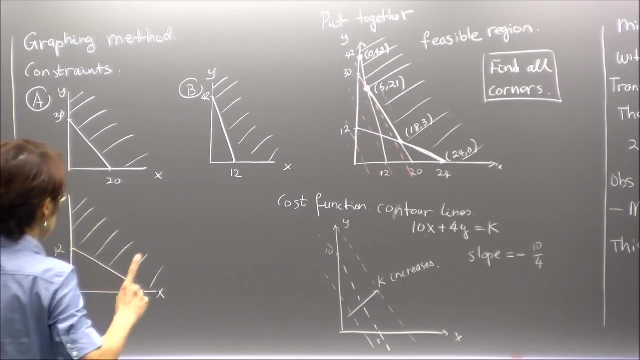 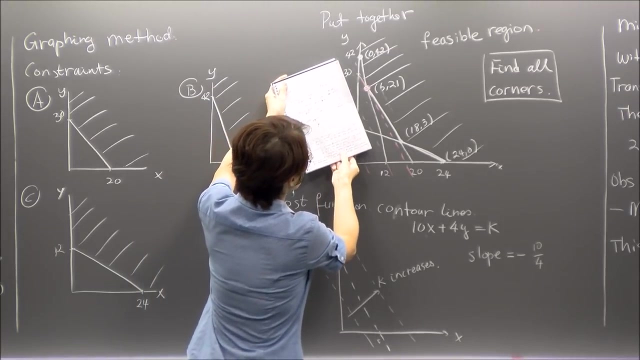 corner. and the second one is this point: they both give me the minimum value. so why is this happening? you want to suggest yes. do we see that? thinking of the first method that we suggested, using the contour line, copy the slope of the contour line and approach my feasible region with that slope, and then where? 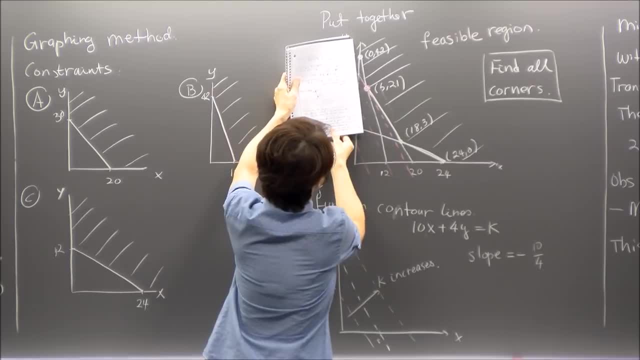 will I touch the region first. it's parallel to this, so I touch now, and then I touch the slope of the contour line, and then where will I touch the region first, it's parallel to this, so I touch now, not at a point, but at an edge. 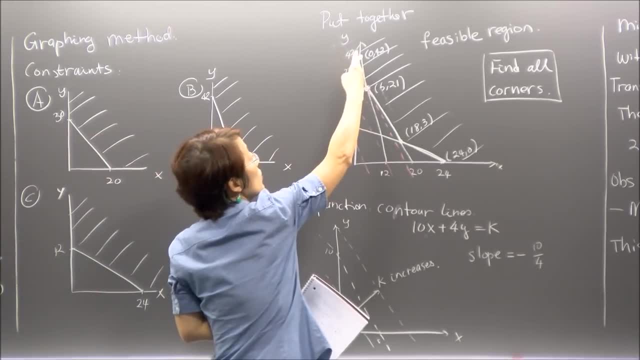 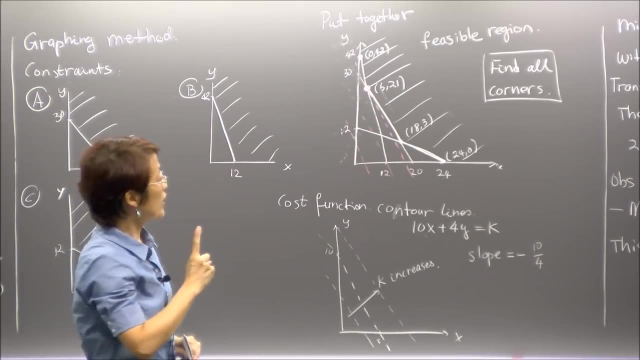 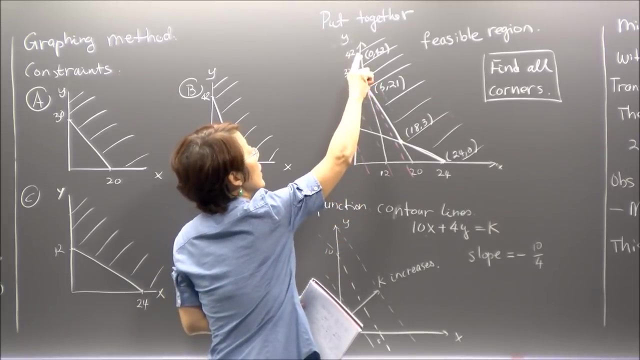 Do we see that? And along this edge, because it's a contour line, the function takes the same value. So not only did we understand now why I have minimum value at two corners, we also find out that along this edge, actually every point. 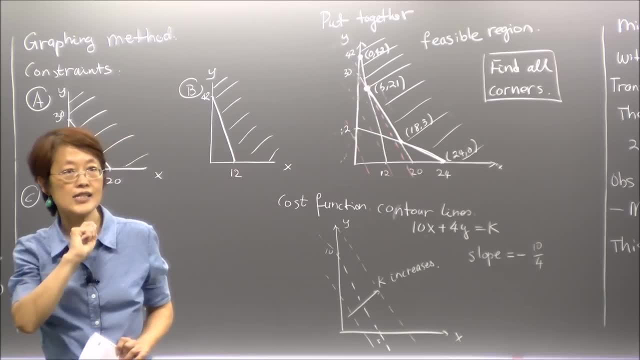 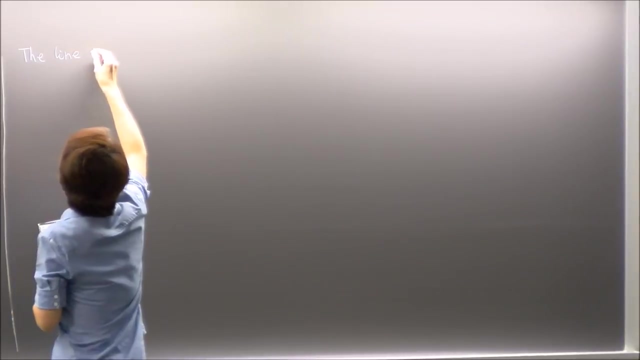 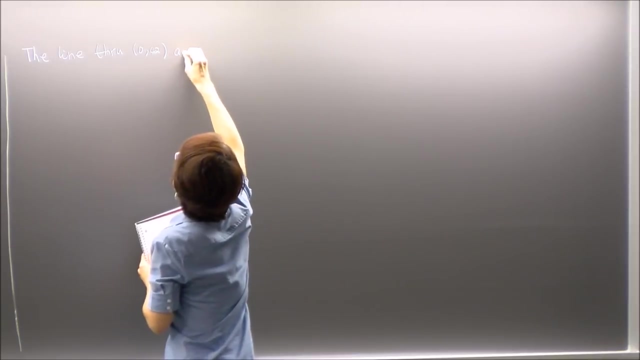 you have the minimum value. It's attained on the line segment on the boundary. Is that clear? So that's the new phenomenon, So let's put this down. So why? So I find out the line through those two points: 0,, 42,. 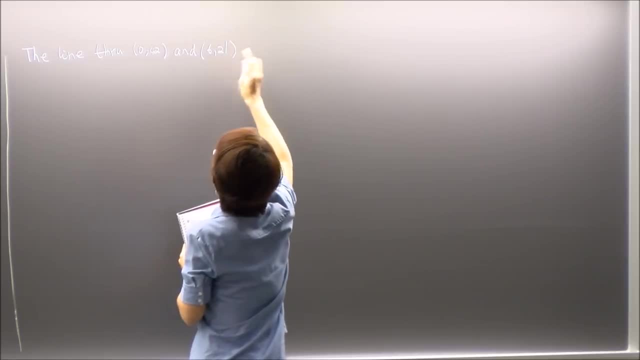 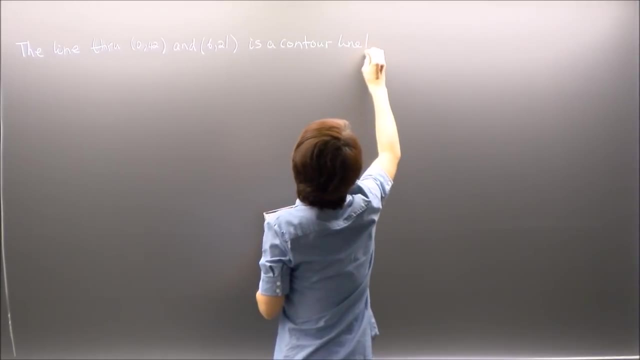 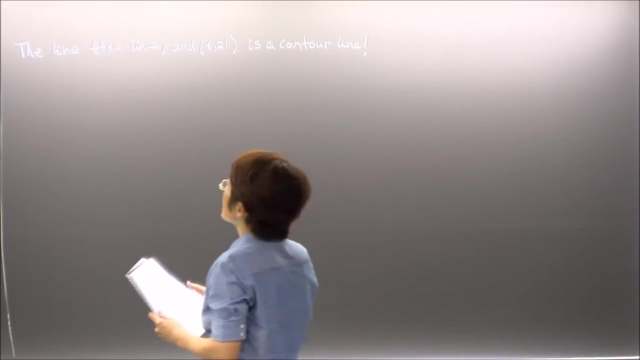 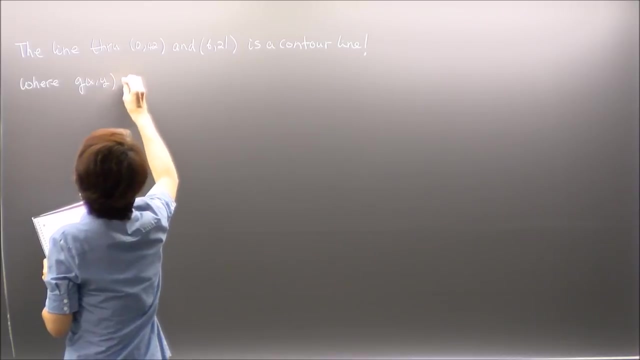 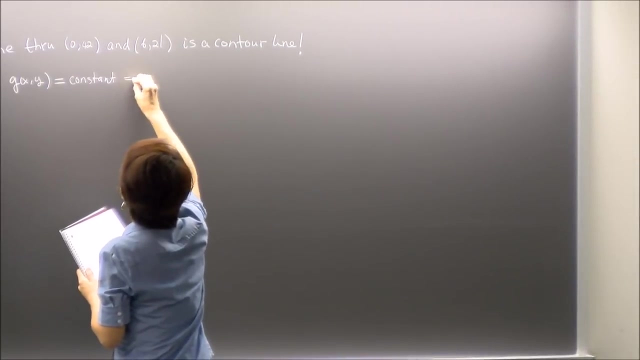 and 6, 21.. That itself is a Contour line, Is that right, OK? And then you can also conclude that the function g of x- y actually is constant along that line segment, So in this case actually attains its minimum value. 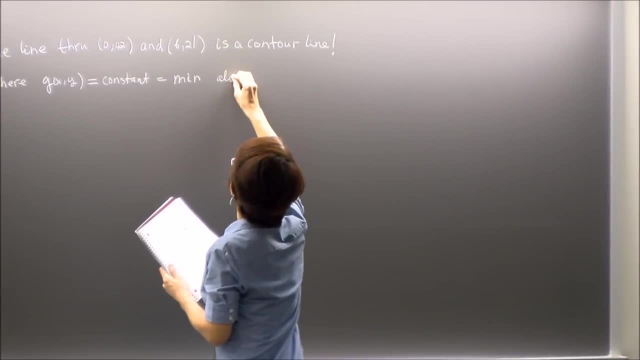 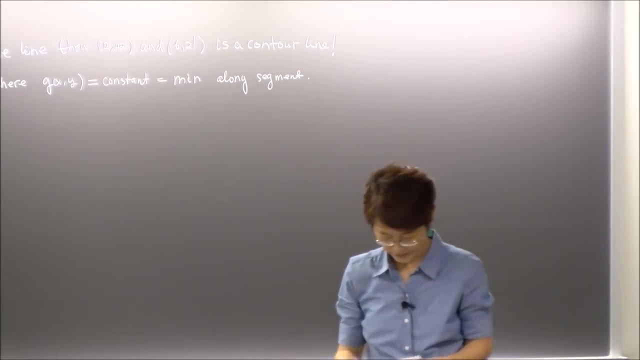 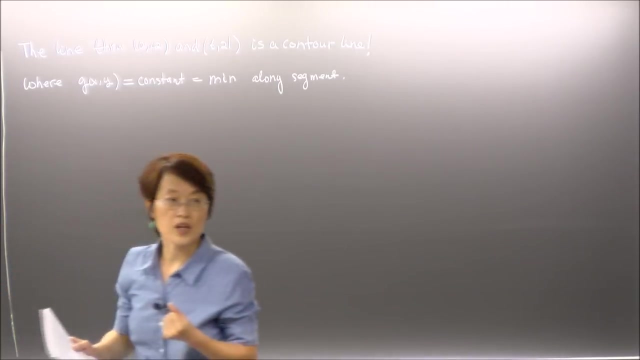 for this problem. Is that right? Yes, OK, So we see that the minimum value is attained, actually at infinitely many points. Not only two, but many, many, many of them Right. So let's list our new observations. 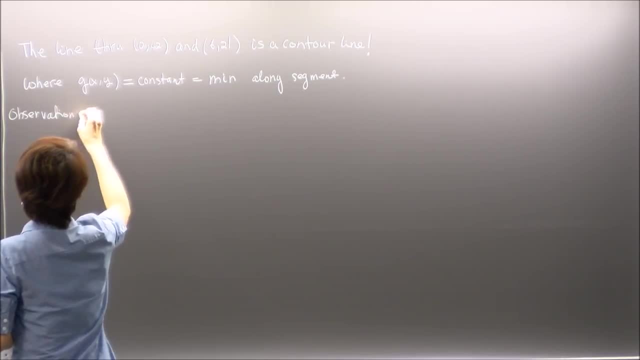 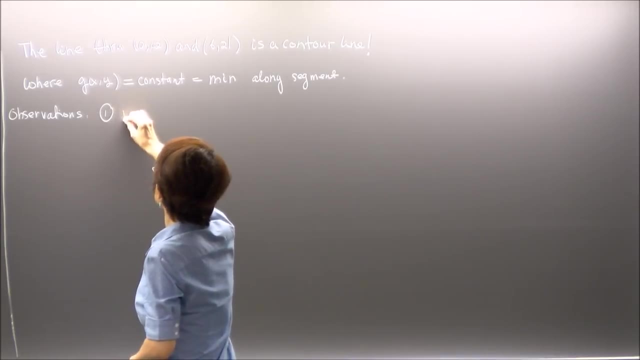 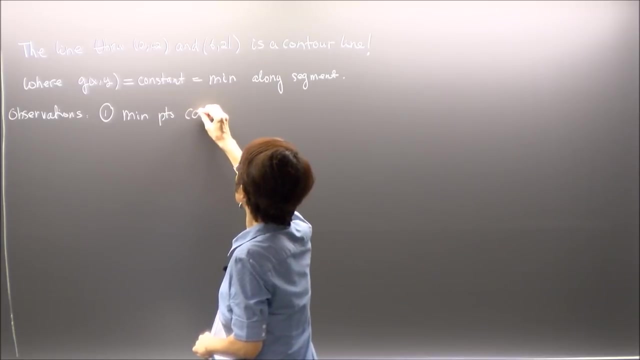 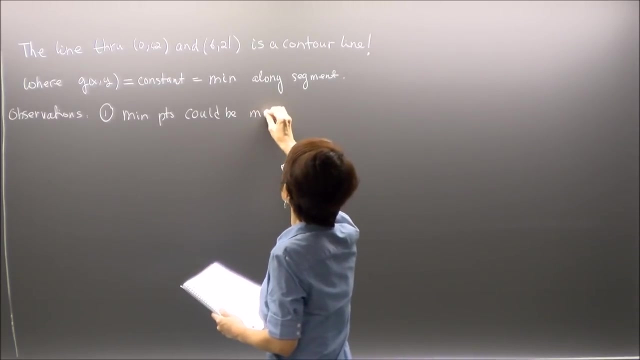 So it's kind of expanded our understanding of the problem a little bit now: Mm-hmm, Mm-hmm. So we observe that now minimum points, the points that minimize your problem, could be minimum. OK, So minimum could be many. 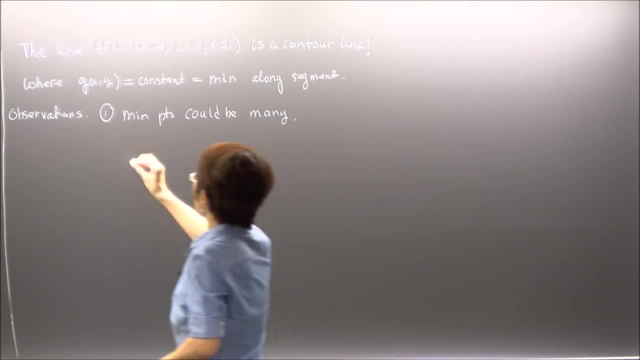 Mm-hmm, That's one thing. So, even though the points you attain, the minimum can be many, many, not unique, But still the minimum value is unique. Is that obvious? That shall be obvious, right, If you find two values, they are different. 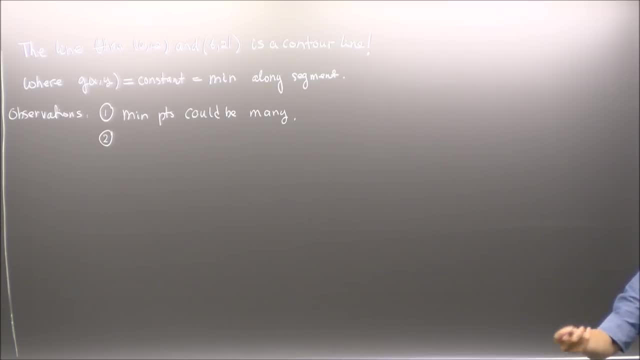 and you say they are the minimum value, of course the smaller one shall be the real minimum value. Is that right? So that's kind of an obvious observation. So I would say, minimum points are not unique, but the minimum value is always unique. 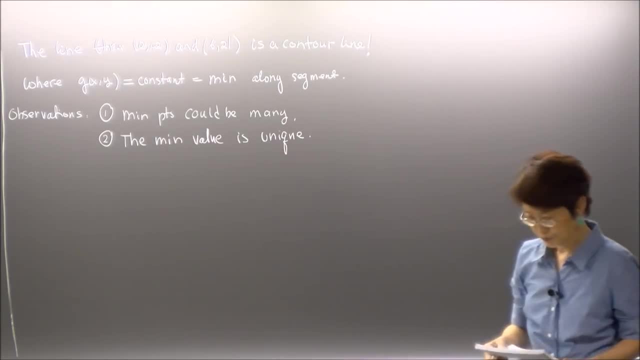 You cannot have more than one, OK, OK. So let's make a third observation. It's kind of important, So let me ask you if, let's say, I'm using this table method, I evaluate my gain and my cost function only. 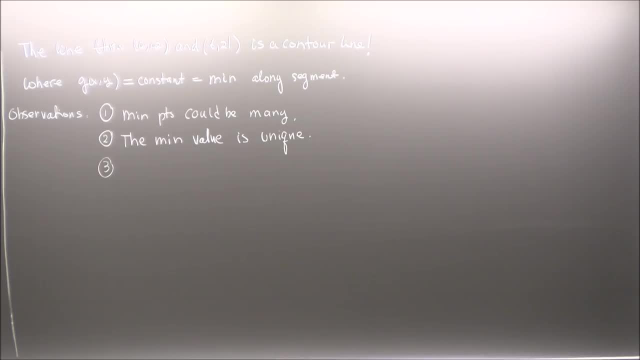 at those corners and I find out two of them are minimal. And then, let's say, I go back to the graph. Let me ask you this question: Would it be possible that those two points are the minimum value? And then, let's say, I go back to the graph. 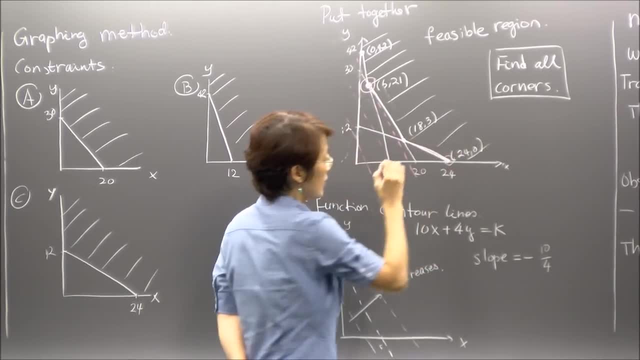 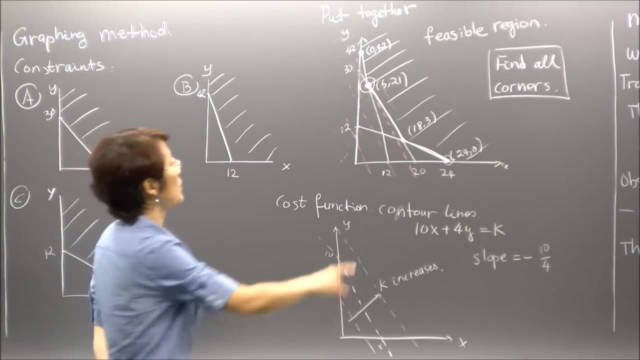 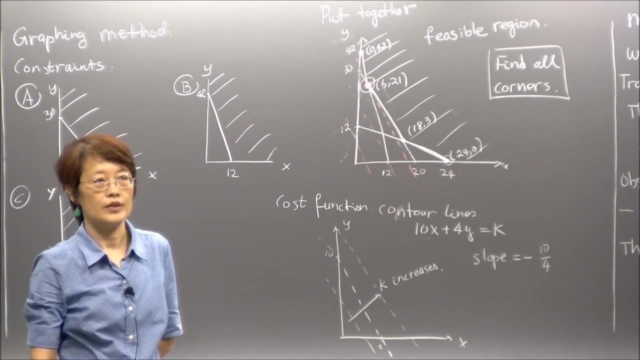 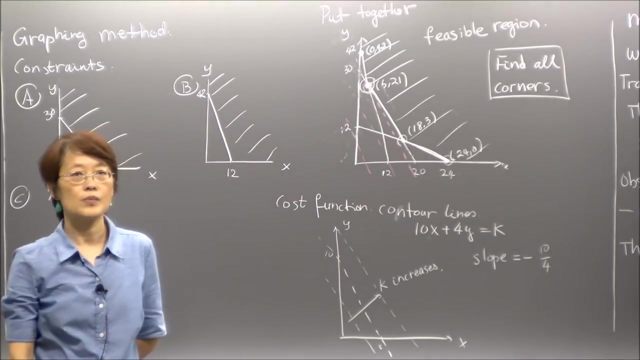 Let me ask you this question: Would it be possible that those two points I found out will be this one and that one? Could that be That your function attain its minimal at this point and that point? Would that be possible? Would it be possible that the two point will? 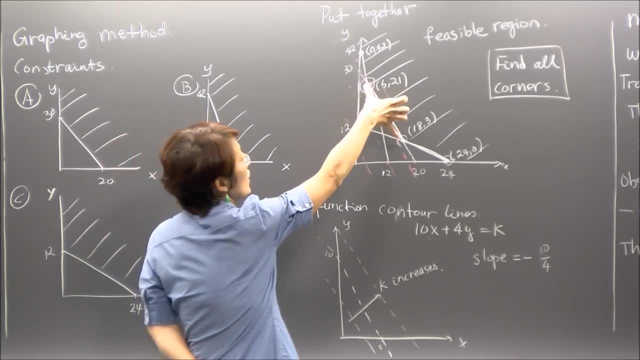 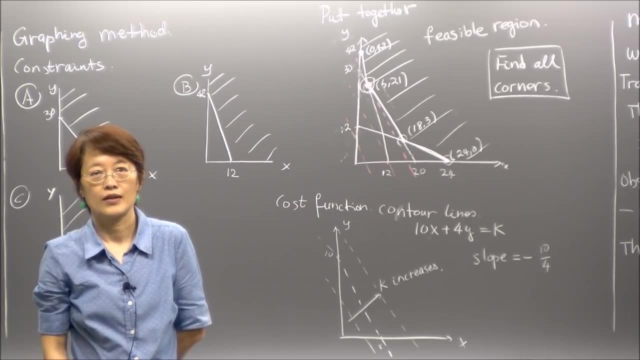 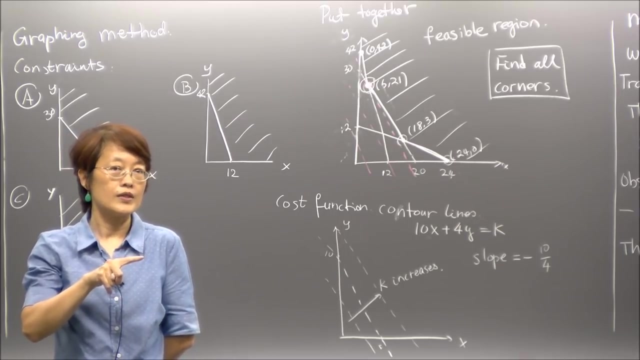 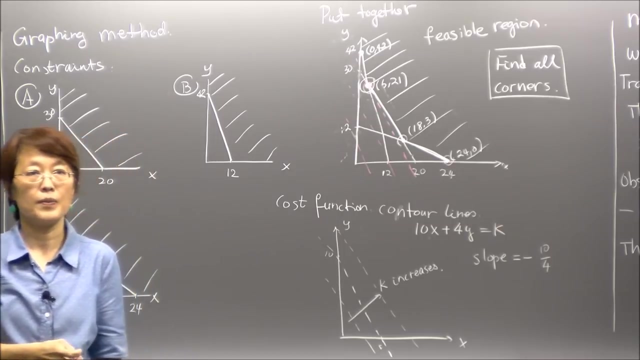 be this one and that one. Would that be possible, like this, and two points like that, if they shall serve as minimal? so if two points, two vertexes, are the minimum point, they have to be adjacent to each other. is that right along the boundary right? okay, so that is another. 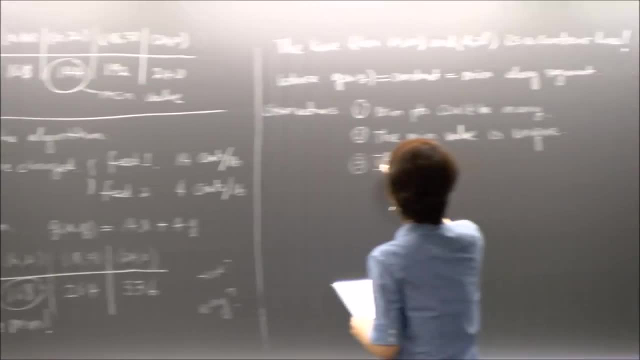 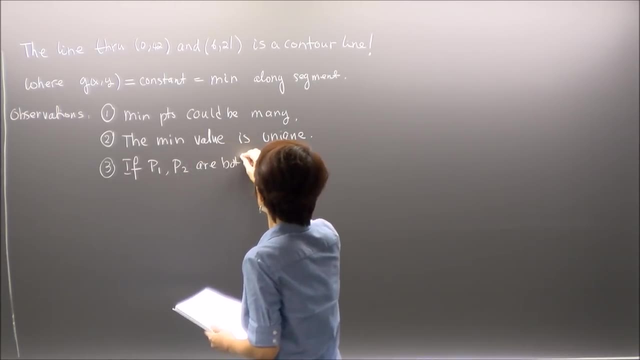 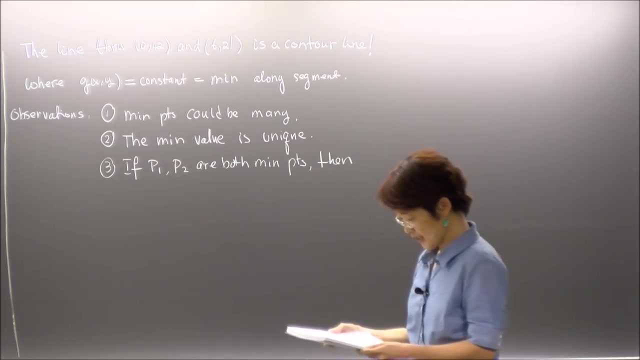 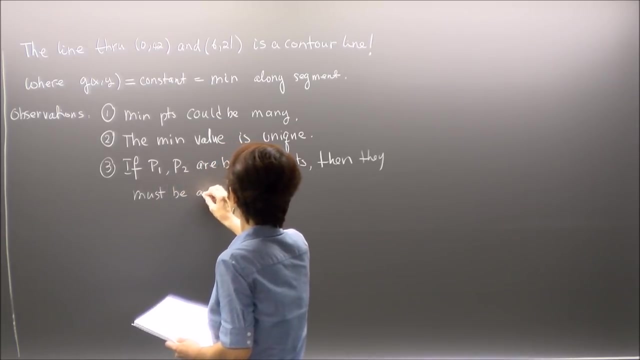 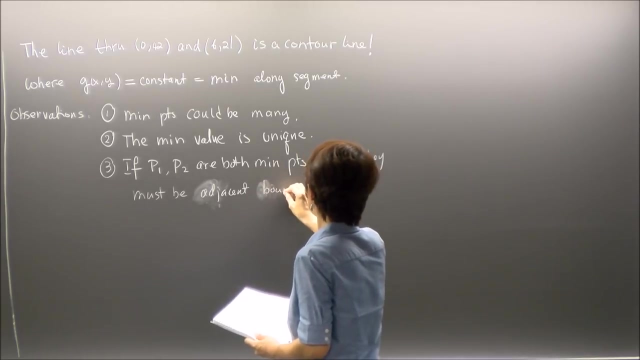 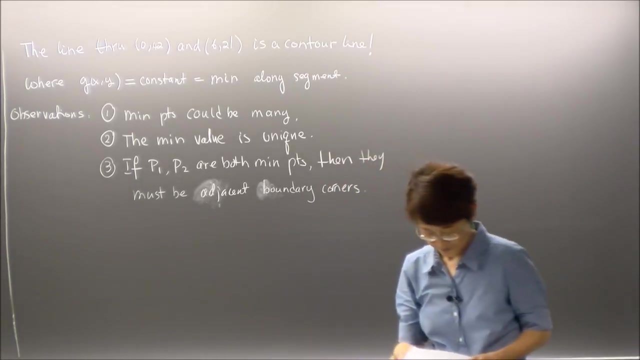 observation. so let's put it up. so if P 1, P 2- okay, are both minimum points, then what can we say? they must be AJ. Oh, okay, I cannot spell. how do you spell adjacent a, B, adjacent, is that right? adjacent boundary corners, vertexes, okay. 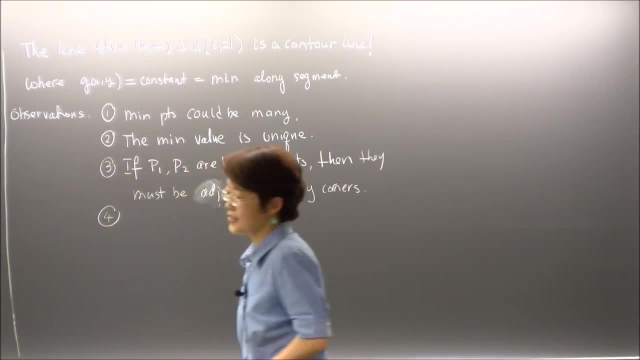 okay, and then okay. so this number four is not really new. so we know the graphing method is not really new, and so we know that the graphing method is not really new, and so we know that the graphing method only works for problem with two. 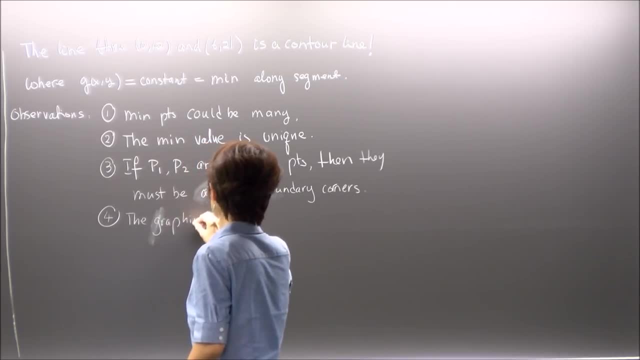 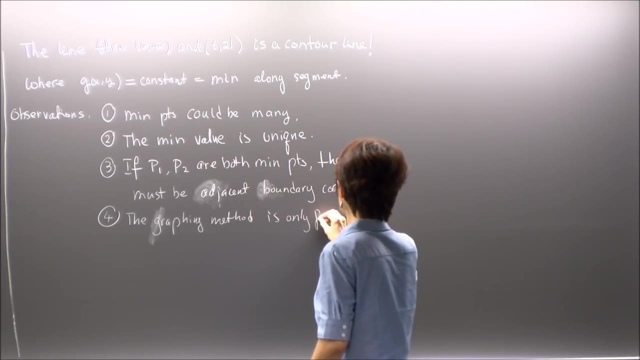 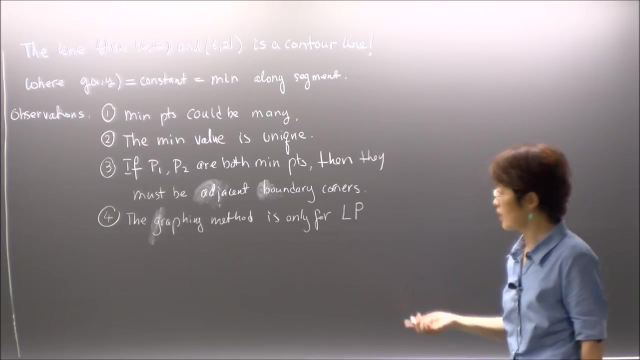 only works for problem with two variables. it's only toward um. okay, let me. it's only toward um- okay, let me. introduce this L P. I'll be using it over. introduce this L P. I'll be using it over and over. these are called shorthand for and over. these are called shorthand for linear programming. 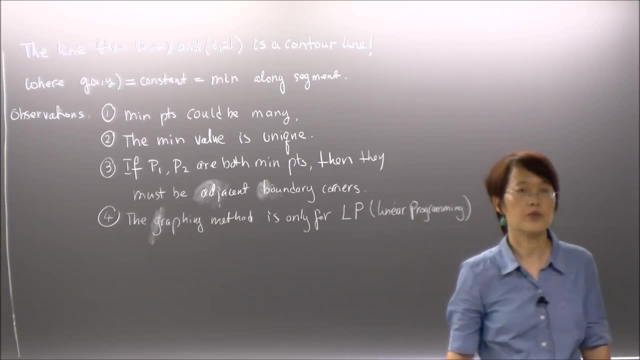 linear programming, because the whole course is about linear programming, so I'll just write LP from now on. it's for linear programming, it's okay, otherwise it's long. okay, it's for linear programming. problem with only two variables. well, that's obvious, because if it's more than two variables, I cannot visualize it and draw it on a black. 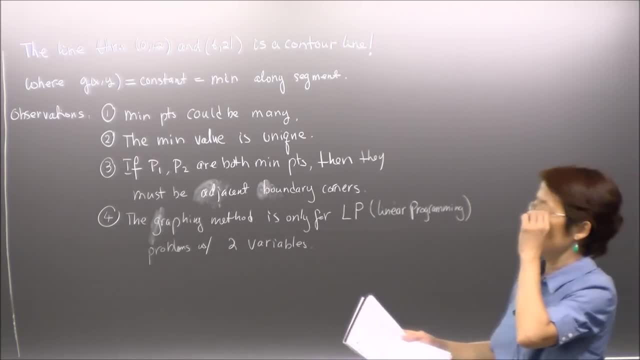 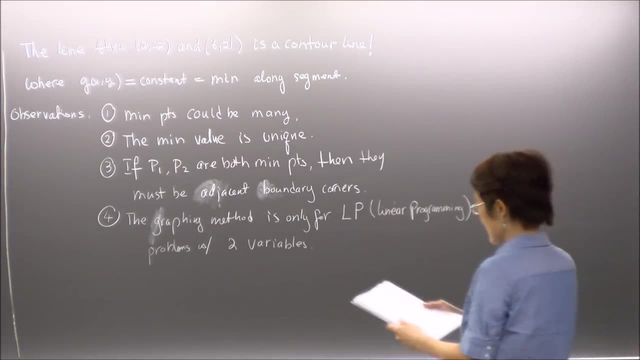 board. okay, even though I could visualize it as surfaces in the 3d, but that's much harder to to show you where they are. okay, okay, last one. so the two examples we have seen now are all minimizing and you can easily think that for a problem. 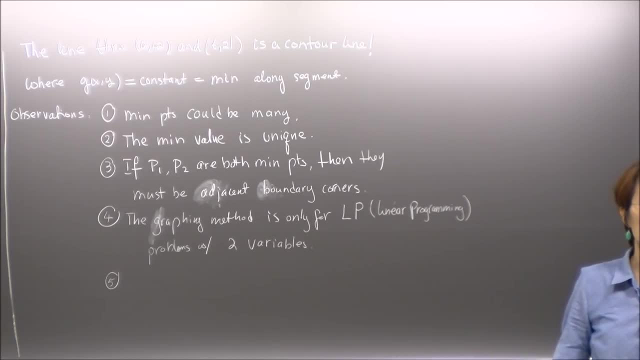 that I need to maximize something. the same approach can be used. is that right, it don't have to limit, so works. also. you for maximization, say, instead of a cost function I have a profit function, then I want to maximize it, right? okay, so these two examples we have had are nice examples where you could find 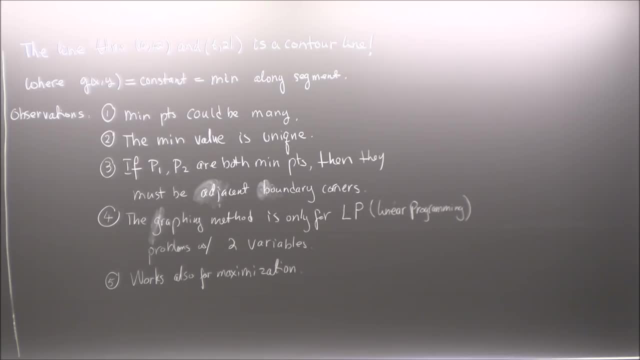 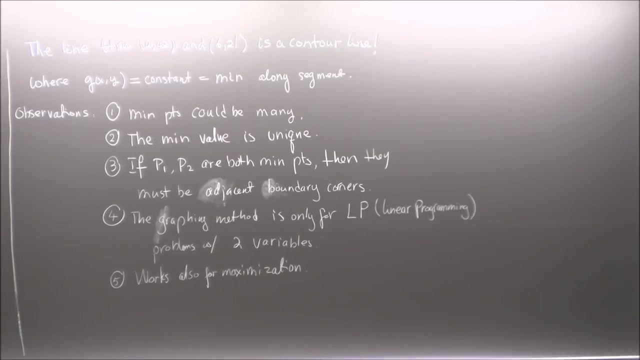 the solution, the optimal solution and the solution are finite and the cost is finite. but that doesn't have to be always the case, because not all problems are so well defined. some are not so well defined, so let's put that up. okay, so we're going to. 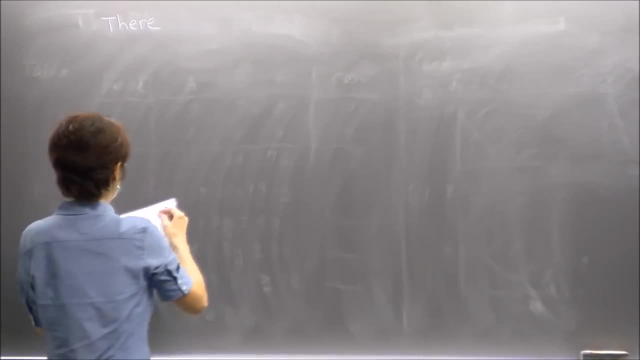 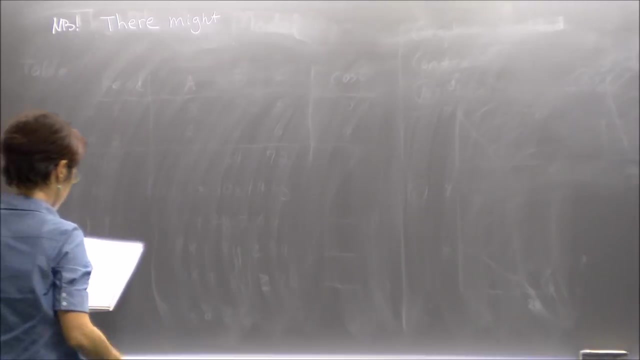 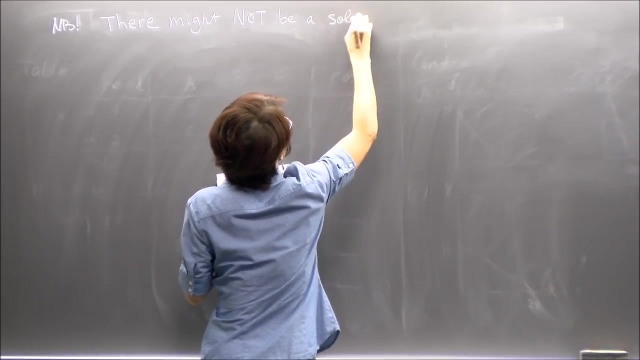 look at it in a kind of abstract setting, not with word problems. so I want to make a statement: okay, so there might not be a solution. It depends on the problem, okay, which you set up with. So let's put the statement up. 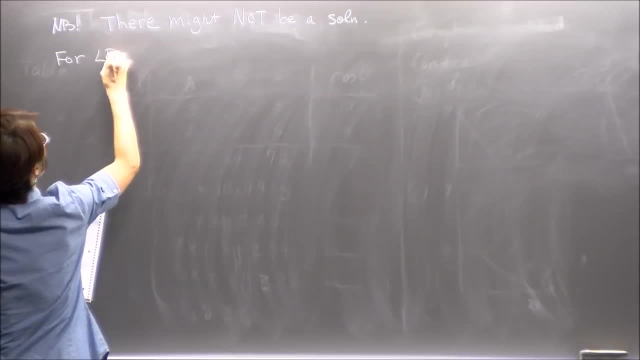 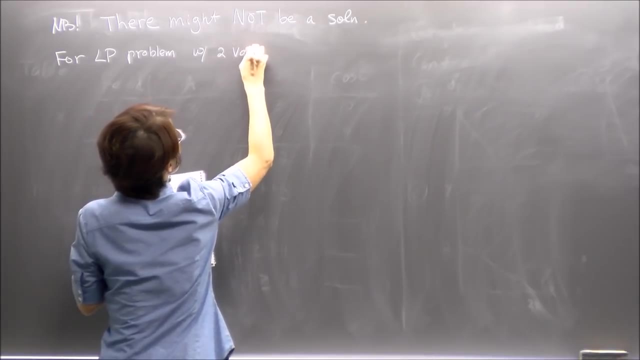 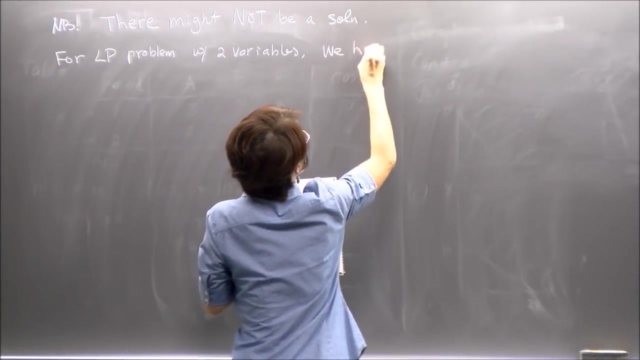 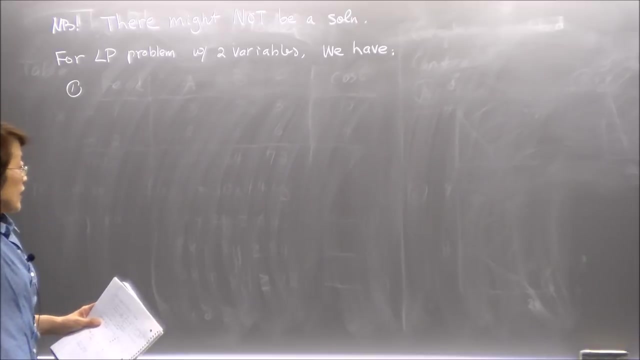 So for linear programming problem- right now I'm talking about it with only two variables- Okay, we actually have the following. we have four cases, so I'm going to list. So the first case, that's the nice one, the first example we have. 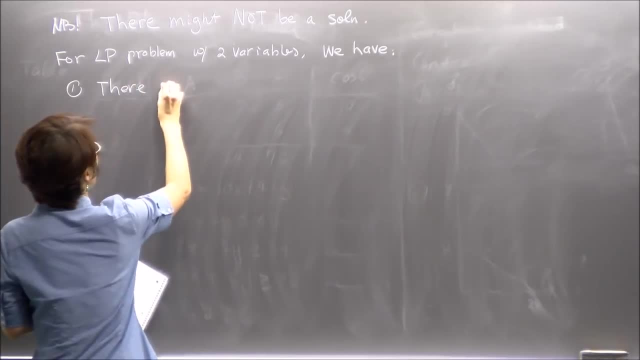 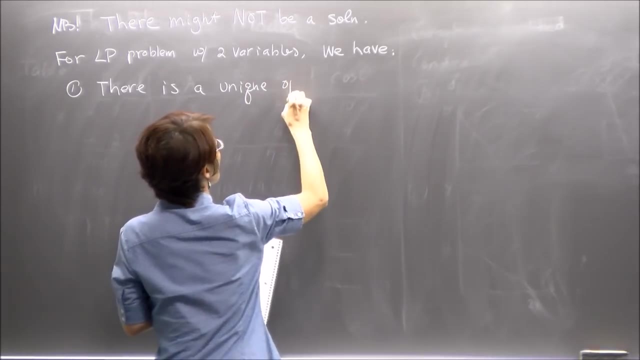 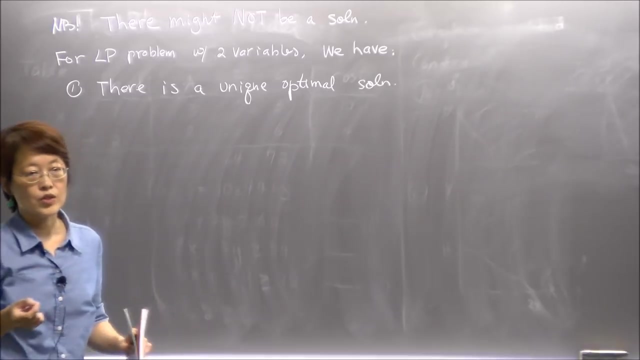 So this is the case, that there is a unique- okay- optimal Solution, meaning a unique point where the optimal value is attained. okay, like the first example. Okay, and then we know that the point where the optimal is attained should always be a vertex point on the boundary right. 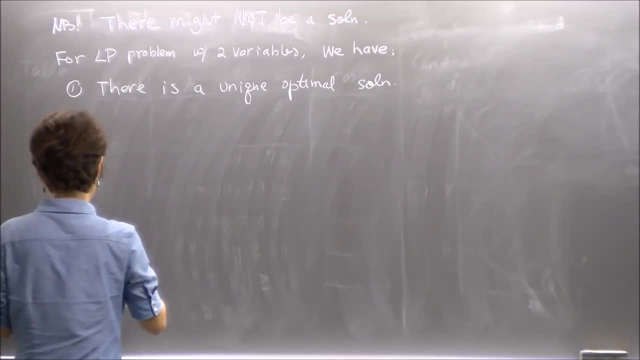 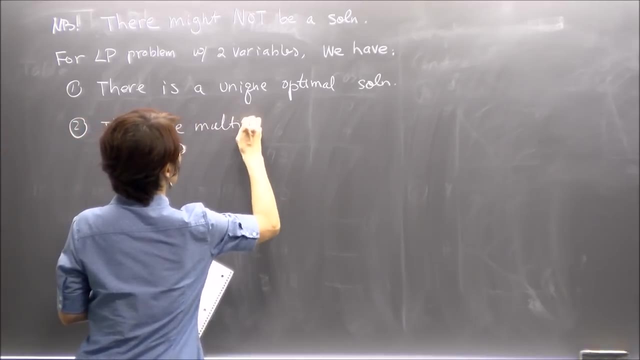 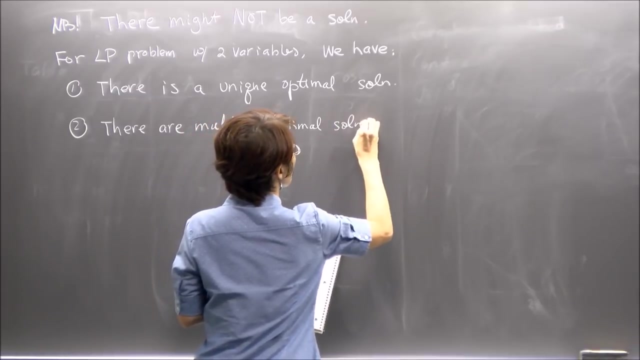 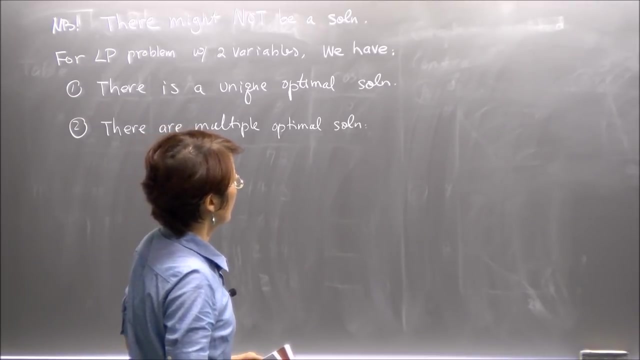 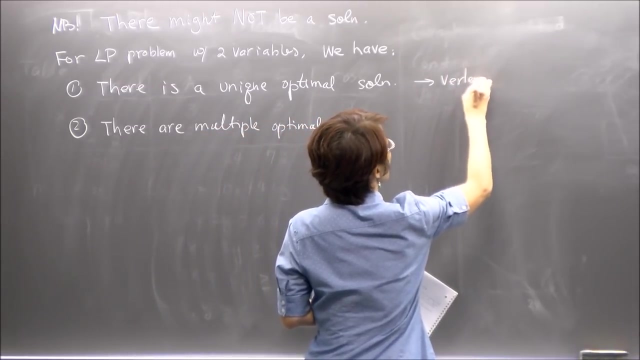 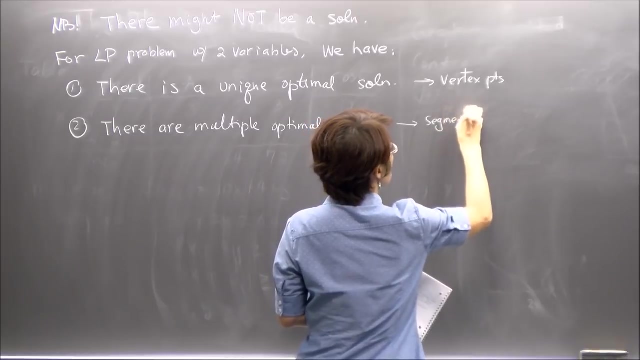 Okay, that's clear. And then, second, there are multiple Optimal solutions. okay, Okay, I could have two vertex as this example. So this, okay, so this usually give you one particular vertex point. okay, and this usually give you a segment, a line segment on the boundary. 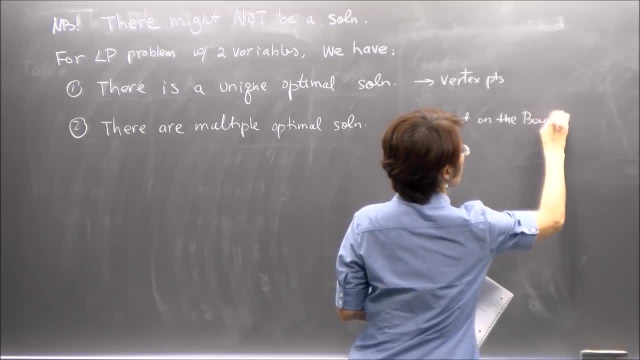 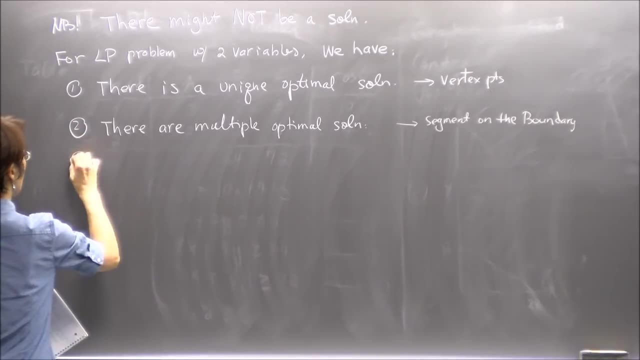 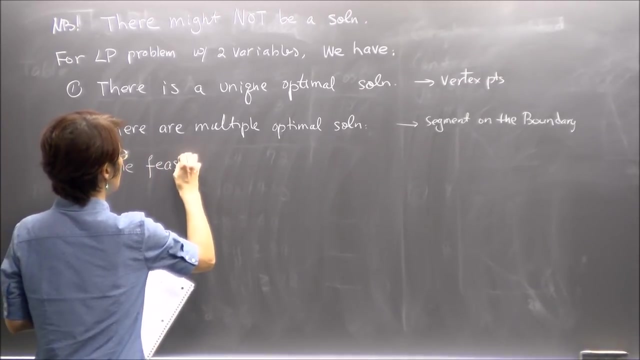 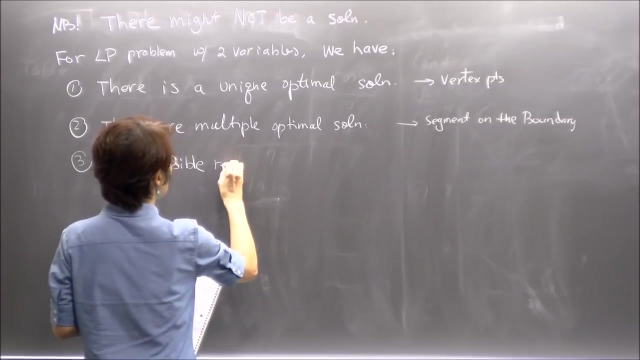 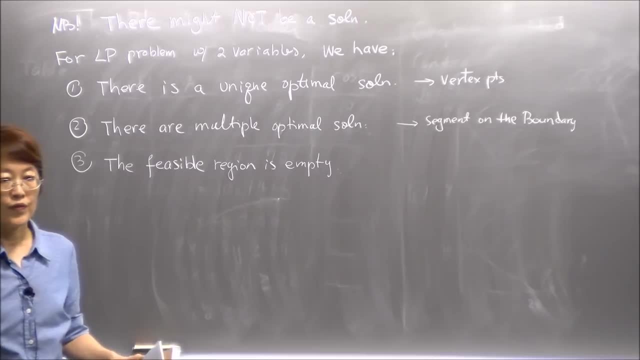 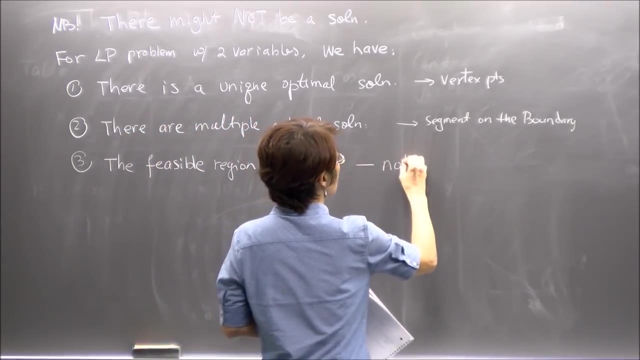 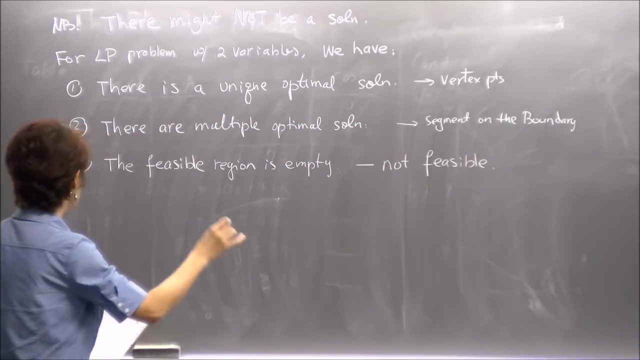 There are no points, x, y, value that will make all the constraints be satisfied. okay, So in this case we call the problem not feasible at all And of course, there will be no solution. okay, We haven't seen examples like that. 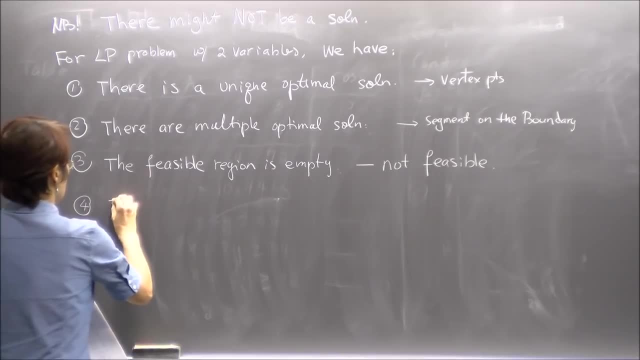 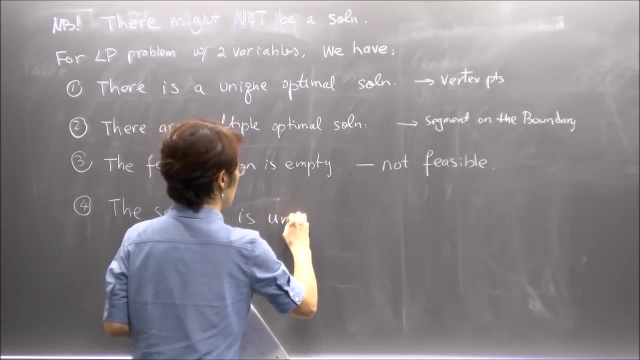 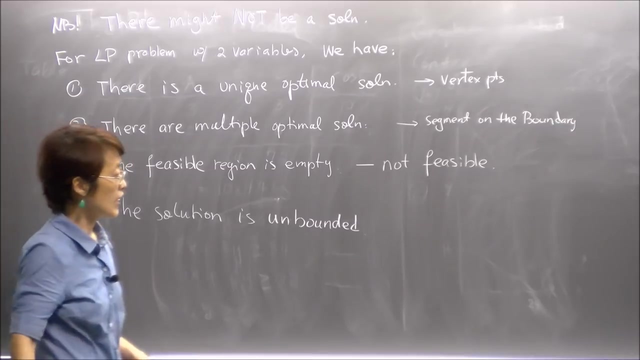 I will give one And then the full one is okay, there is a feasible region, none empty. but the solution I found is unbounded. I do not have a finite value as my optimal value in the problem. Okay, 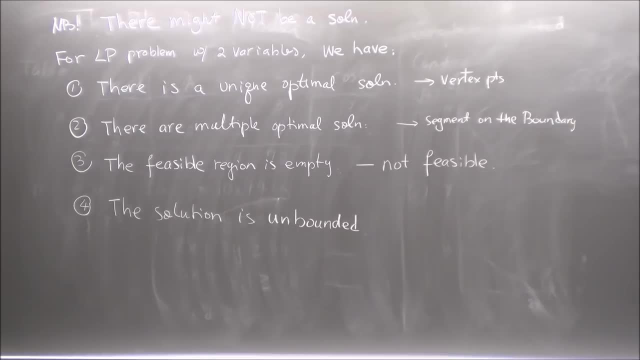 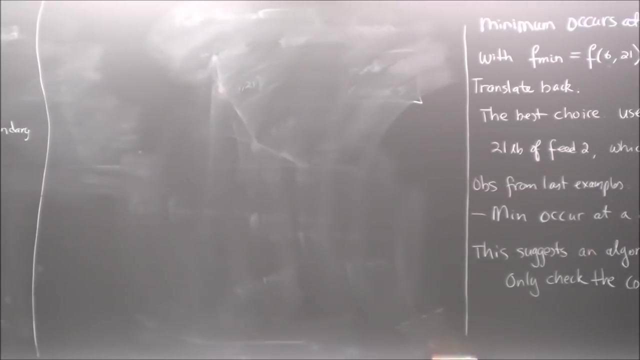 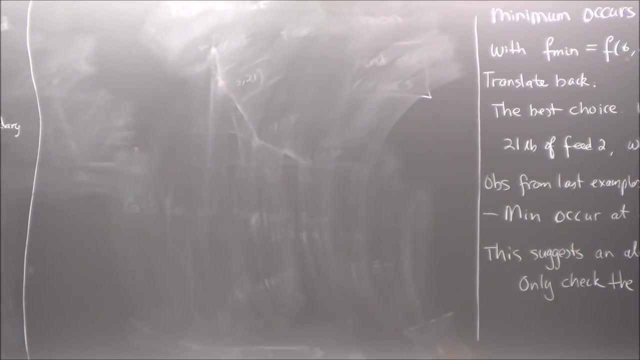 Let's take some examples. Okay, I'll give some examples. Okay, Okay, Okay, Are we okay? We need a break. No falling asleep. There was a semester I taught also a class. that's 75 minutes, a 400 level course. 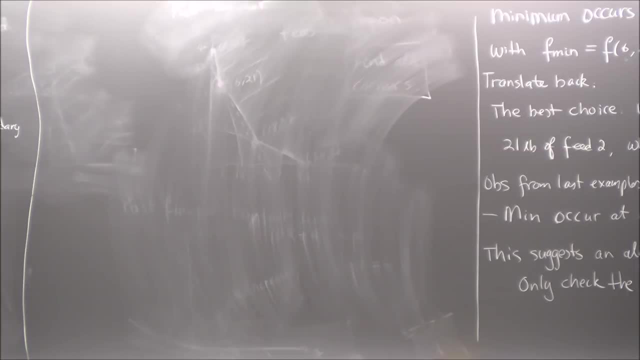 I know it's a bit rough to sit there for 75 minutes and not falling asleep. The only person could stay awake easily is the one standing here talking right? Yeah, I know I've been to sitting in talks. it's very hard to stay awake. 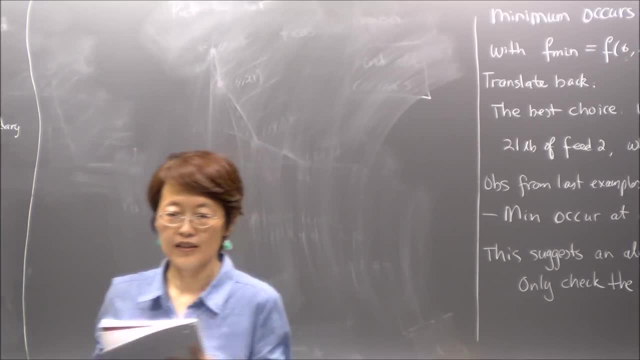 So what I did was we'd take like a couple of minutes break. just I don't know if you have funny jokes you want to share with the class, or I tell a little funny joke, So And then we have a laugh or we wake up. 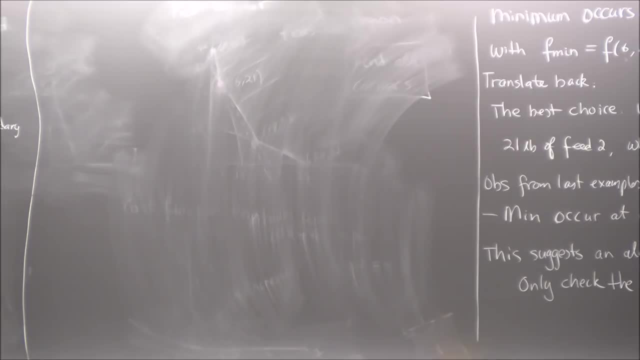 Mm-hmm. So I saw Shom, you've been in my class. Is that the 411? you took that? we took, we took, yeah, we took joke breaks. Do you remember any of the jokes you want to share with the class? 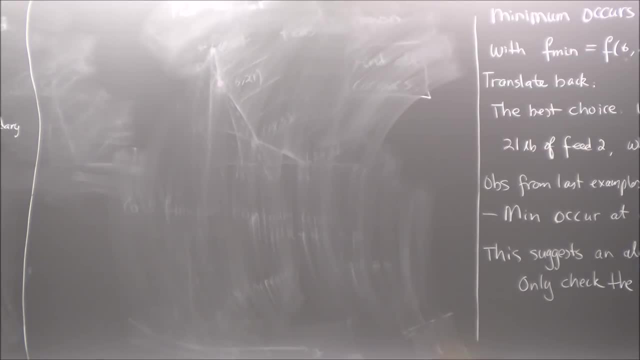 They were like the same ones you told over the summer too, like you would end your email if you like. Yeah, I have a collection of them. yeah, Okay, now it's against the policy of this course. This course we're doing math. that's really useful, right. 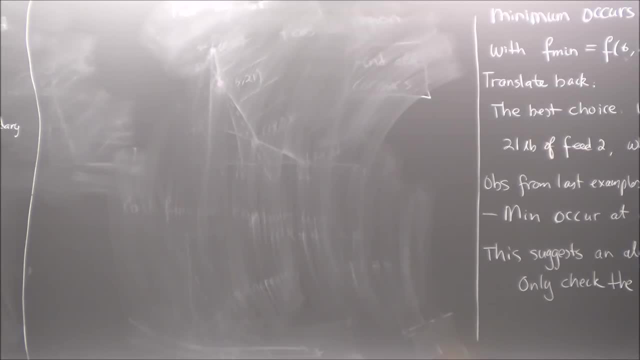 So, but some math are very abstract. So there is saying: says: a mathematician is a blind man sitting in a completely dark room trying to find a black cat that does not exist. So he's very quietly hunting for that black cat. 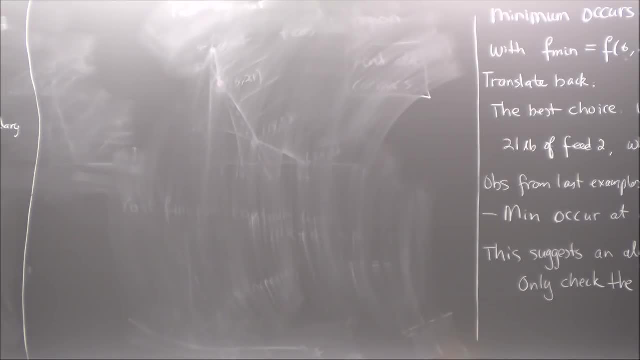 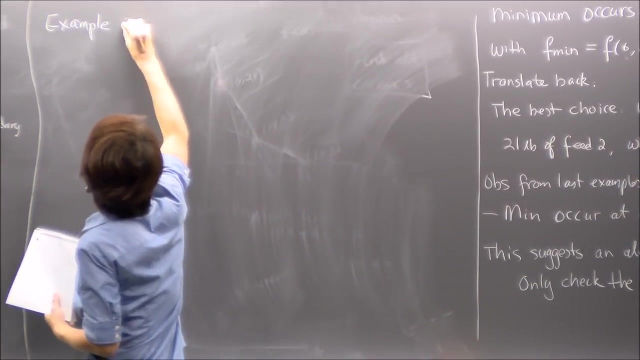 Okay, well, very much the same can be said about a philosopher, Do we agree? Except every now and then you will hear the philosopher yell: Yeah, caught it. okay, I'm the only one who's laughing. come on, guys. okay, let's take some examples. all right, okay, let's take an example for case number three. hmm, 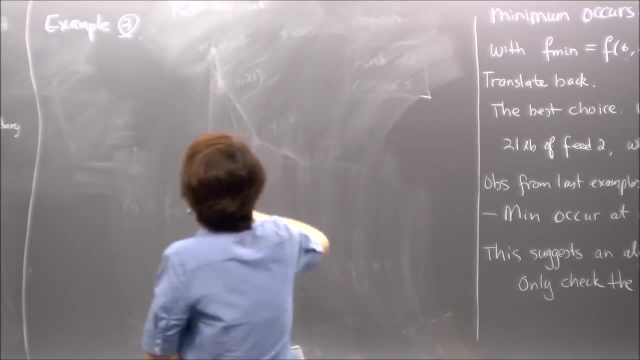 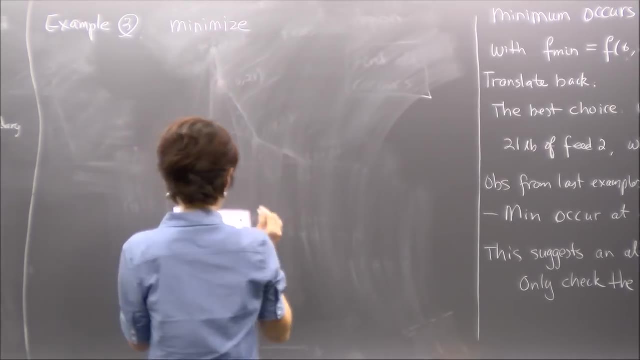 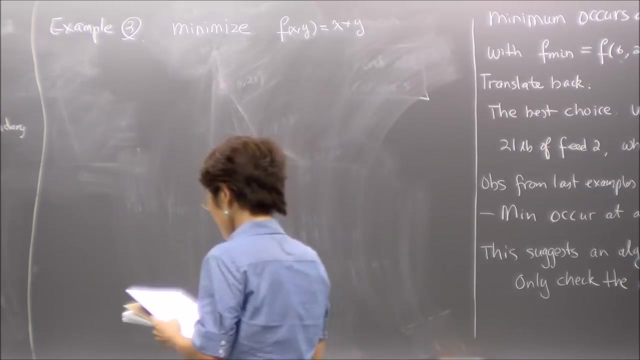 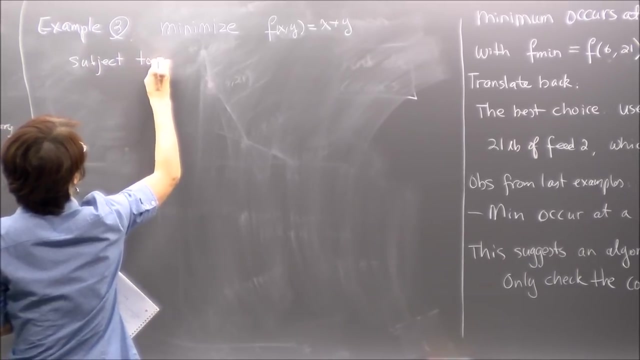 where the feasible region is empty. let's say it's not a word problem, it's just an abstract problem. let's say: I want to minimize some function, okay, and if you're not careful with your constraint, it could also happen in real life. the constraints are so bad that you just the problem is not solvable, so let's put. 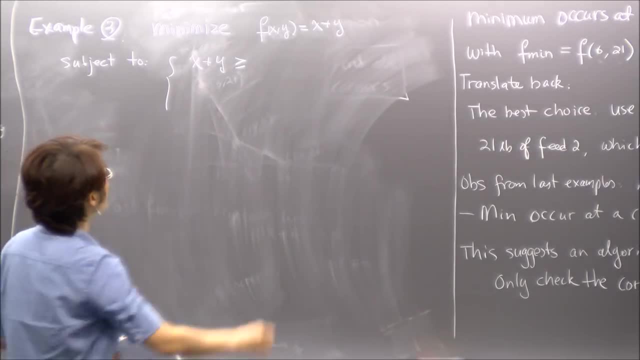 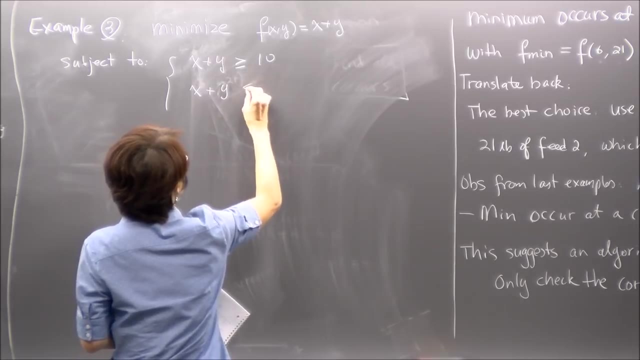 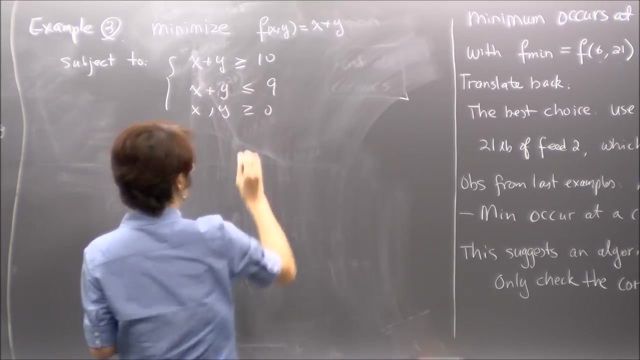 some silly constraints. so X plus Y, let's say, shall be bigger than 10, and then, at the same time, X plus Y, let's put it obvious, that's the 9 and X Y 0. is it possible to find some XY value that all these constraints are satisfied? no, because this number 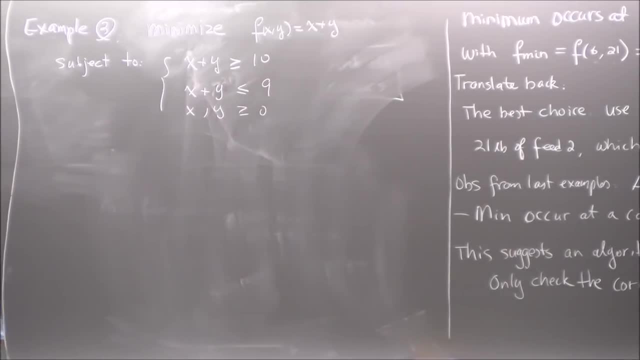 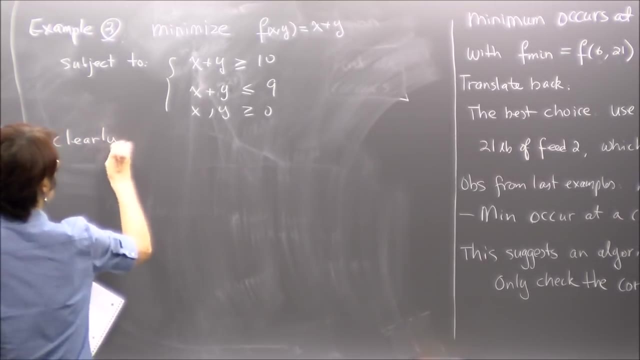 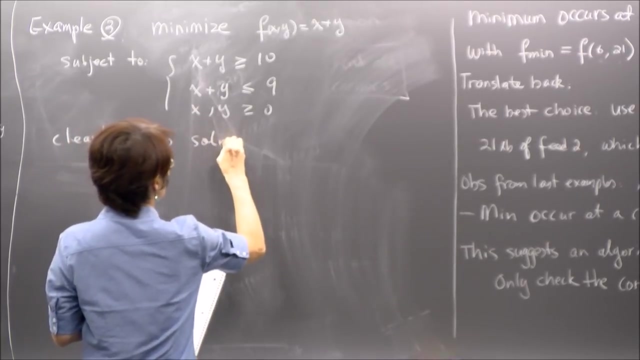 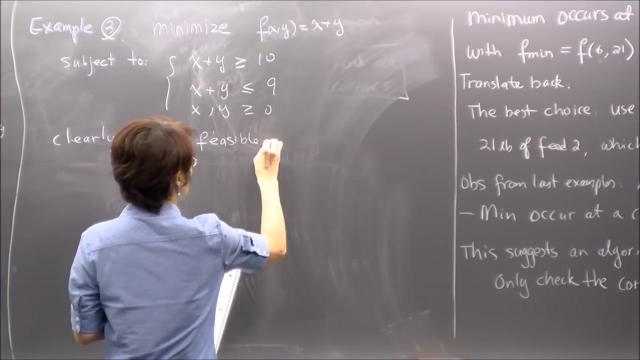 shall be bigger than 10 and less than 9 at the same time. that's not possible, right? okay? so can I write clearly? I don't want to offend, is it clear? right? so no solutions. okay, it's not even feasible. let's say not feasible, okay, and 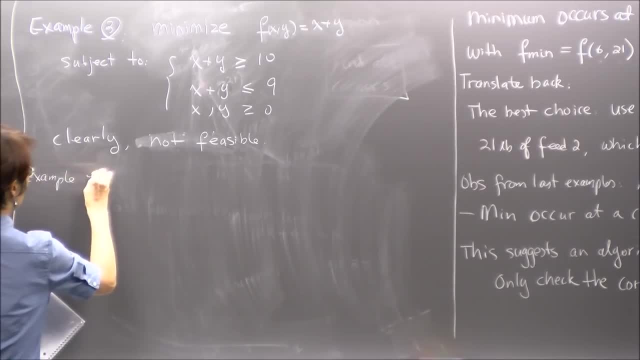 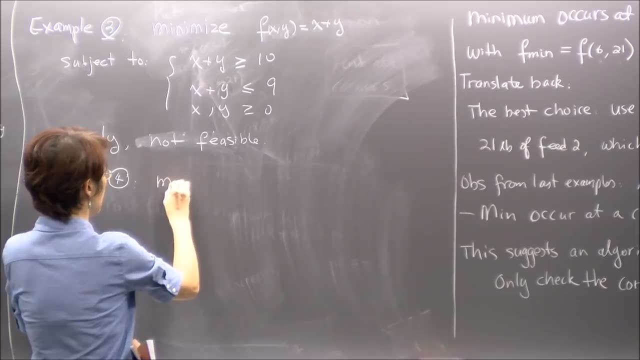 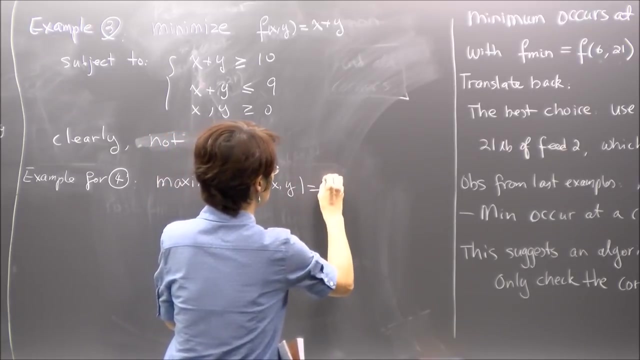 let's take an example for the case number four here that this is solutions unbounded. well, you can easily cook up many problems like that. so let's say I want to maximize some function. I can put anything here. let's just put X plus Y, it doesn't matter. 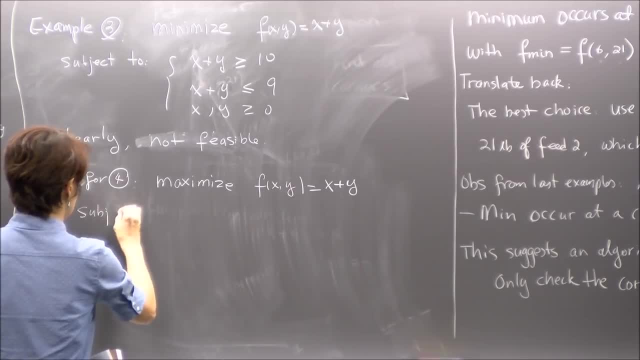 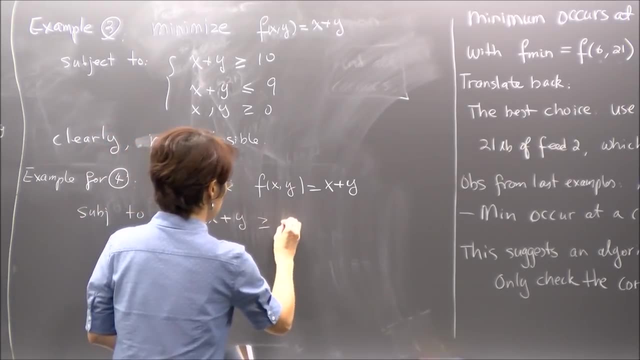 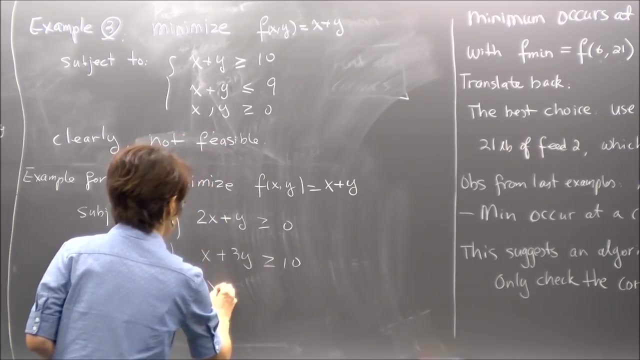 nothing fancy, subject to the following: so I have 2x plus Y bigger than zero, and X plus 3y bigger than 10, XY bigger than zero. so I want to maximize the sum of X plus Y. with this constraint. where will I find the maximum? XY? the positive, so you. 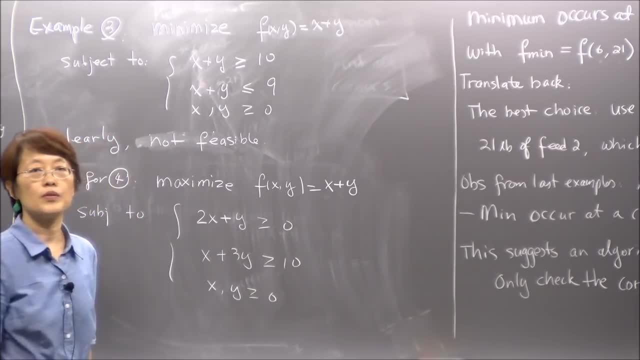 see, I should make them as big as possible. is that right? the bigger the better. the but the constraint has no upper bound for the X and Y value, so I can take them as big as I want. so the maximum value is unbounded. it can go to infinity, do we? 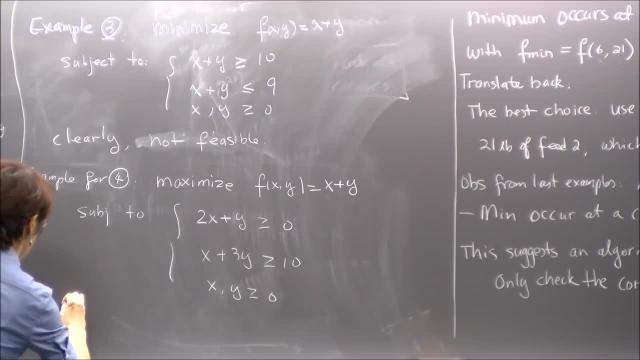 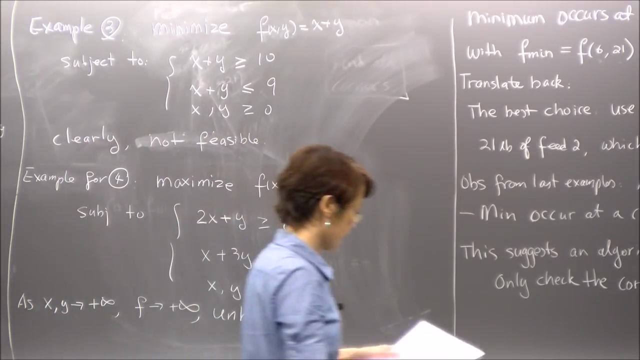 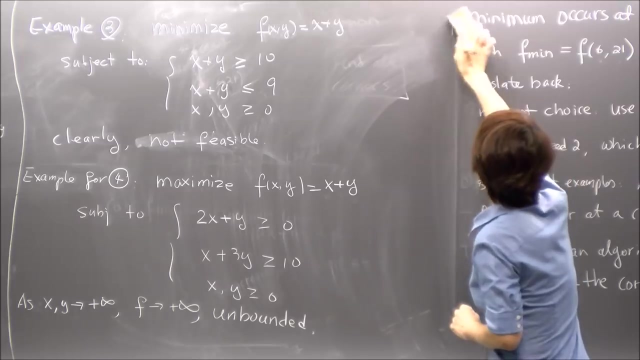 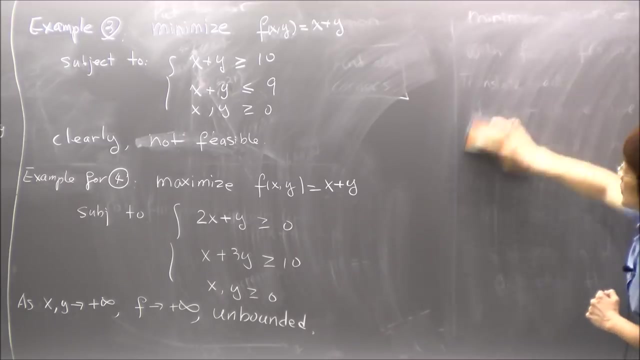 see that. so we see that as XY goes to plus infinity, my function F goes to plus infinity, so it's unbounded. so that can happen also. okay, okay. so that's all I'm gonna say for the graphing method, for LP, problem with two variables. and in your homework you will have four little problems for 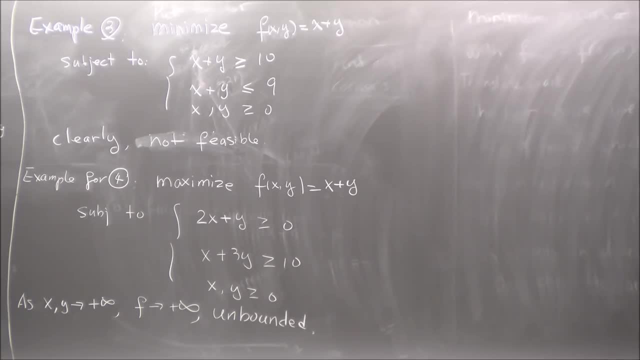 you to practice and have fun with. okay, it's up. I don't expect it to work, but it to be a big homework set. but practice that and make sure you you know how to do it. so what we will do now and maybe next week, a big chunk of time we will spend on- will be um learning how to. 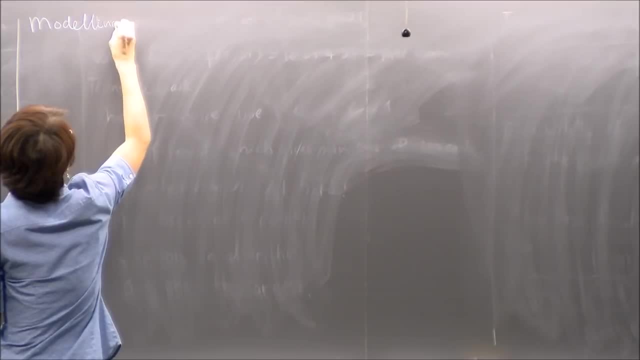 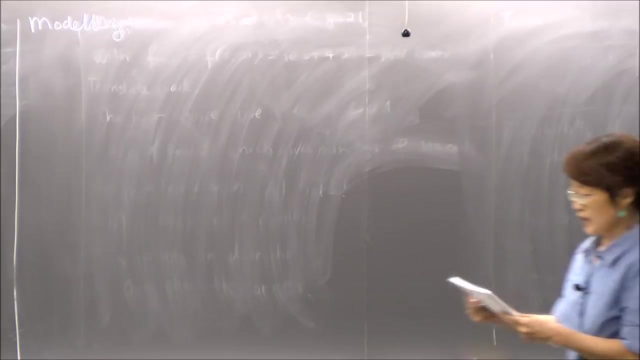 do modeling. so we will go through a set of model problems from simple ones and then we'll make it more complicated and we'll have more complicated models and we'll set up the linear programming problem but not solving it. that comes later, is that okay? okay, so, if you have the textbook, 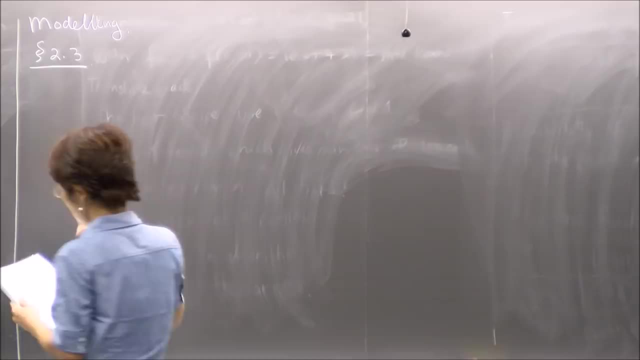 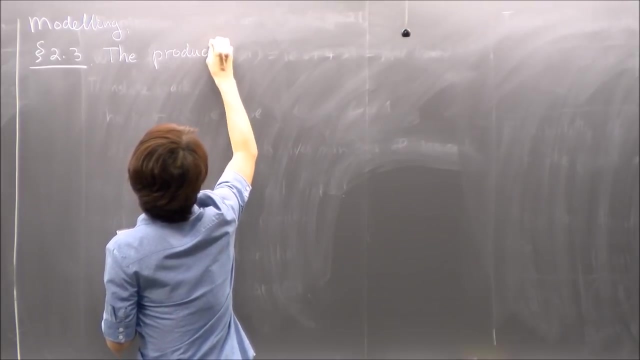 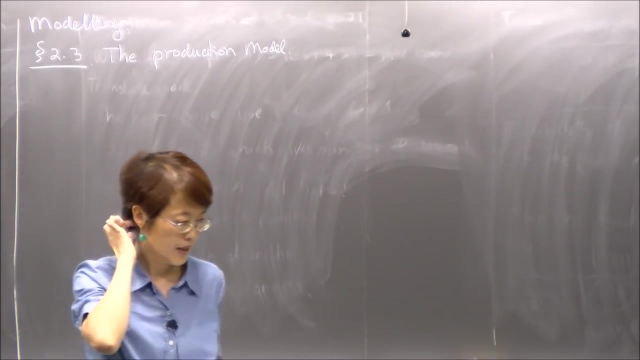 what comes here is from two point, chapter 2.3. so this is one situation um production model. okay. so here's a setting: you are a factory and you want to produce a list of products. okay, so you might have two or three, and each of them you can sell on the market. 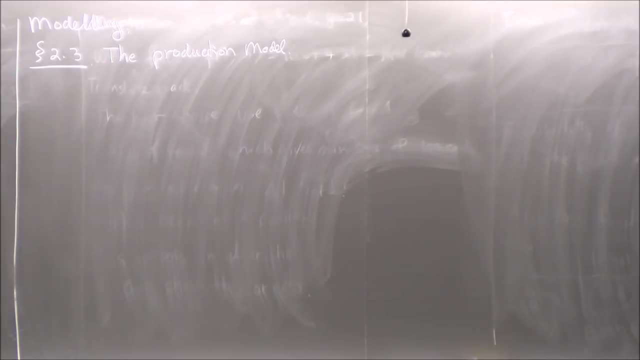 with certain price, so that's your profit. okay, you know, and assume you can sell all of them, and then to produce each of these items you need some resources, you need raw material, you need labor, you need use some machine or whatever, so they might be limited. okay, so your goal now will be: 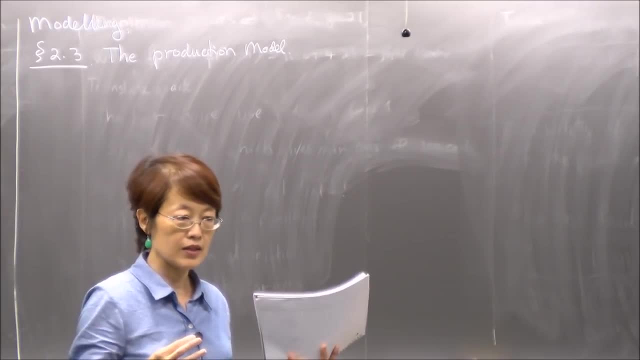 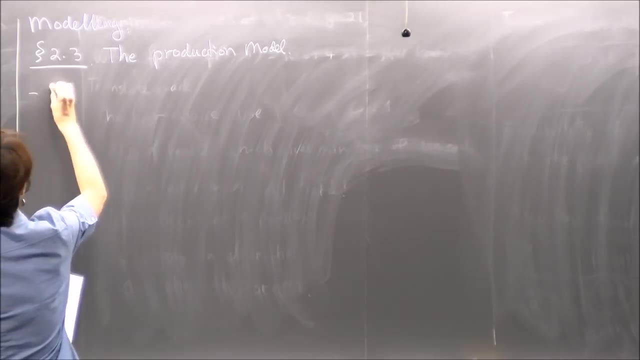 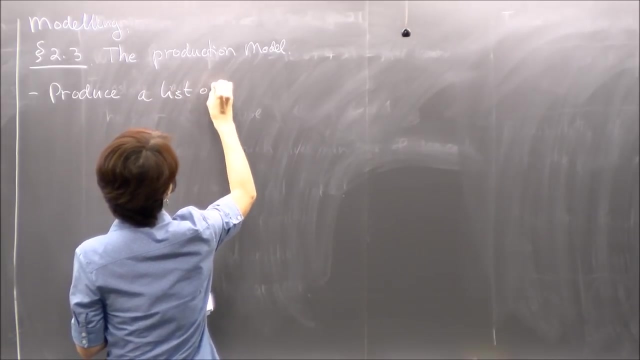 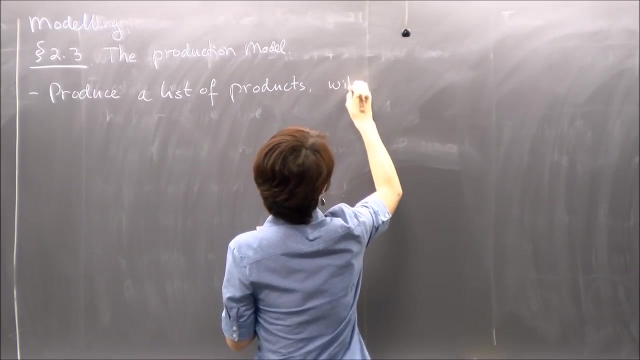 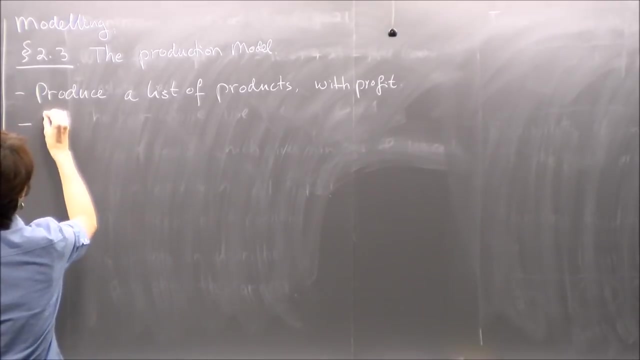 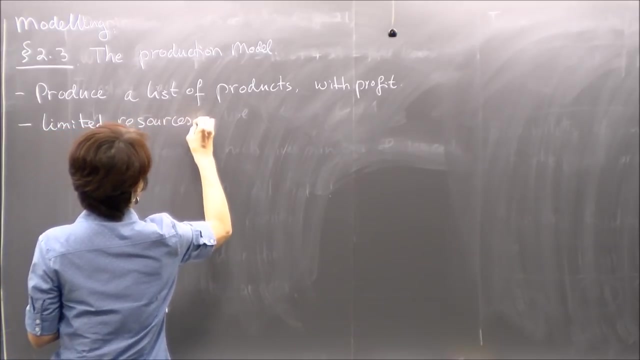 maximize your profit and within the range of limited resource, okay, so let me put this up. so so first i am produce, i'm producing a list of products, okay, and then each one has a price or profit, which i know how much money i can make from each, but then i have limited resources. okay, these could be like raw material. 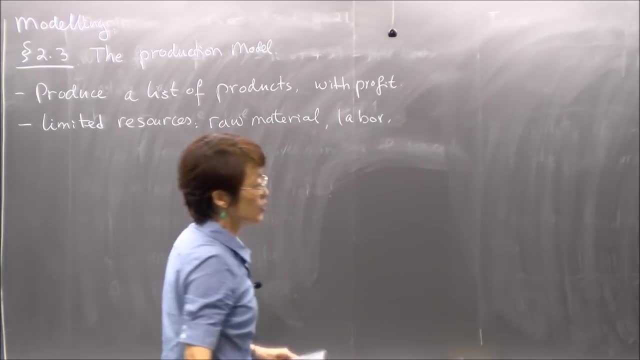 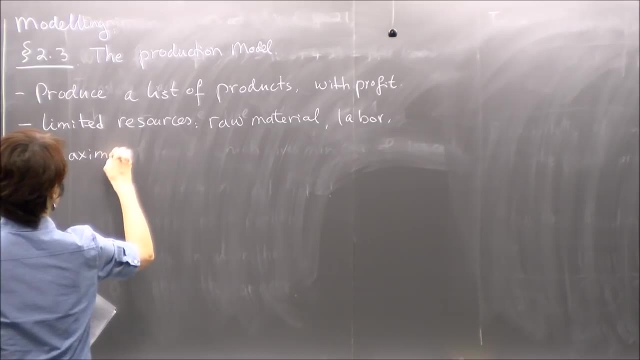 labor or whatever capital or whatever many of them, and then your goal here will be maximize the profit. okay, so this will typically end up in the maximization problem, right? okay so, um, let's take an example. i i just take the one from the book. example two, three one: let's go through that. okay, so a company wants to produce two types of boats. 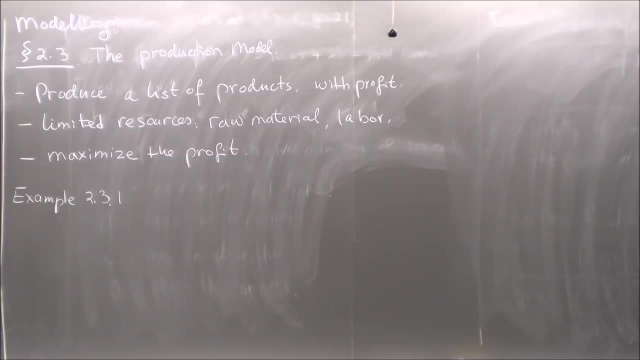 so in the textbook this is written, a long paragraph and lots of explanation of the situation. so let's pour out the key thing. so i'm producing two types of boats. i'm going to call it. i will call them type a and type b, it's okay. or you can say one is a selling boat and the other is a. 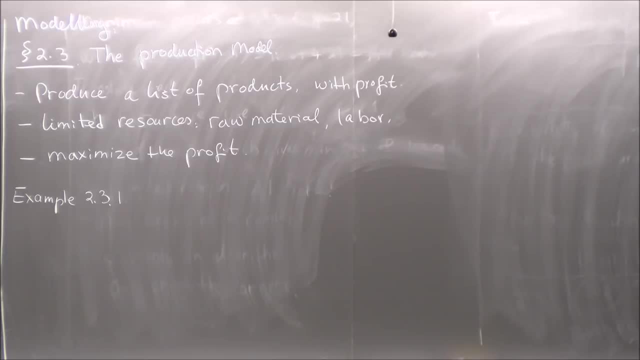 luxurious yacht or whatever. call it a and b, all right. so produce two types of boat, boats, so i call them type a and type b, just to be a bit abstract. and then to produce that i use, i need resources. so what are the resources i need to? 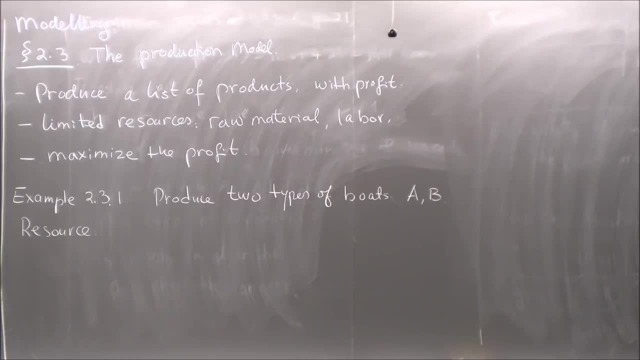 make these both so raw material. let's say i need to use. um, these right here, these are tensors, the. so raw material. let's say i need to use, you know, soyный lá pc. this shows the overall mass of the. so what are the resources i need to make these boats so raw material? let's say i need to use. 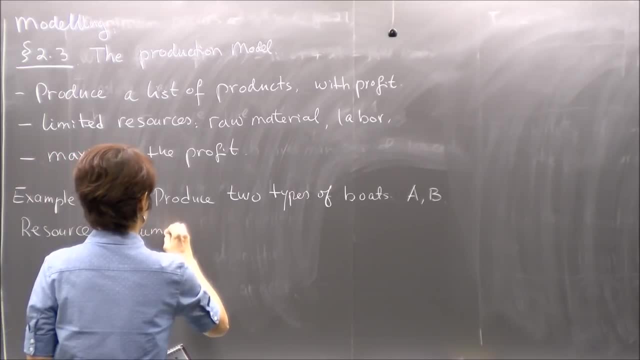 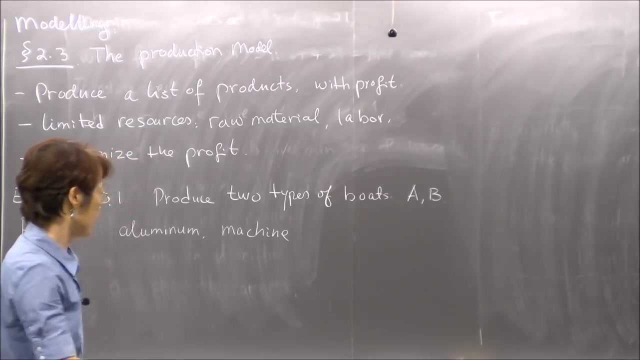 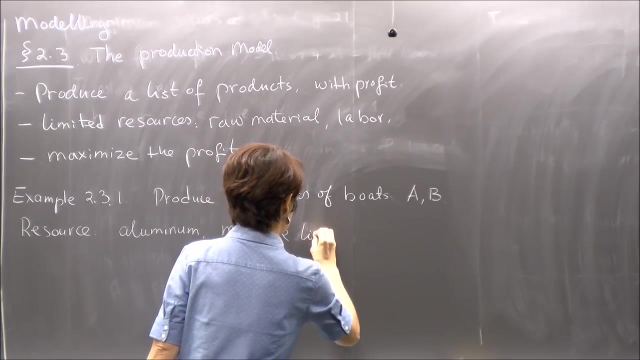 aluminum, that's my raw material, and then to to work on the boat. there is some machine that I need to use, but I have limited number of hours I can. I can use some machine time. I cannot run this machine to an unlimited amount of time, okay, and I have a group of workers that they work for me for certain hours, so I 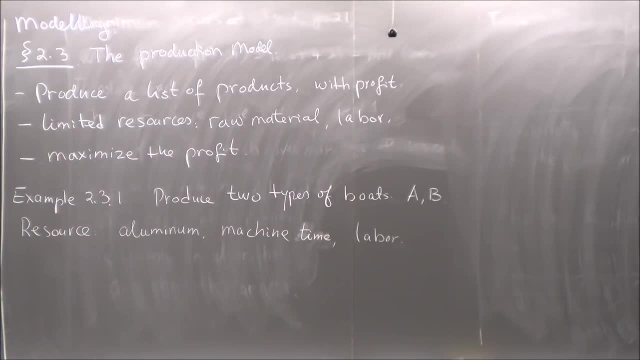 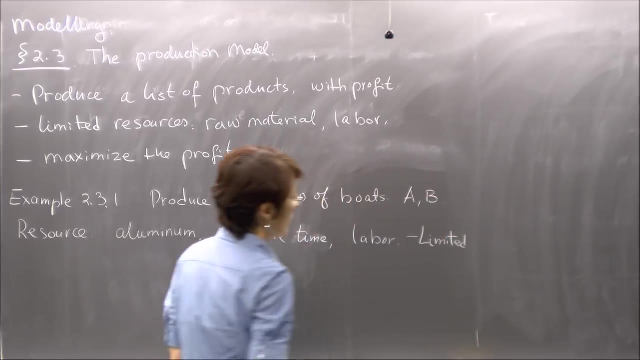 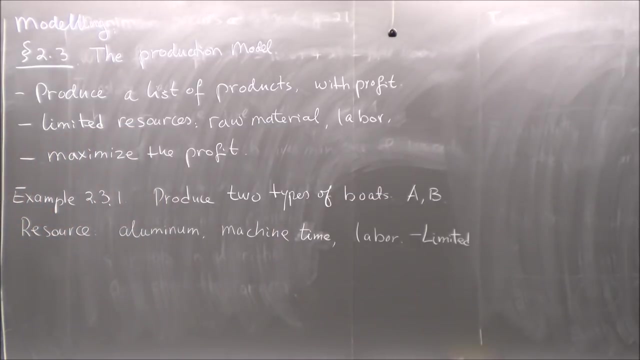 have labor. okay, these are the resources and these, somehow they are limited. so that's the point that gives me the constraint. so I don't have infinite amount of aluminum or machine time or labor at my disposal, so I I have to stop. okay, so I can put all these in a table. so 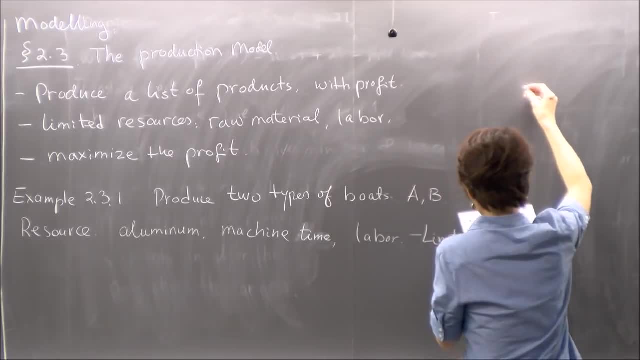 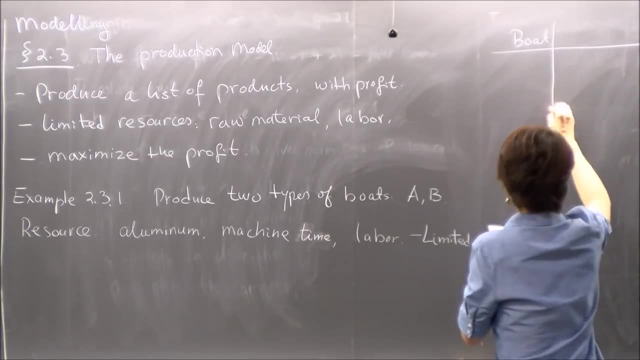 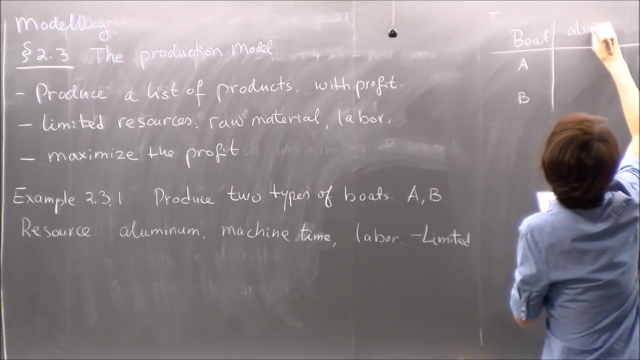 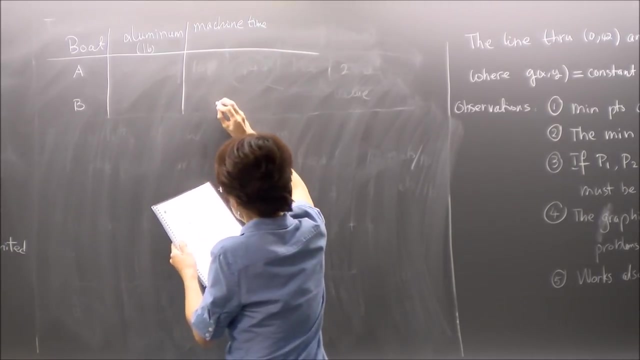 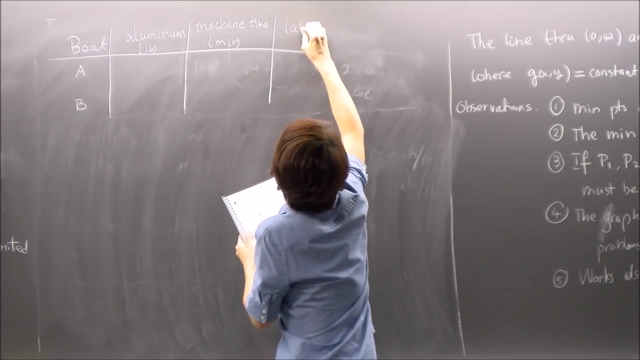 let's see, let's do that, so I put it in the table. so boat type here, mm-hmm, so I have type a and I have type B and let's see aluminum. okay, let's say the unit is pounds and the machine time. well, let's say minutes, it doesn't matter, it's just the unit and labor. okay. 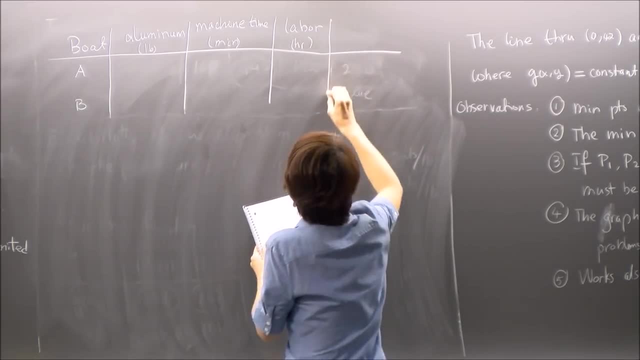 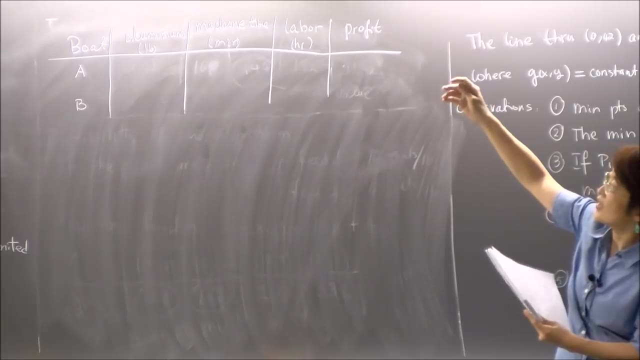 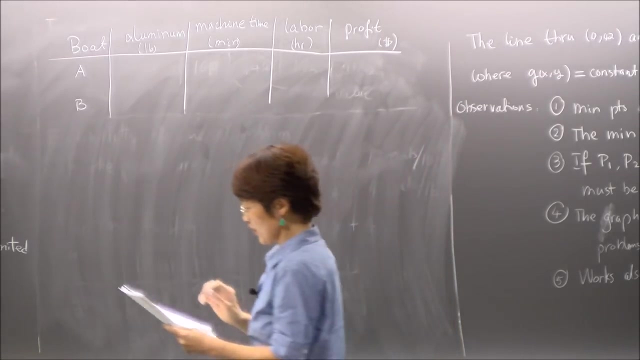 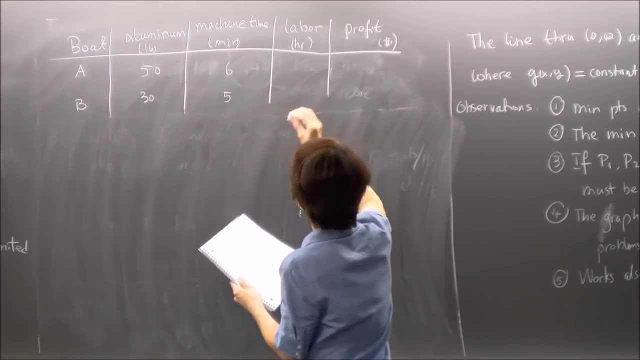 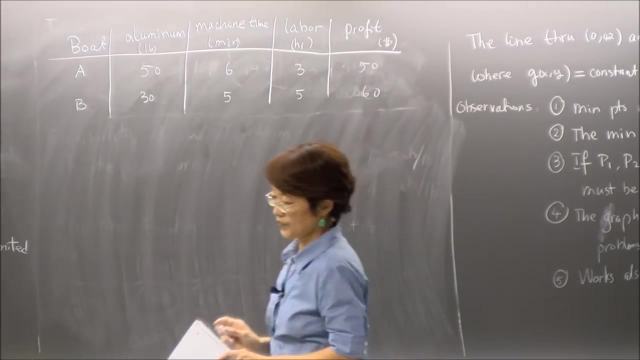 so how many hours I have? okay. and then there is a profit. so in this profit- I already did the math- the final sale price minus whatever the, the, the material cost and so on, so forth. okay, that's the pre-op profit here. so that's in dollar. so let me put up so 50, 30, 6, 5, 3, 5, 50, 60. so that is already a. 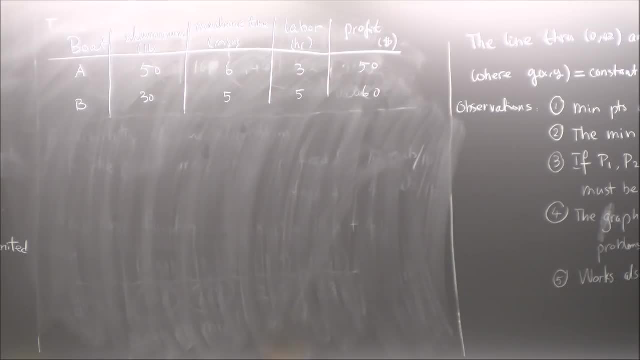 step. so usually you have a problem. it's all described by word and you should first set up this table. okay, to get all the information organized. so you see it very clearly. and then now comes the constraint, because I have limited resource. so maximum resource that I could use for each of these items are: 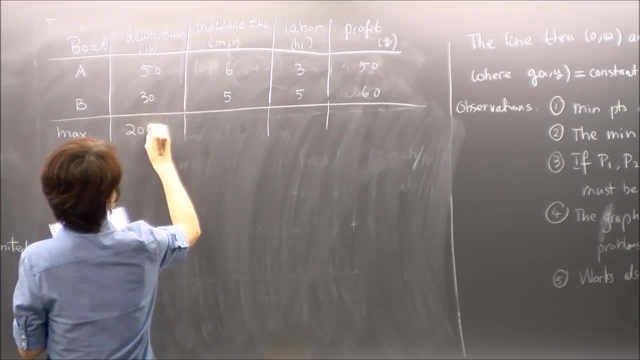 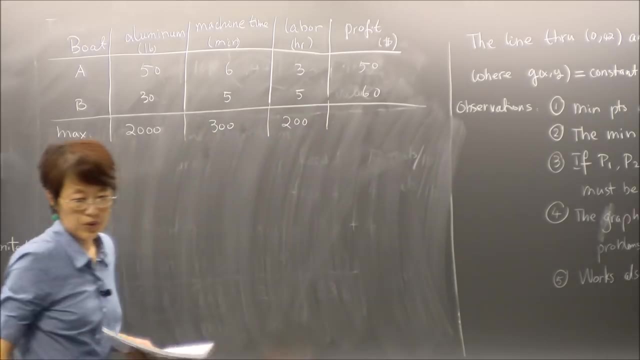 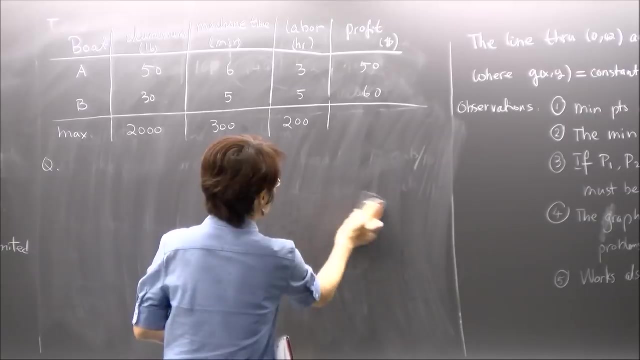 listed. so I can use at most 200 pounds of aluminum, 300 minute of the machine and 200 hours for my labor. is that clear? so that is the situation. okay, so here comes the question. so so you are the manager of that branch. you have to make a decision. 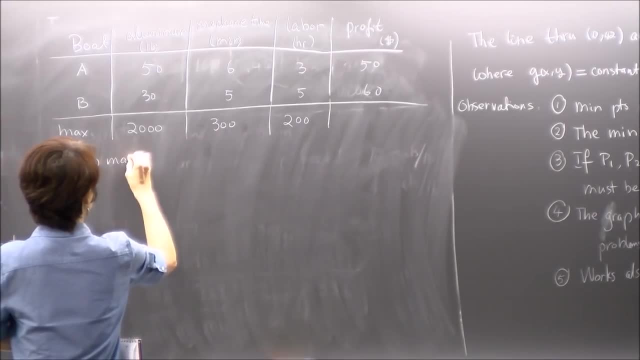 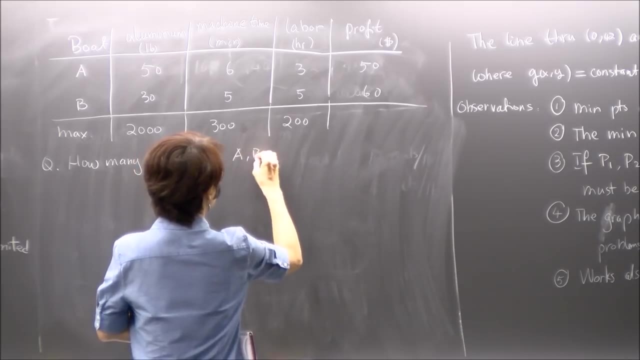 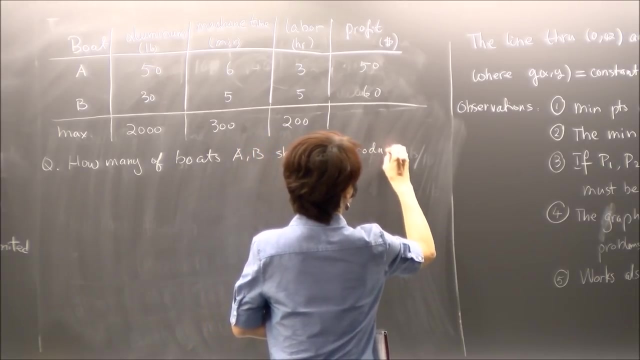 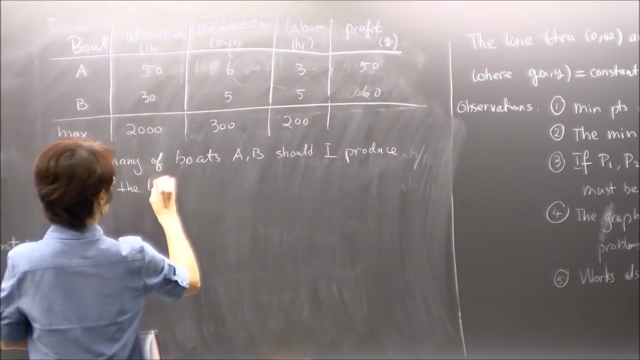 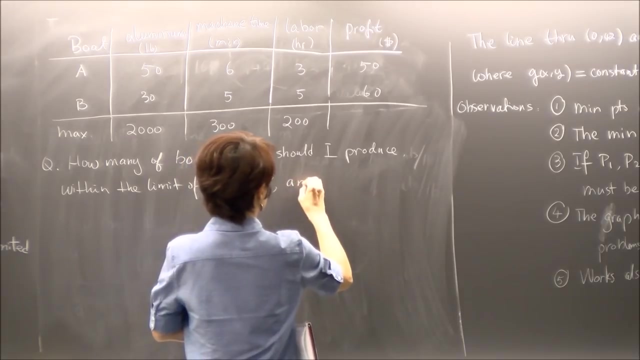 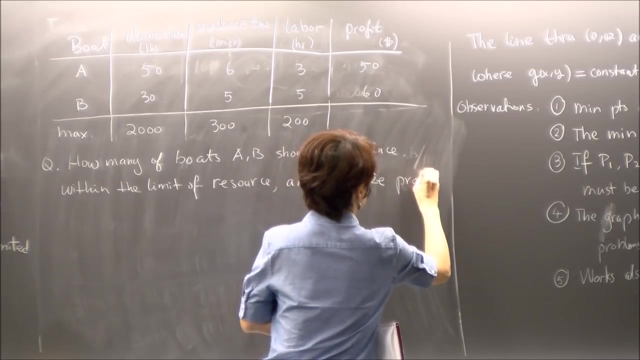 so how many of votes a- B should I? should I produce okay and within the limit of resource and maximize my profit? you have to make a decision. I'm going to produce okay and within the limit of resource and maximize my profit. you have to make a decision. I'm going to produce 10 of both a and 20 of both B, or what? 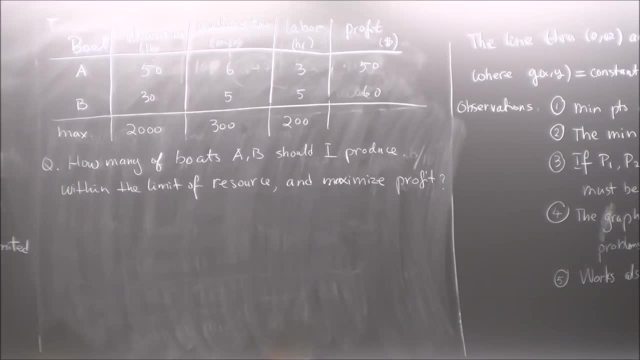 produce 10 of both a and 20 of both B, or what produce 10 of both a and 20 of both B, or what? what will be a good number for me to what will be a good number for me to what will be a good number for me to do? is it clear the setting mm-hmm. okay, so. 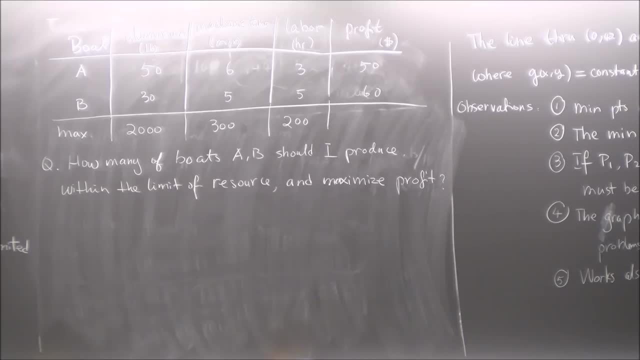 do is it clear the setting mm-hmm? okay. so do is it clear the setting mm-hmm? okay. so how do we set up this model. so here's how do we set up this model. so here's how do we set up this model. so here's the modeling part. I see, I still think. 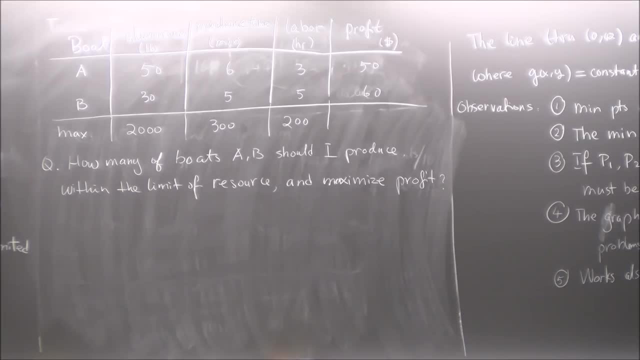 the modeling part. I see, I still think the modeling part. I see, I still think this is a very sorry should go come here. this is a very sorry should go come here. this is a very sorry should go come here. so here's the modeling part, so here's the. 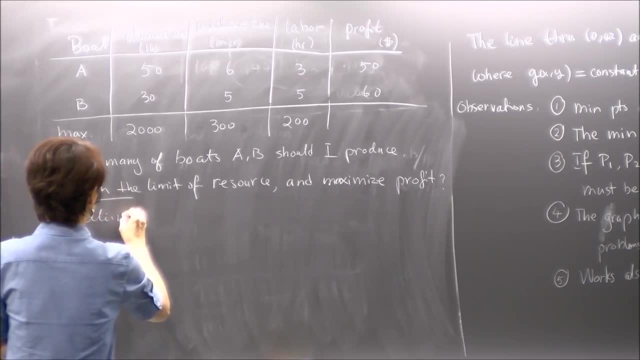 so here's the modeling part. so here's the modeling part. so here's the modeling part. this is a very modeling part. this is a very modeling part. this is a very standard situation. everything is listed. standard situation. everything is listed. standard situation. everything is listed on this table. I think you could. 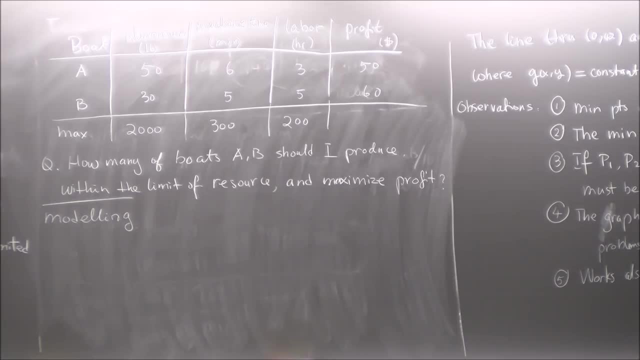 on this table. I think you could on this table. I think you could probably do it by yourself. would we be probably do it by yourself? would we be probably do it by yourself? would we be able to do that? anybody wants to help me able to do that? anybody wants to help me? 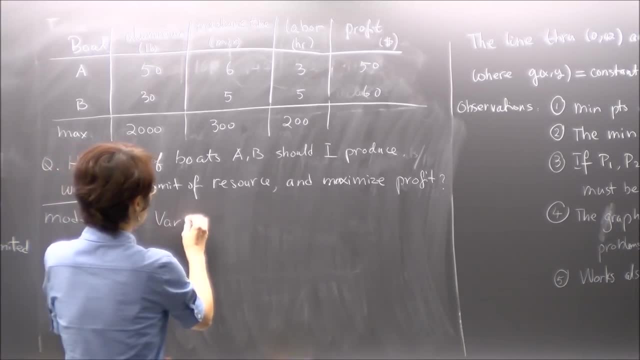 able to do that. anybody wants to help me out? hmm, so what variables should I out? hmm, so what variables should I out? hmm, so what variables should I define? what is the decision I have to define? what is the decision I have to define? what is the decision I have to make here in the question I have to? 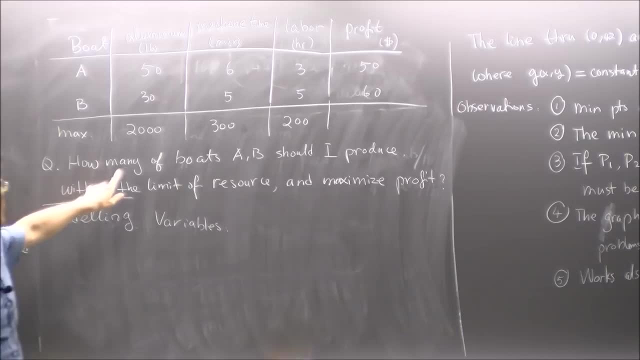 make here in the question I have to make. here in the question I have to decide on what. how many of both a and B decide on what? how many of both a and B decide on what? how many of both a and B? right, those are the two numbers that I 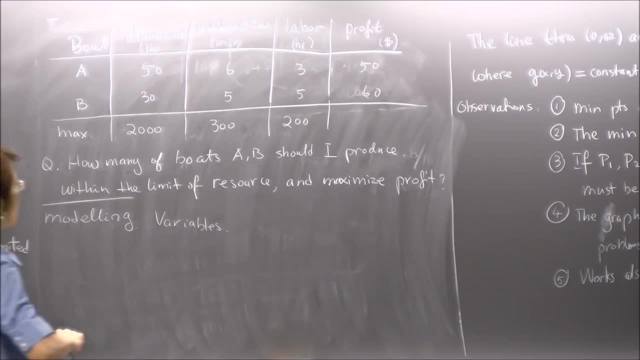 right. those are the two numbers that I right. those are the two numbers that I need to decide right to produce. so I need to decide right to produce. so I need to decide right to produce. so I would call these my variables, so any would call these my variables, so any. 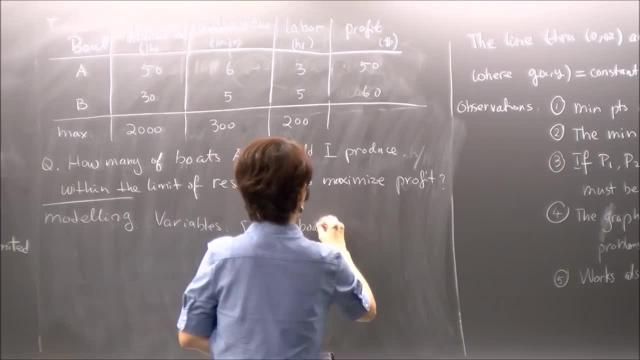 would call these my variables. so any will be. number of both type a and B will be number of both type a and B will be number of both type a and B. will be number of both B for me to will be number of both B for me to. 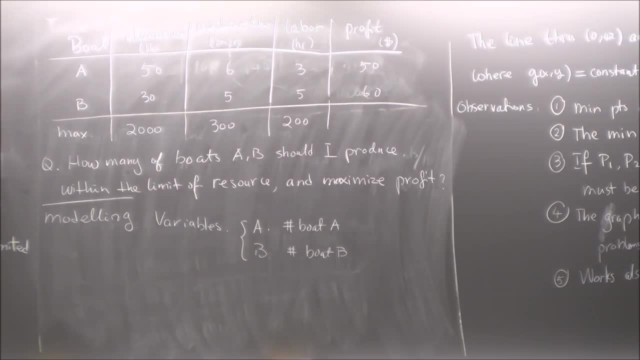 will be number of both. B for me to produce, so those will be produce. so those will be produce. so those will be the things I decide and my variables. okay, okay, let the things I decide and my variables. okay, okay, let the things I decide and my variables. okay, okay, let me go up. don't write too. 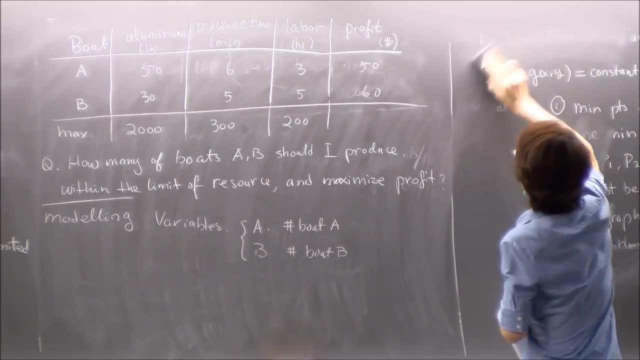 me go up. don't write too me go up. don't write too long. you sit in the back. you can't really long. you sit in the back. you can't really long. you sit in the back. you can't really see. let me use the upper part of. 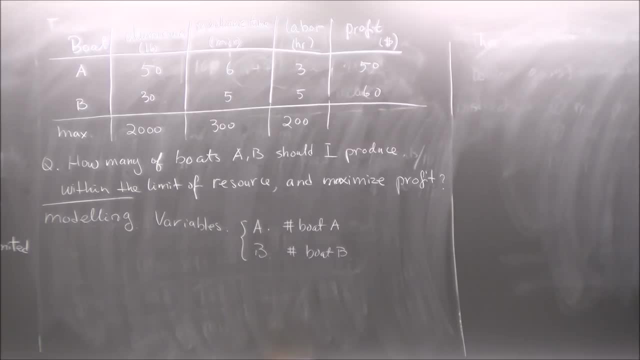 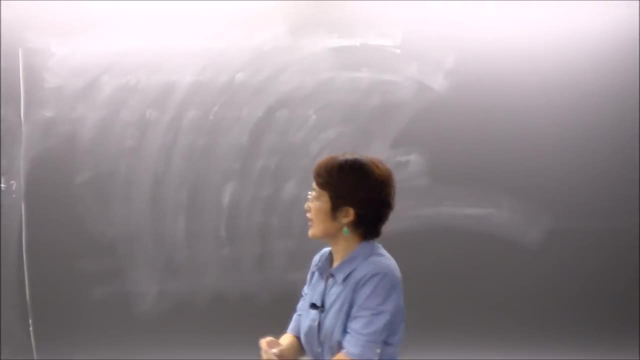 see, let me use the upper part of? see, let me use the upper part of the board. okay, so now we don't have a cost the board. okay. so now we don't have a cost the board. okay, so now we don't have a cost function. this problem is slightly 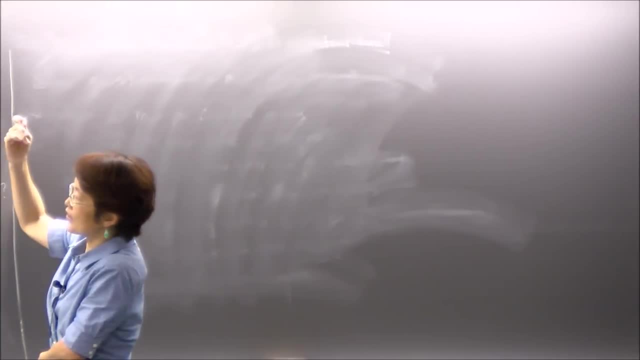 function. this problem is slightly function. this problem is slightly different. what we have is a gain different. what we have is a gain different. what we have is a gain: function that it's a profit, or function that it's a profit, or function that it's a profit or right. so I actually gain something. I 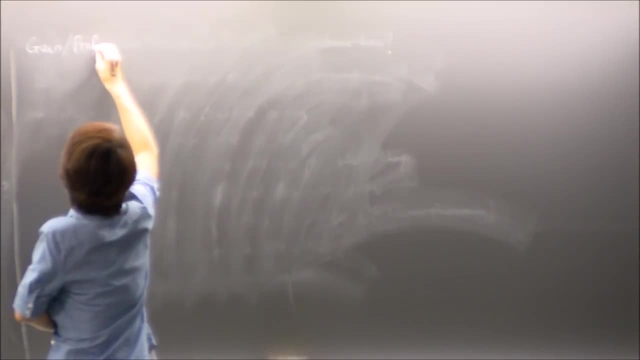 right, so I actually gain something. I right, so I actually gain something. I want to maximize it. so you can call it a want to maximize it. so you can call it a want to maximize it. so you can call it a gain function or a profit function. okay, 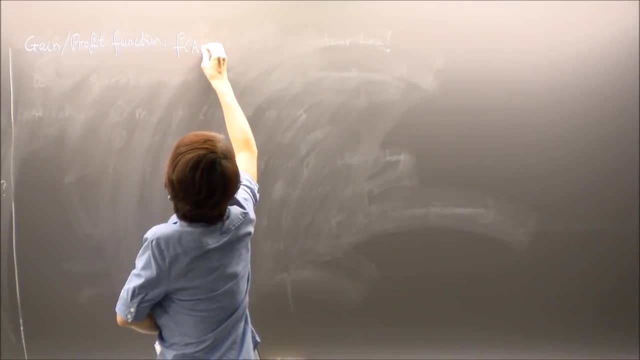 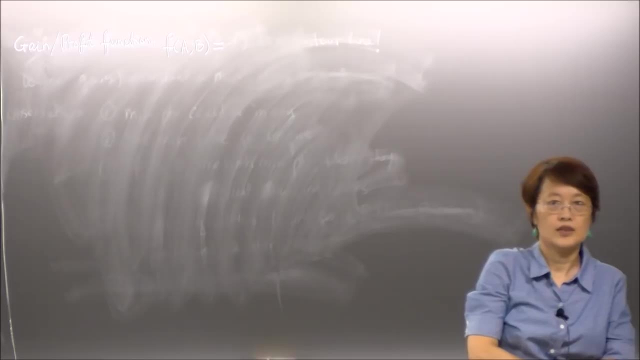 gain function or a profit function: okay, gain function or a profit function. okay, so a function depending on a and B. which? so a function depending on a and B. which so a function depending on a and B, which will be my profit in this case. so will be my profit in this case. so 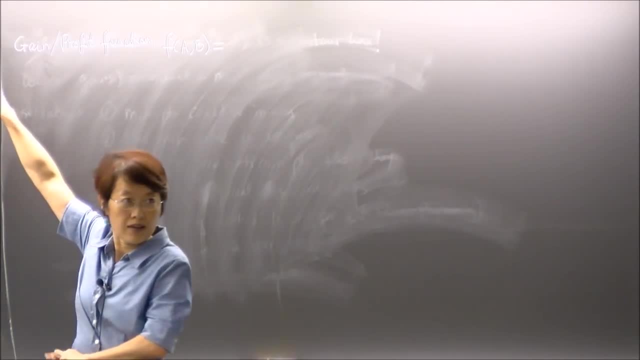 will be my profit in this case. so did we say that we multiply the first row? did we say that we multiply the first row? did we say that we multiply the first row by a that variable we call and the? by a that variable we call and the? 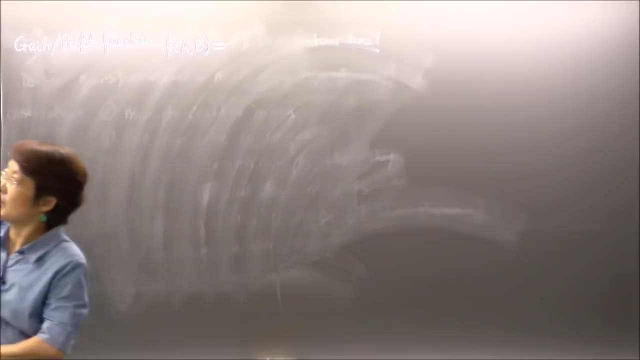 by a, that variable we call, and the second one by B, and then we add them up, second one by B, and then we add them up, second one by B, and then we add them up vertically. is that right the same thing? vertically, is that right the same thing? 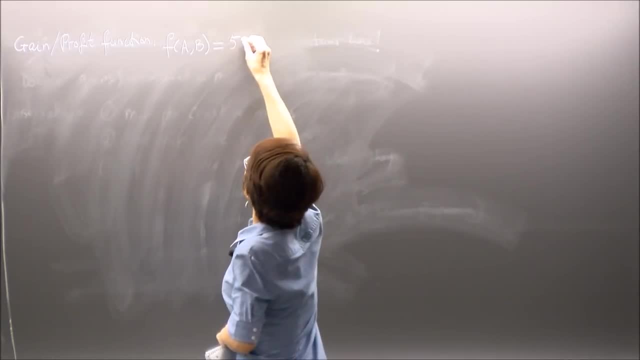 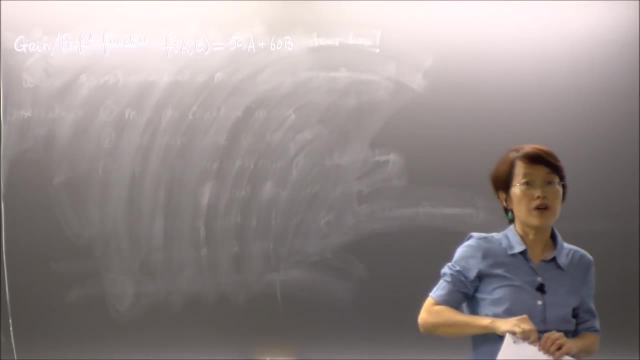 vertically. is that right the same thing here. right, so I would have 50 a plus 60 here. right so I would have 50 a plus 60 here. right so I would have 50 a plus 60 B. that will be my profit, right so the? 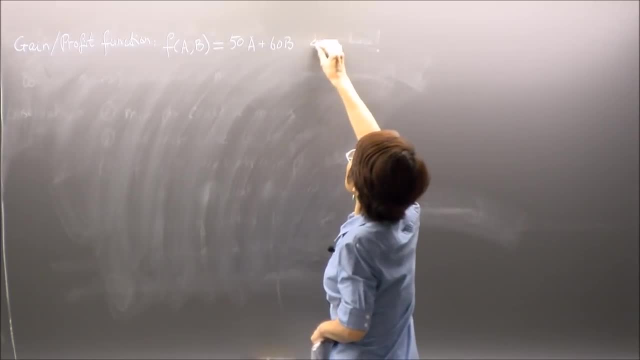 B, that will be my profit right. so the B, that will be my profit right. so the difference here is: I want to maximize difference. here is: I want to maximize difference here is: I want to maximize this, this, this, I not minimize, I want to maximize it. I not minimize, I want to maximize it. 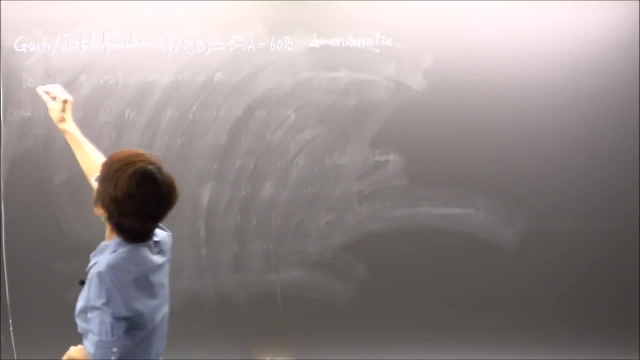 I not minimize, I want to maximize it. okay, okay, subject to constraints. I think, okay, okay, subject to constraints. I think, okay, okay, subject to constraints. I think that's all standard. so let's say I have, that's all standard. so let's say I have, that's all standard. so let's say I have three constraints: aluminum, aluminum. 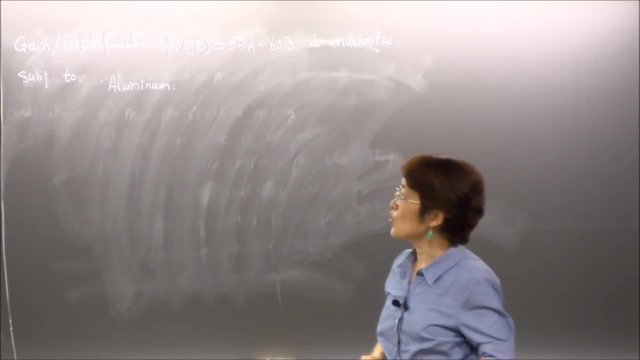 three constraints aluminum- aluminum. three constraints aluminum- aluminum. total amount is 2,000 pound. I cannot go. total amount is 2,000 pound. I cannot go. total amount is 2,000 pound. I cannot go above that. so what will I have? so if I 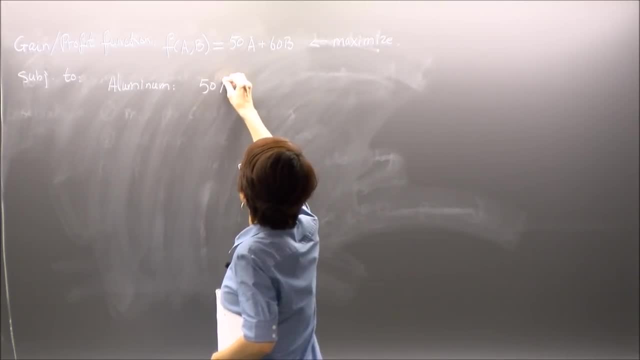 above that. so what will I have? so if I above that? so what will I have? so if I add up the first, add up the first, add up the first column, it gives me 50 a plus 30 B, that will column. it gives me 50 a plus 30 B, that will. 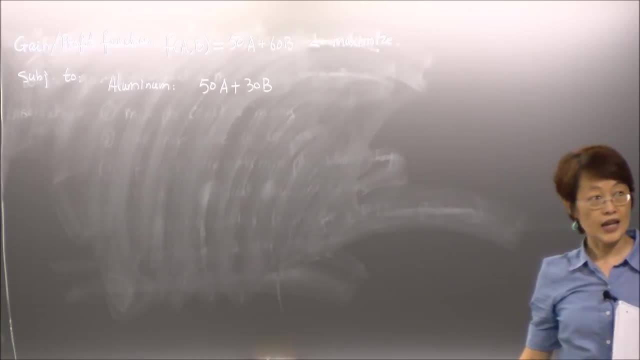 column. it gives me 50 a plus 30 B. that will be the total aluminum I will use and be the total aluminum I will use and be the total aluminum I will use, and that has to be. how shall that relate to? that has to be. how shall that relate to? 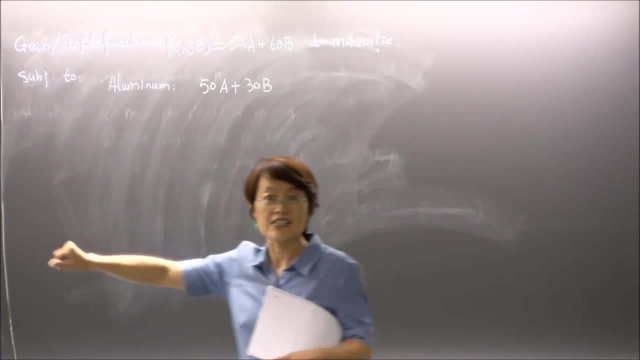 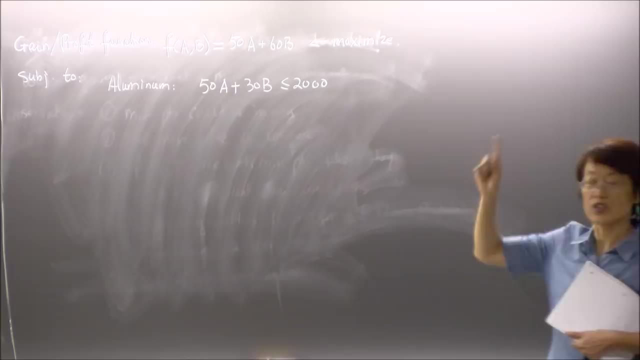 that has to be. how shall that relate to 2,000 less than is that right? I cannot. 2,000 less than is that right, I cannot. 2,000 less than is that right, I cannot go above. is that clear? so the new: go above. is that clear? so the new. 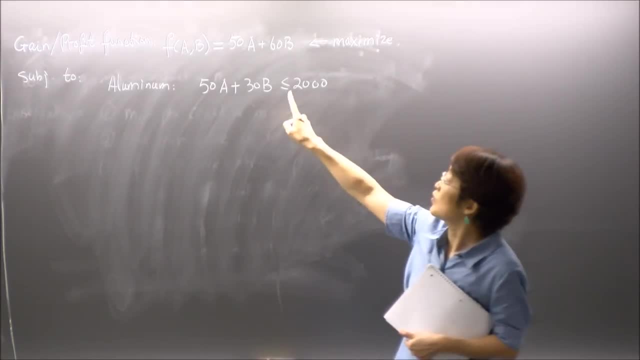 go above. is that clear? so the new change here is: now it's maximizing, and now my change here is: now it's maximizing, and now my change here is: now it's maximizing, and now my constraint is less than constraint, is less than less than constraint is less than less than okay. that's it okay. so the rest shall be. 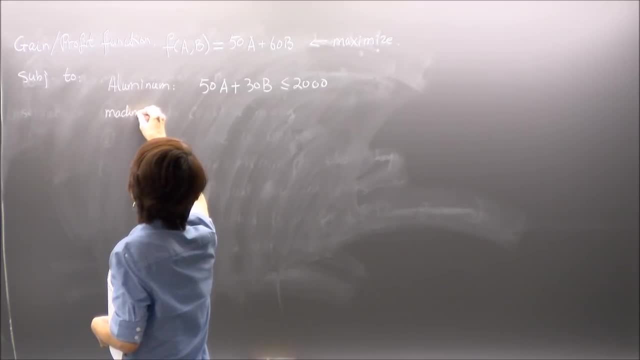 okay, that's it okay, so the rest shall be okay. that's it okay, so the rest shall be pretty straightforward. machine time is pretty straightforward. machine time is pretty straightforward. machine time, is it okay? so I add up vertically 6a plus it okay? so I add up vertically 6a plus. 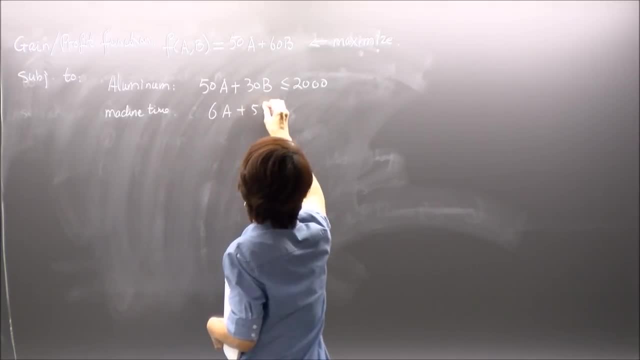 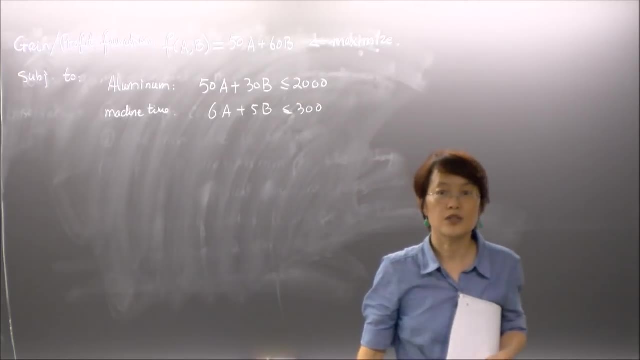 it okay. so I add up vertically 6a plus 5b and I cannot exceed 300 because I 5b and I cannot exceed 300 because I 5b and I cannot exceed 300 because I don't have access to more than that. 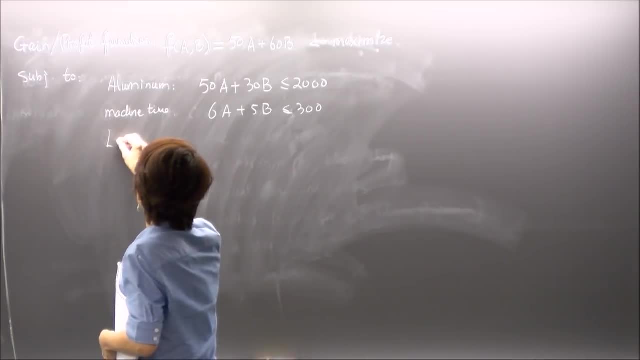 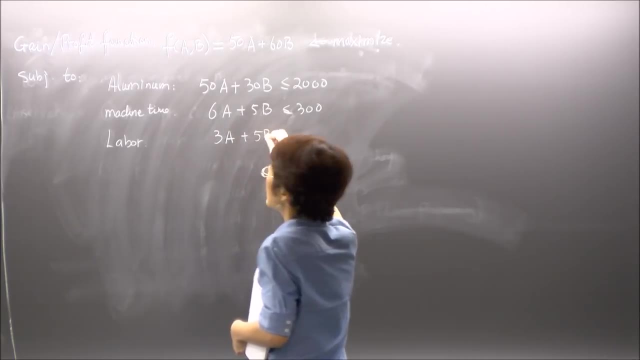 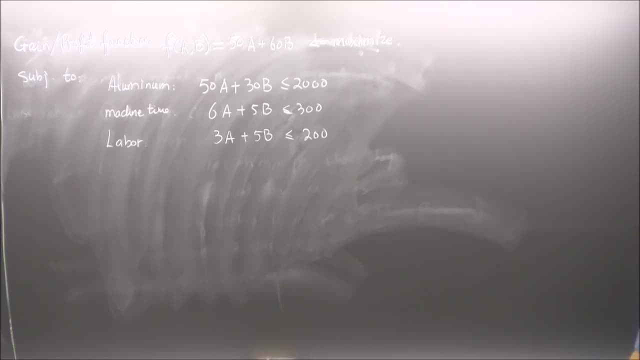 so 3a plus 5b: now I have only 200. not so 3a plus 5b: now I have only 200, not more than that. is it clear? any questions more than that? is it clear? any questions more than that? is it clear? any questions? it's okay, am I done? did I forget? 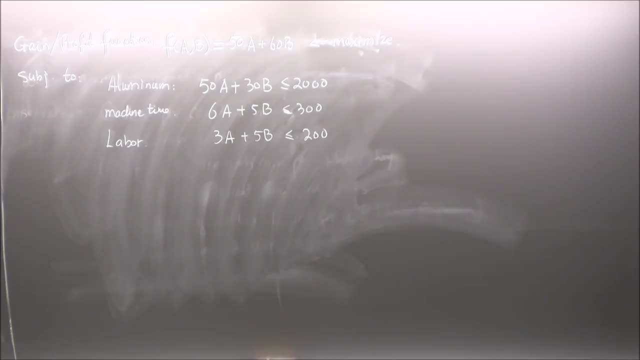 it's okay, am I done? did I forget? it's okay, am I done? did I forget something mm-hmm and what? what do I have something mm-hmm and what? what do I have something mm-hmm and what? what do I have to put up? yes, I cannot produce negative. 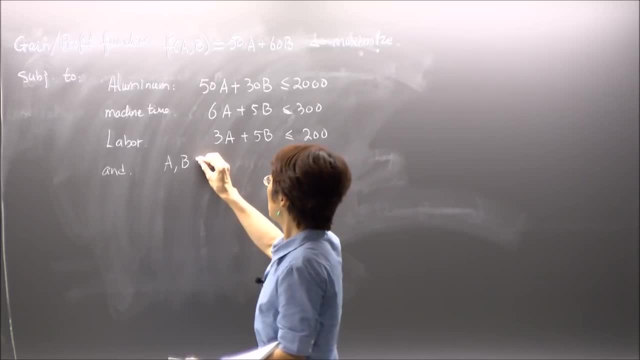 to put up. yes, I cannot produce negative to put up. yes, I cannot produce negative. amount of bones- is that right? so I amount of bones. is that right, so I amount of bones. is that right? so I always have that okay, so always take. always have that okay, so always take. 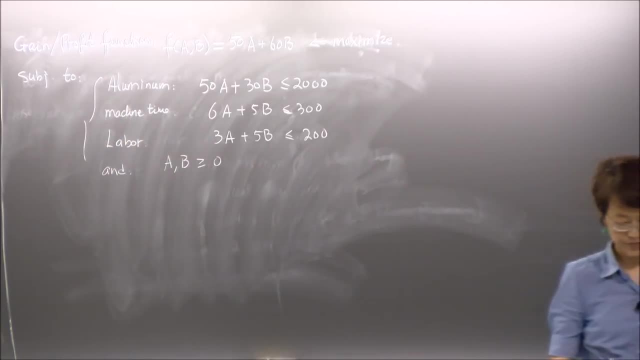 always have that okay, so always take that with you, never lose it okay. is that with you never lose it? okay? is that with you never lose it? okay, is that okay. this example: so that's a that okay. this example: so that's a that okay. this example: so that's a straightforward situation. no, 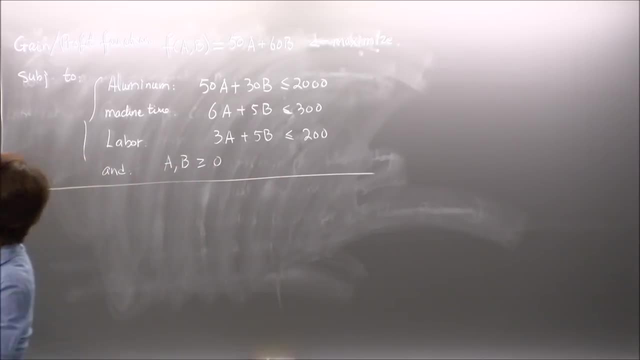 straightforward situation. no straightforward situation, no complication, nothing, complication, nothing, complication, nothing complex. just everything can be represented complex, just everything can be represented complex, just everything can be represented at this table. you carry this at this table. you carry this at this table. you carry this procedure. multiply the first by the variable a. 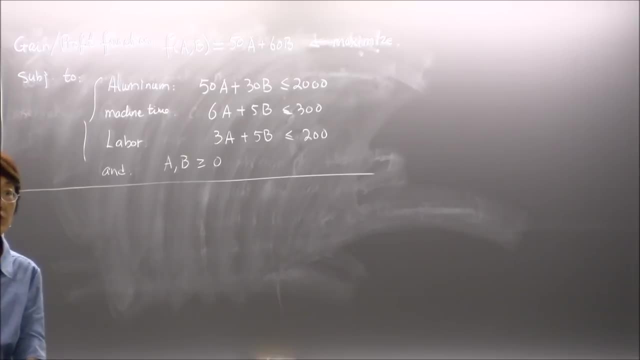 procedure: multiply the first by the variable. a procedure: multiply the first by the variable a, second by B and you add second by B and you add second by B and you add vertically to find your constraint and vertically to find your constraint and vertically to find your constraint and your kind of a gain profit function. 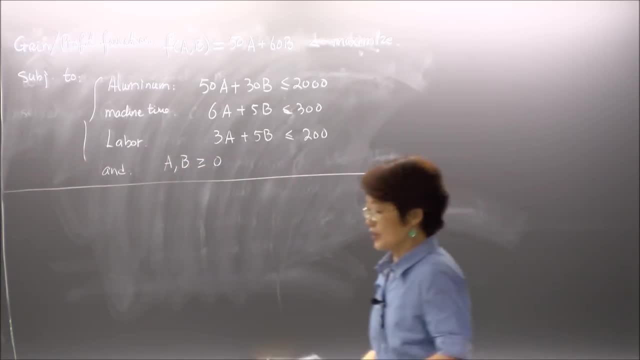 your kind of a gain profit function, your kind of a gain profit function, that's okay, okay, so that's that okay, but that's okay, okay, so that's that okay, but that's okay, okay, so that's that okay. but in real life, but in real life. 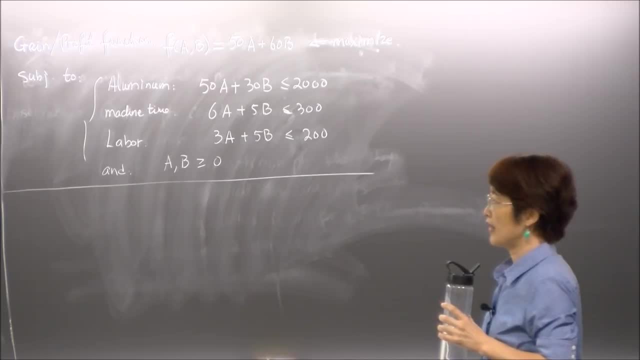 but in real life it it's always a little bit more complicated. it it's always a little bit more complicated, it it's always a little bit more complicated than that. so let's add some than that. so, let's add some than that. so let's add some complication into the problem, okay, so, 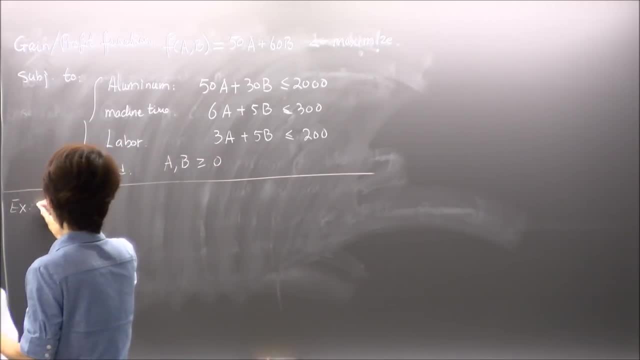 complication into the problem. okay. so, complication into the problem, okay. so, based on this problem, we're going to put: based on this problem, we're going to put: based on this problem, we're going to put something more complicated into it, something more complicated into it, something more complicated into it. that's also in in the textbook I take. 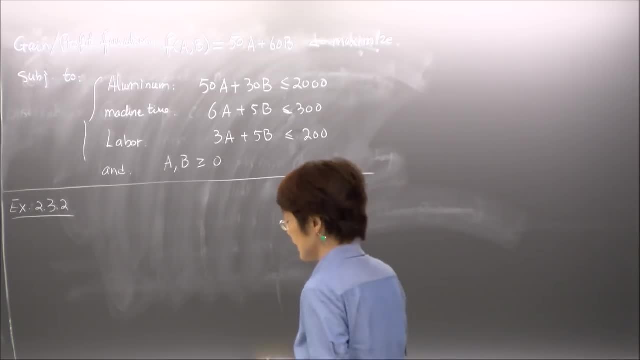 that's also in in the textbook, I take, that's also in in the textbook, I take them. so now let's say them. so now let's say them. so now let's say: there's some complication here, it's not. there's some complication here, it's not. 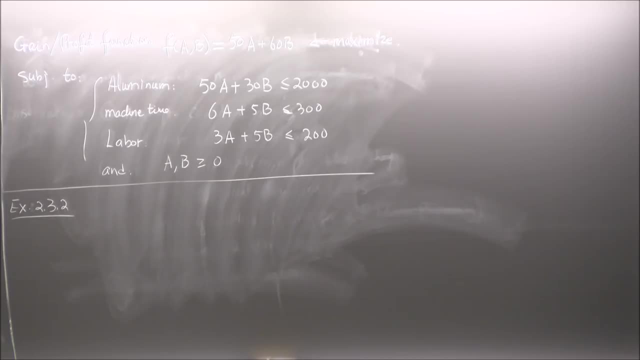 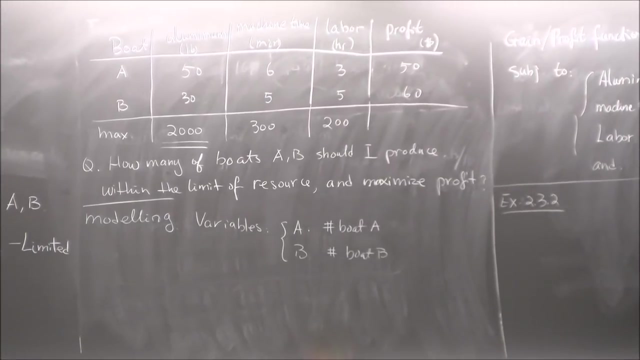 there's some complication here. it's not as simple as this one of the resource, as simple as this one of the resource, as simple as this one of the resource: this aluminum- here I still can buy this aluminum here. I still can buy this aluminum here I still can buy maximum 200 pounds, but the price will be. 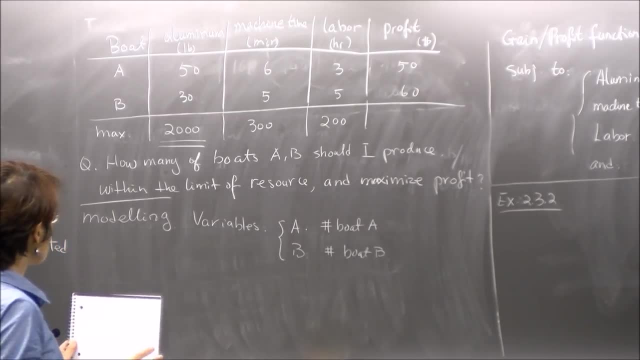 maximum 200 pounds, but the price will be maximum 200 pounds, but the price will be different. if I buy only 1,500 pounds, I different. if I buy only 1,500 pounds, I different. if I buy only 1,500 pounds, I can have it at the lower price and then. 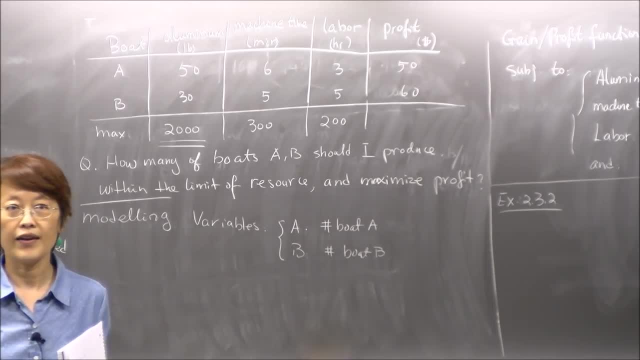 can have it at the lower price, and then can have it at the lower price, and then the last 500 pound. the price will be a the last 500 pound, the price will be a the last 500 pound. the price will be a bit higher, bit higher. 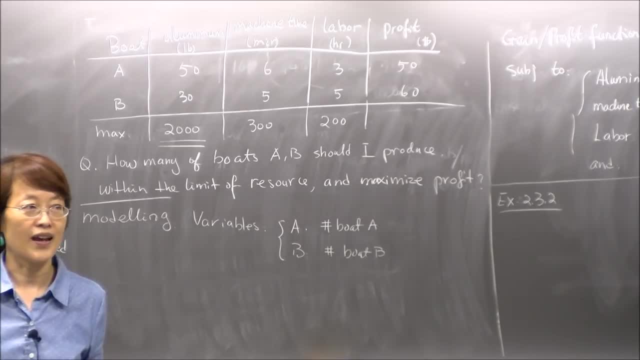 bit higher because I want too much of it. that's because I want too much of it. that's because I want too much of it. that's something that happens very commonly. is something that happens very commonly. is something that happens very commonly. is that right, okay? so let's put that in to. 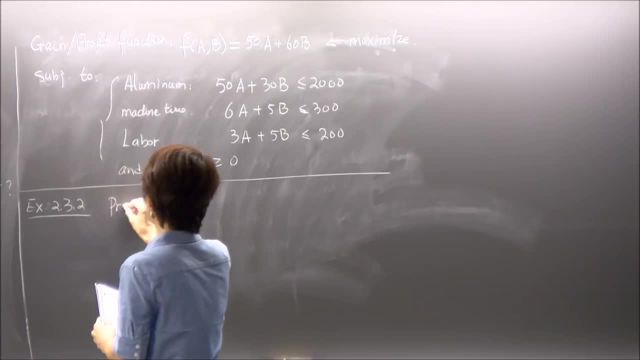 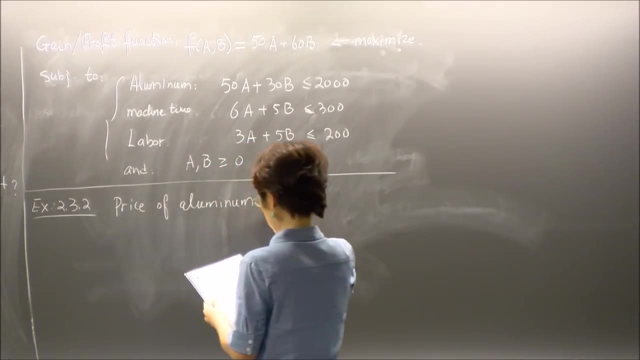 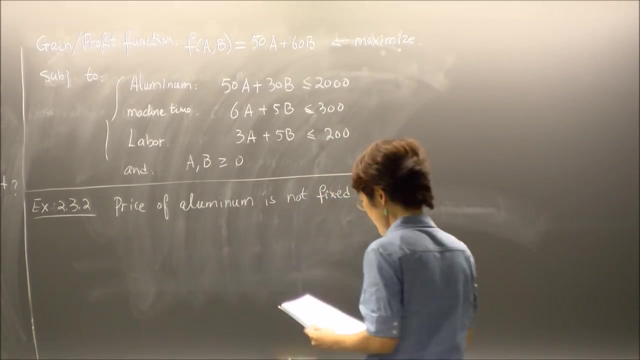 that right? okay, so let's put that in to that right. okay, so let's put that in to see how that changes, okay. so price of see how that changes: okay. so price of see how that changes: okay. so price of aluminum: aluminum: aluminum is not completely fixed, okay, it changes. 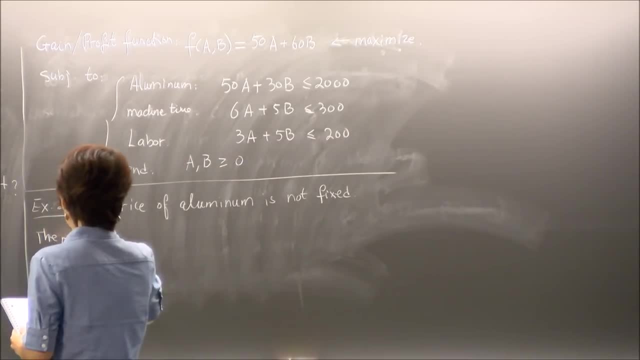 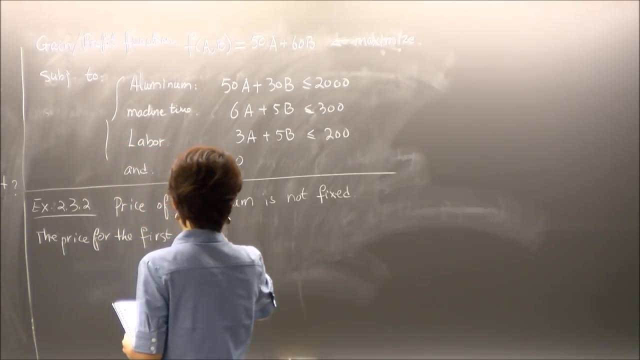 is not completely fixed, okay, it changes, is not completely fixed, okay, it changes. so let's put it, so, let's put it, so, let's put it, let's say, let's say, let's say the price for the first one: five zero, zero. the price for the first one: five zero, zero. 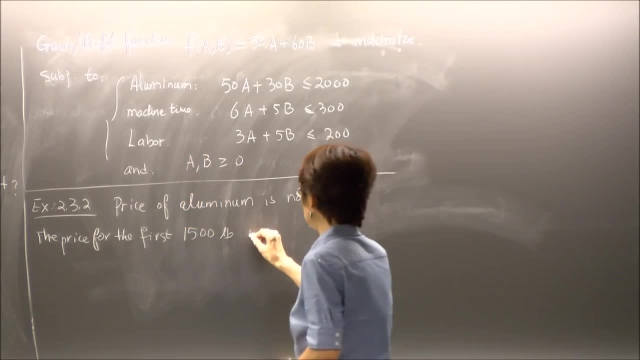 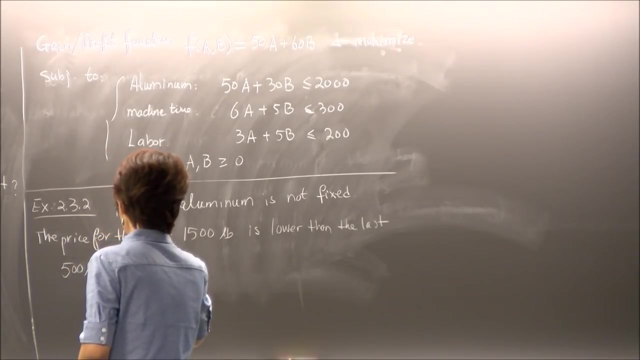 the price for the first one. five zero zero. pound is a bit lower, so is lower. pound is a bit lower, so is lower. pound is a bit lower, so is lower. then the last 500 pound, let's say by um. then the last 500 pound, let's say by um. 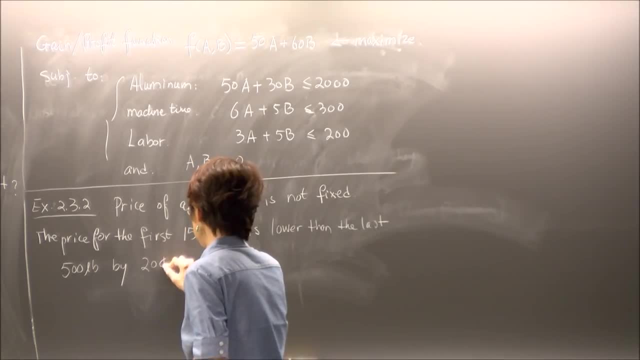 then the last 500 pound. let's say by um a few cents, let's say by 20 cents, just a few cents. let's say by 20 cents, just a few cents, let's say by 20 cents. just some number, some number, some number, okay. so for the last 500 pounds you have. 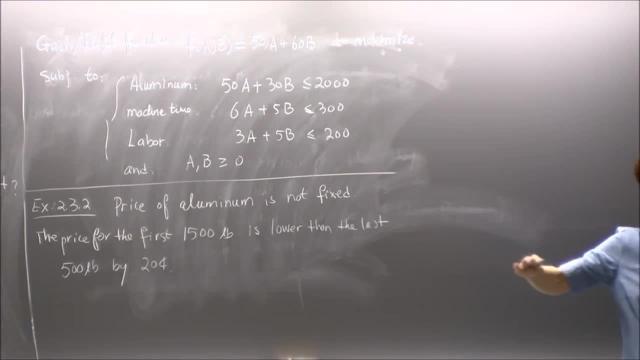 okay, so for the last 500 pounds you have. okay, so for the last 500 pounds, you have to pay 20 cents more to pay 20 cents more, to pay 20 cents more. but there's still this cap five two. but there's still this cap five two. 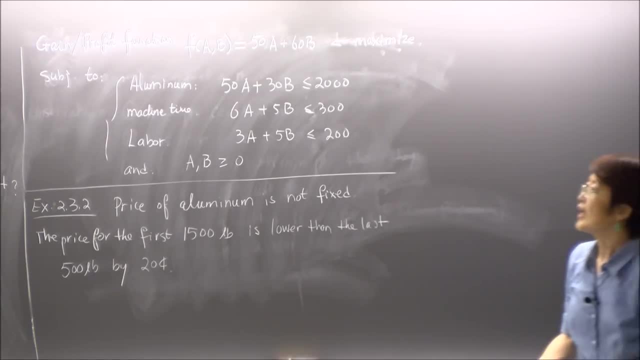 but there's still this cap: five, two thousand pounds. that's the maximum you thousand pounds, that's the maximum you, thousand pounds, that's the maximum you can buy. can buy, can buy, okay, and the profit here: okay, and the profit here: okay, and the profit here is calculated by using the lower price. 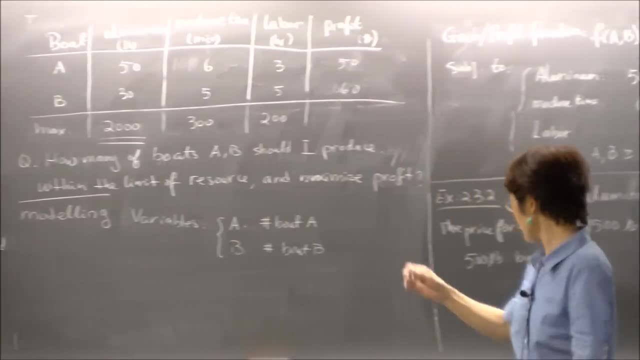 is calculated by using the lower price, is calculated by using the lower price of the aluminum, of the aluminum, of the aluminum. is that clear okay? so let me use right. is that clear okay, so let me use right. is that clear okay, so let me use right there. so the price. 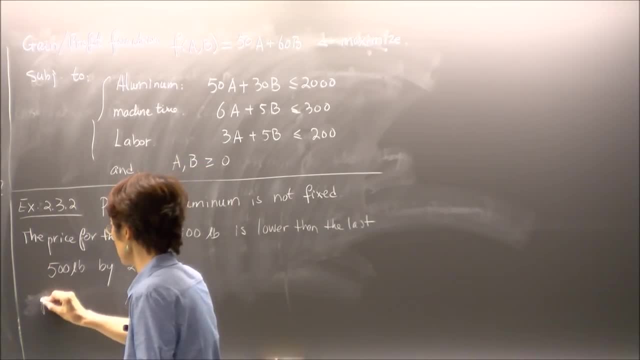 there. so the price there, so the price in the table there, the profit there. let in the table there the profit there. let in the table there the profit there. let me see the profit, me see the profit, me see the profit. the profit listed there is obtained by: 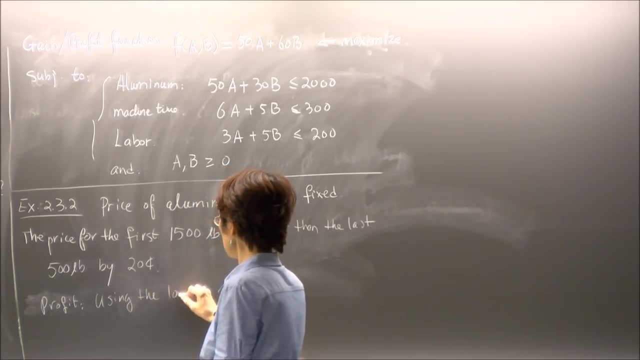 the profit listed there is obtained by. the profit listed there is obtained by using: using: using the lower, the lower, the lower aluminum price. okay, so how can we set up? okay, so, how can we set up? okay, so, how can we set up? so it's the same setting. 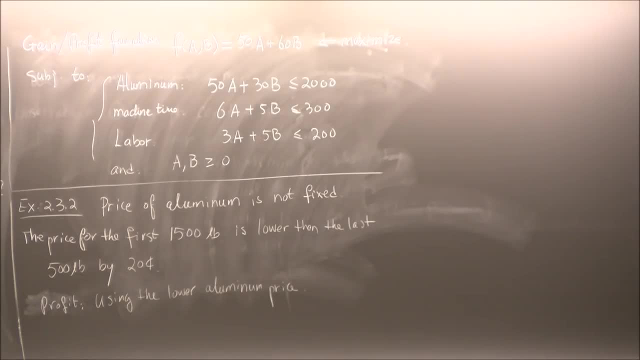 so it's the same setting. so it's the same setting. a- a- a same question. how many of both type? a same question. how many of both type? a same question. how many of both type? a and b? should i produce and b should i produce and b should i produce so that it's within the 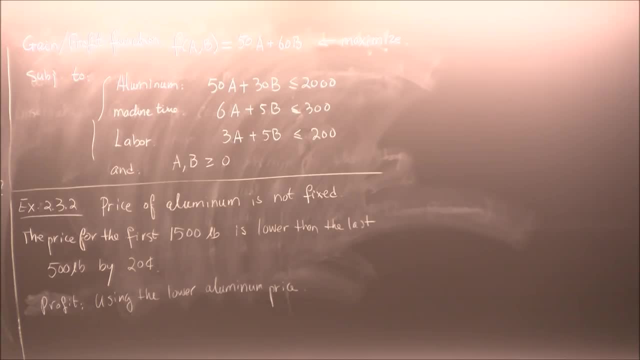 so that it's within the, so that it's within the resource, resource, resource limitation, and i want to maximize my limitation and i want to maximize my limitation and i want to maximize my profit, profit, profit. okay. so you see it's a little bit okay. so you see it's a little bit. 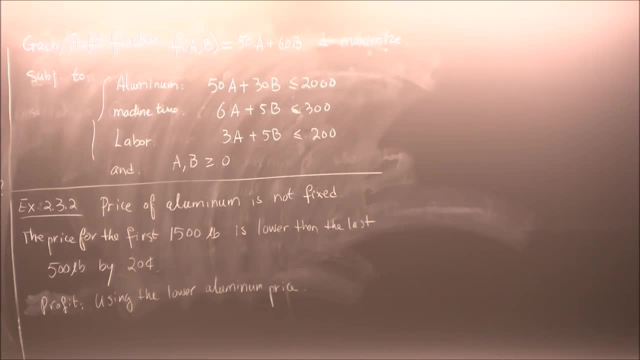 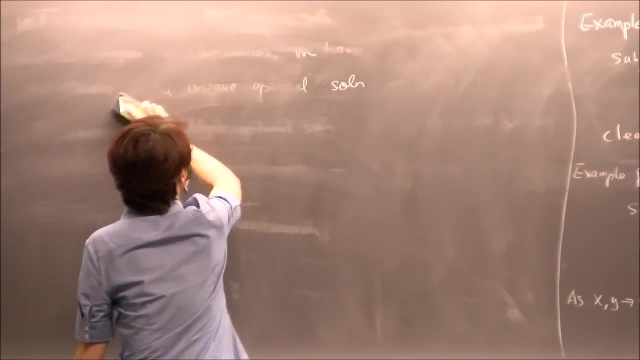 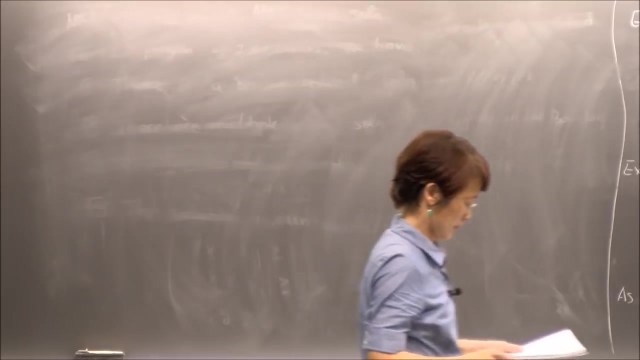 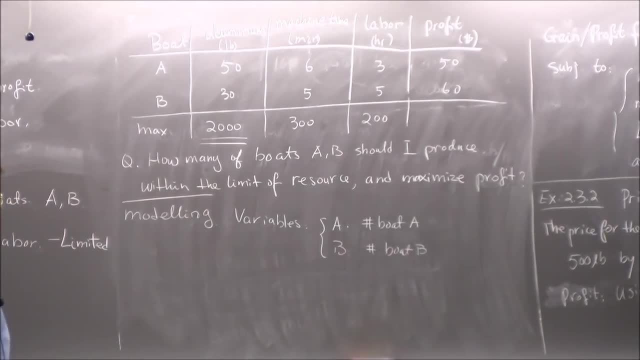 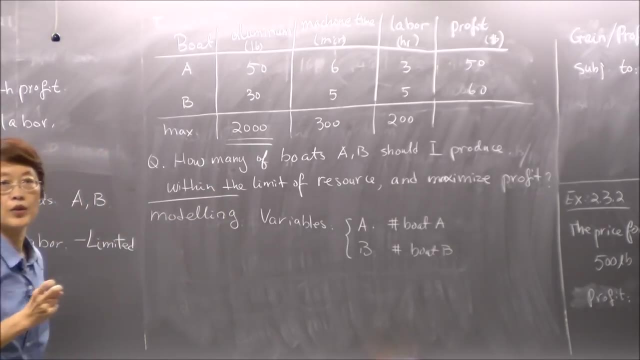 so here, besides the decision how many boats, boats, boats i should produce, i should produce, i should produce, i have another decision, i have another decision. i have another decision, that is that is, that is: how do i use the aluminum right? should i? how do i use the aluminum right, should i? 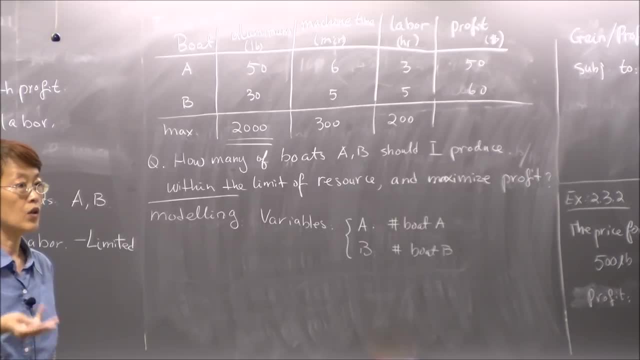 how do i use the aluminum right? should i use more than use more than use more than 1 500 pound, or should i not use that 1 500 pound? or should i not use that 1 500 pound? or should i not use that right, and how much more over 1 500 pound? 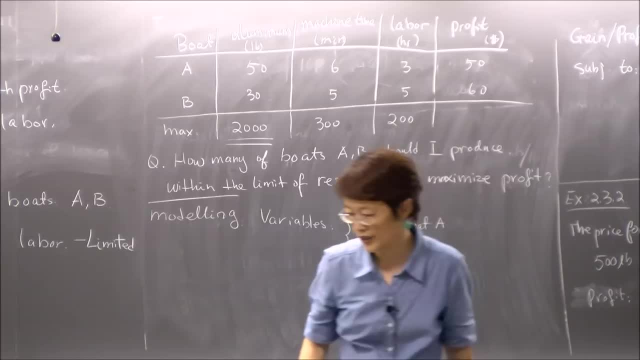 right and how much more over 1 500 pound? right and how much more over 1 500 pound should i use? should i use? should i use? is that right? so i have a third thing to. is that right? so i have a third thing to. 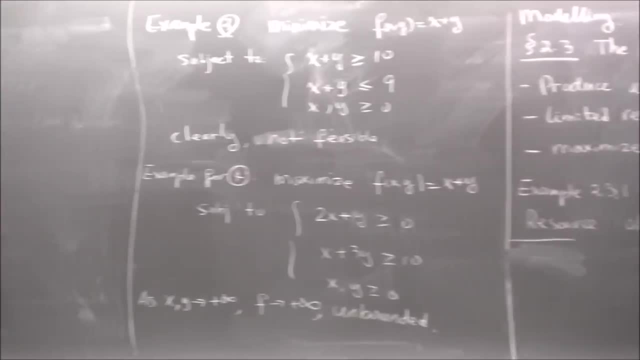 is that right? so i have a third thing to decide. then let's introduce another. decide, then let's introduce another. decide, then let's introduce another variable, variable variable. so let now this variable x, i introduce a. so let now this variable x, i introduce a. so let now this variable x, i introduce a new one. okay, 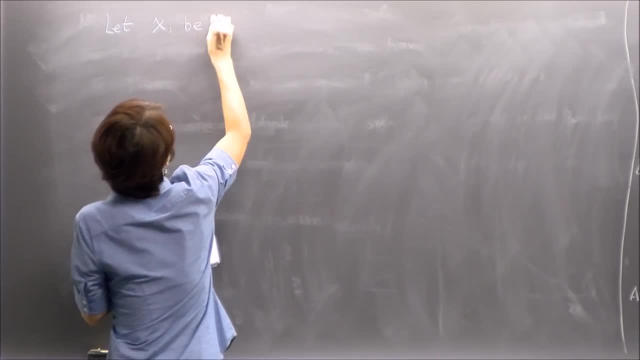 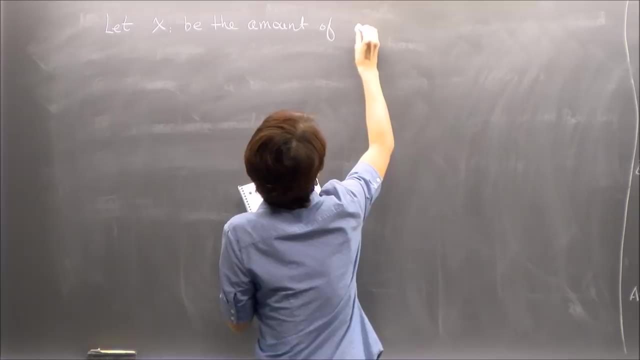 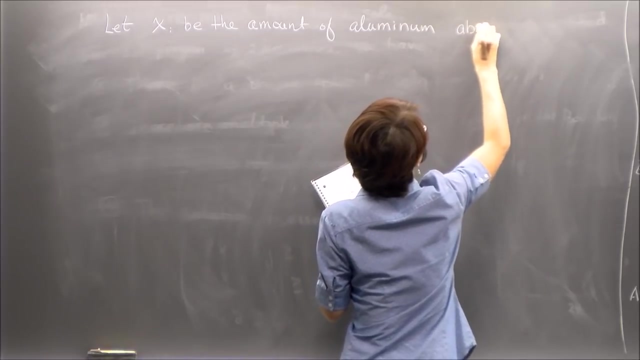 new one, okay, new one. okay, be exactly this decision. so be exactly this decision, so be exactly this decision. so that will be the, that will be the. that will be the amount of amount of amount of aluminum above, above above 1 500: 1 500. 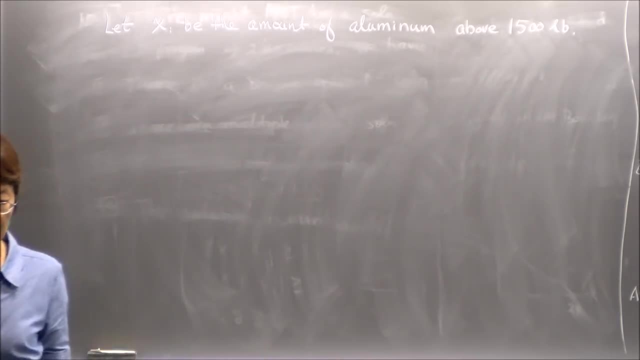 1 500 pound. pound, pound. so watch carefully the wording here. so watch carefully the wording here. so watch carefully the wording here. x is the amount of aluminum above 1 500. x is the amount of aluminum above 1 500. x is the amount of aluminum above 1 500 pound. 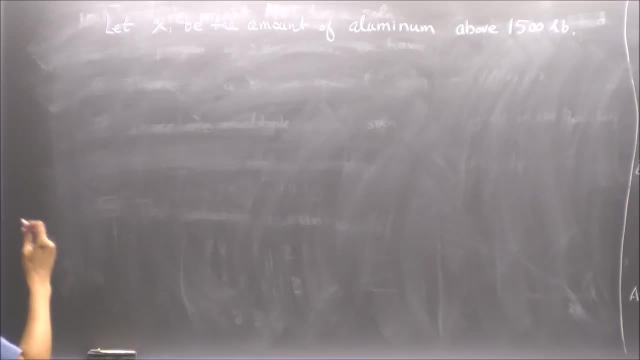 pound, pound. it will come into the picture only if i. it will come into the picture only if i. it will come into the picture only if i use, use, use more than 1 500 pound. if i use less more than 1 500 pound, if i use less. 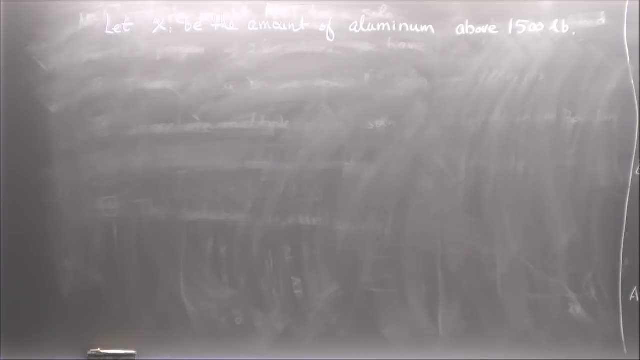 more than 1 500 pound if i use less. x is zero, it's not negative. x is zero, it's not negative. x is zero, it's not negative. is that clear? so i want to catch your. is that clear? so i want to catch your. is that clear? so i want to catch your attention here. so here, 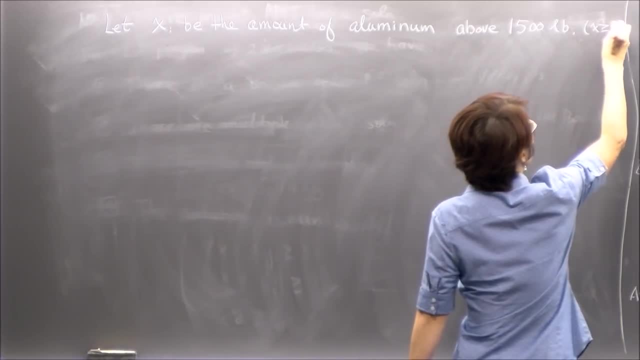 attention here, so here. attention here, so here. i am implying that x cannot be. i am implying that x cannot be. i am implying that x cannot be negative. i don't consider that negative. i don't consider that negative. i don't consider that okay. okay, let's see how we can change. 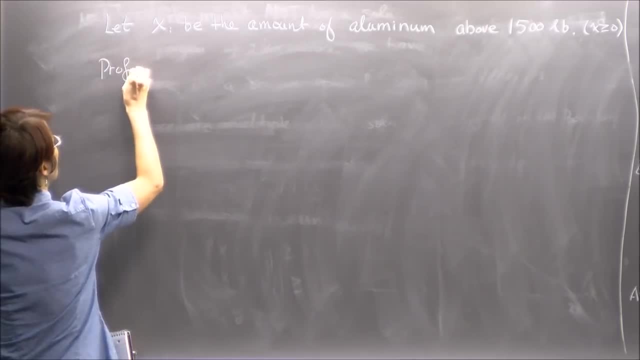 okay, okay, let's see how we can change. okay, okay, let's see how we can change our model, our model, our model. so what will be my? so, what will be my? so what will be my? profit function, profit function, profit function in this case. okay, probably i should write. 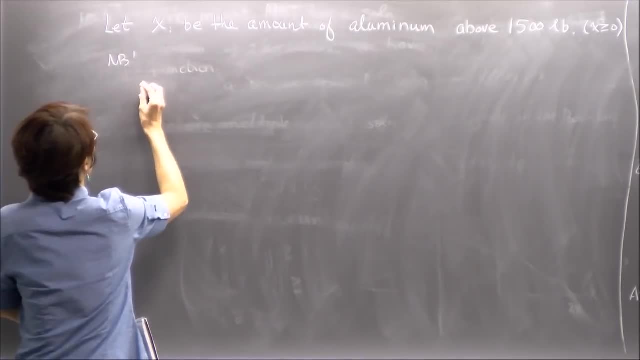 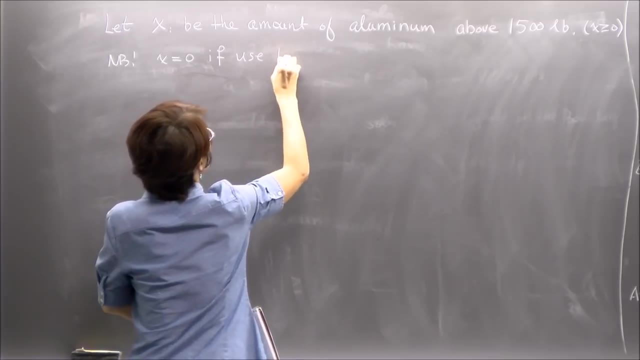 in this case: okay, probably i should write. in this case, okay, probably i should write. write this as: pay attention x will be zero. if pay attention x will be zero. if pay attention x will be zero if use less, use less. use less than one five zero, zero pound. 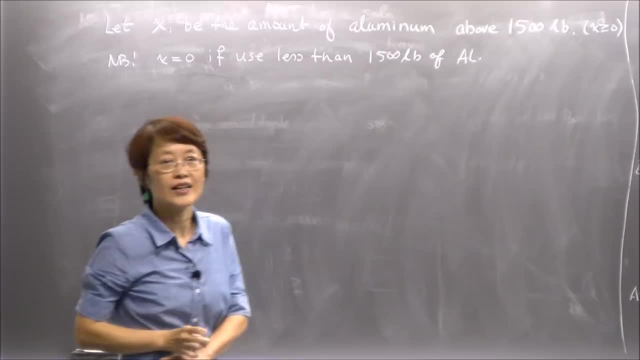 than one five zero zero pound, than one five zero zero pound of the aluminum, of the aluminum, of the aluminum. is that clear okay? so keep that okay. so is that clear okay? so keep that okay. so is that clear okay? so keep that okay. so now i'm going to write my 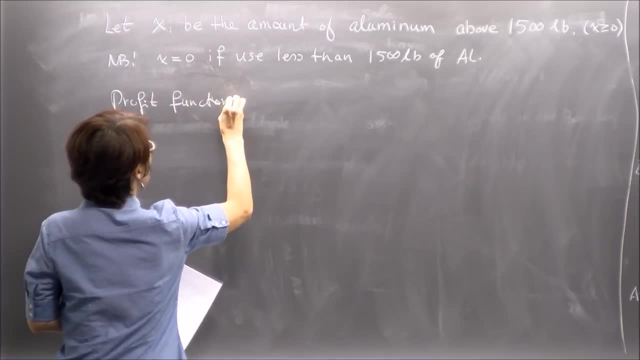 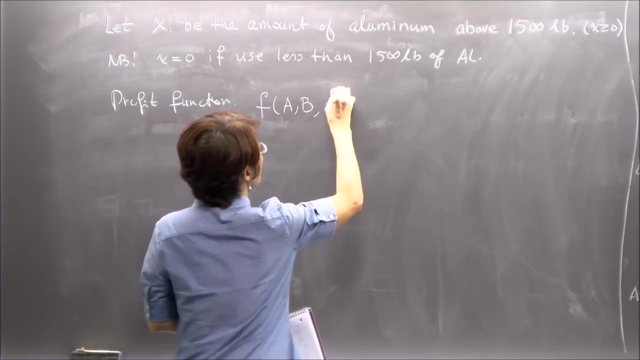 now i'm going to write my. now i'm going to write my profit function, profit function, profit function. now the profit function depends on a. now the profit function depends on a. now the profit function depends on a, b, b, b and also this x, because that's the part. 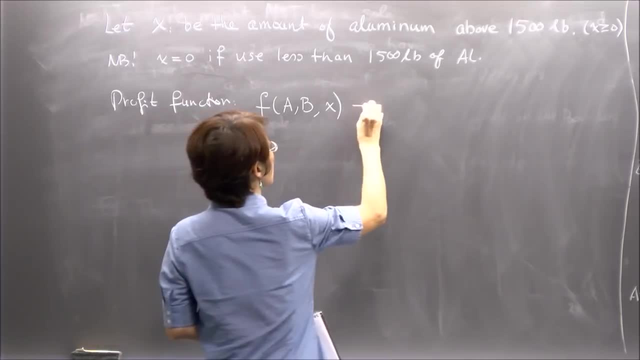 and also this x, because that's the part, and also this x, because that's the part, incurs an extra cost for me. is that incurs an extra cost for me? is that incurs an extra cost for me? is that right, right, right? so what will be the profit function? how? 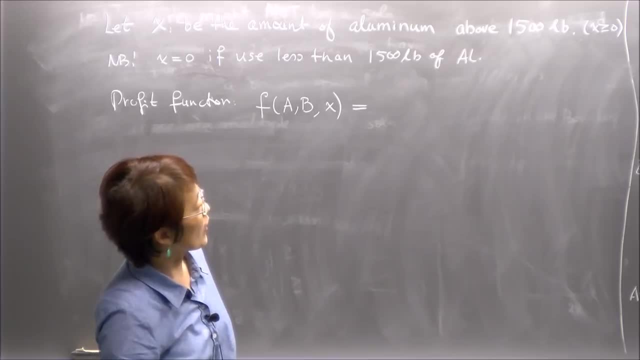 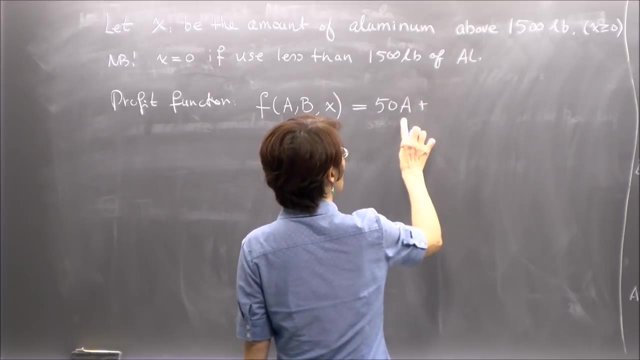 so what will be the profit function? how? so what will be the profit function? how should i, should, i should i change it from, change it from change it from the model i had there the model i had there, the model i had there. so so so i will have 50 a the profit for making. 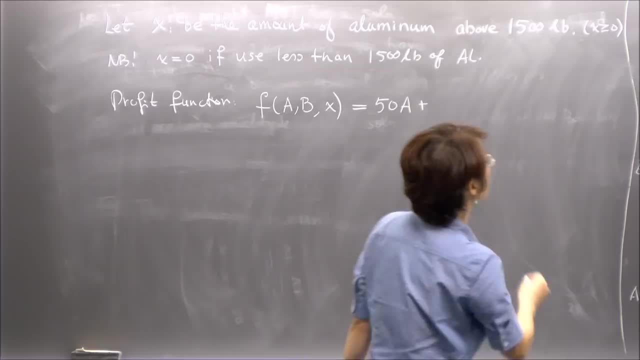 i will have 50 a the profit for making. i will have 50 a the profit for making both a, both a, both a. is that right? is that 60, hopefully? is that right? is that 60, hopefully? is that right? is that 60, hopefully? the other one is a 40, i can't see. 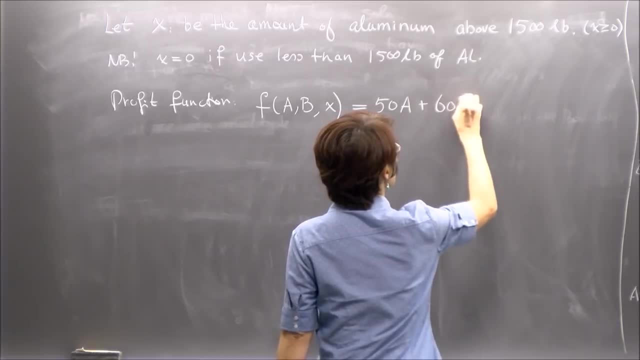 the other one is a 40, i can't see. the other one is a 40. i can't see 60, 60, 60 and 60 and 60 and 60, b, b, b. that will be the profit if i sell those. that will be the profit if i sell those. 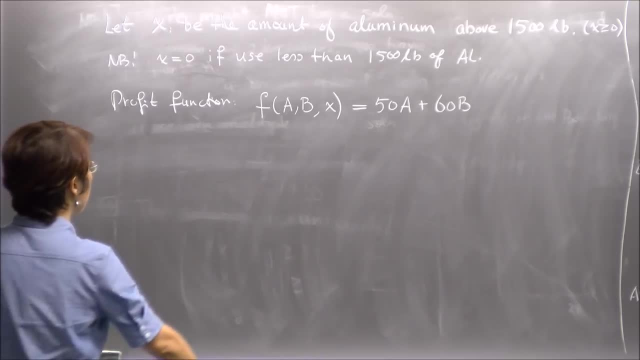 that will be the profit if i sell those votes which i assume i can, votes which i assume i can, votes which i assume i can. but then if the x shall be numb, but then if the x shall be numb, but then if the x shall be numb, bigger than strictly, bigger than zero, i 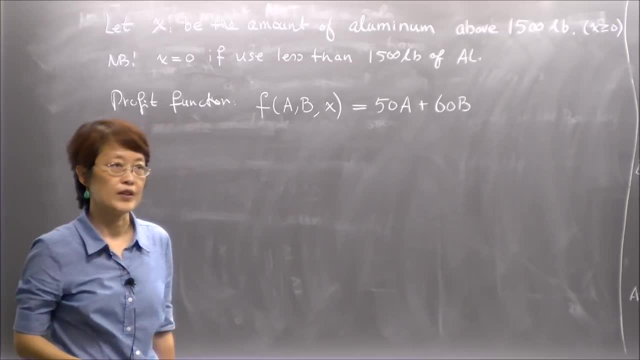 bigger than strictly bigger than zero. i bigger than strictly bigger than zero. i used more, used more, used more. this would take away some of my profit. this would take away some of my profit. this would take away some of my profit. is that right so? is that right so? 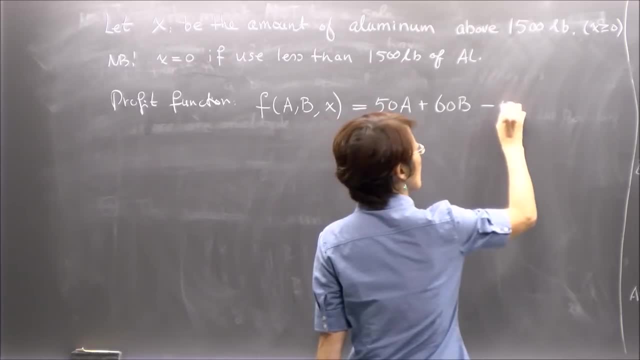 is that right? so i should take that away. is that right? i should take that away. is that right? i should take that away. is that right? so for each pound, so for each pound, so for each pound of x, it costs 20 cents of x, it costs 20 cents. 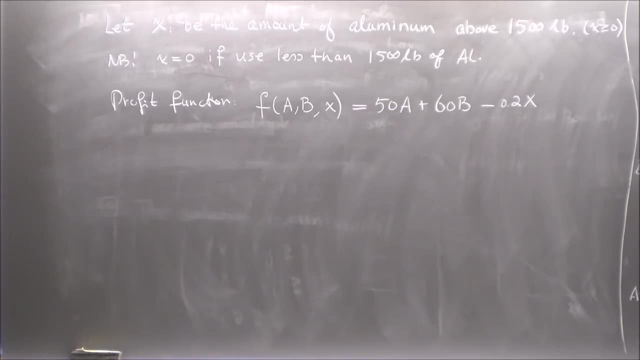 of x, it costs 20 cents so that i should remove from my profit, so that i should remove from my profit, so that i should remove from my profit. does that make sense? does that make sense? does that make sense? so this is the new part. so this is the new part. 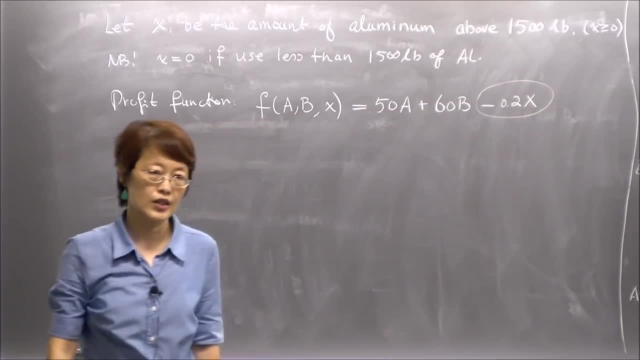 so this is the new part. i'm going to circle it, i'm going to circle it, i'm going to circle it. that's the new part. the change in the: that's the new part. the change in the: that's the new part. the change in the cost, in the profit function. 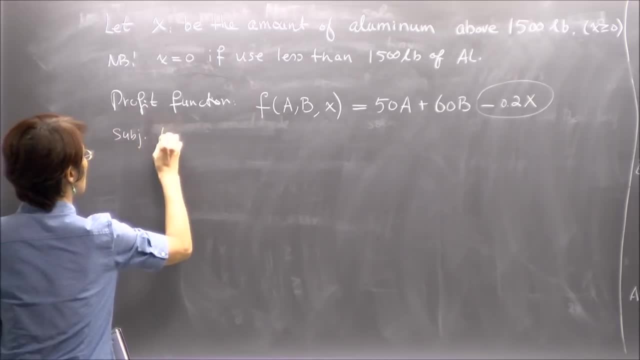 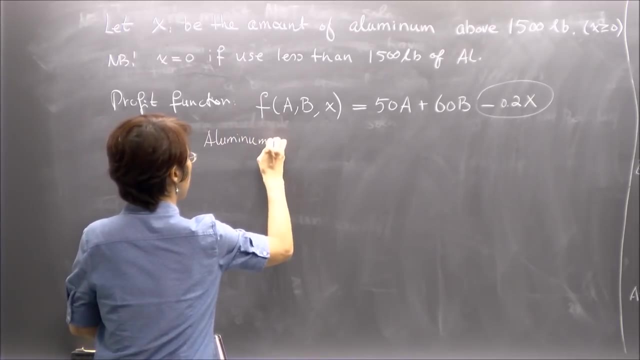 cost in the profit function okay, so subject to okay, so subject to okay, so subject to all these constraints so aluminum, all these constraints so aluminum, all these constraints so aluminum. okay, so how should i write out my okay? so how should i write out my okay? so how should i write out my aluminum constraint? 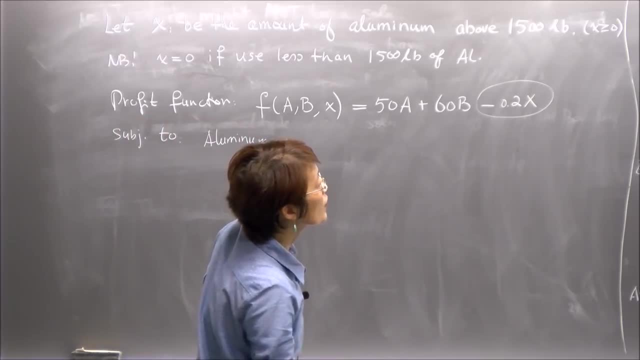 aluminum constraint, aluminum constraint. so the total aluminum i will be using. so the total aluminum i will be using. so the total aluminum i will be using is 50, 30, so is 50, 30, so is 50, 30, so 50, 50, 50 a plus. 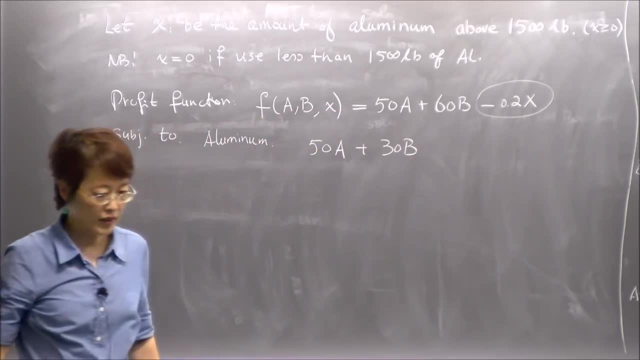 a plus a plus 30 b, 30 b, 30 b- that will be the aluminum. that will be the aluminum. that will be the aluminum i would need to produce that amount of, i would need to produce that amount of. i would need to produce that amount of votes. 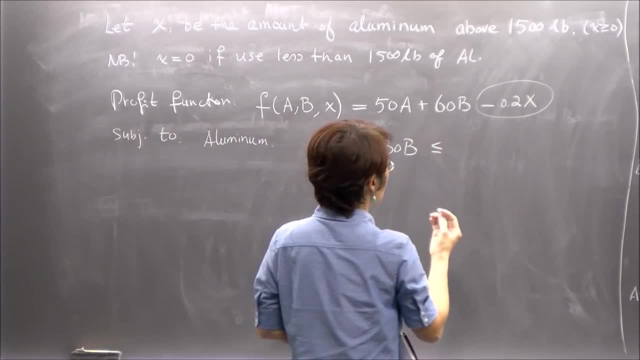 votes, votes, and then i know that this shall be less, and then i know that this shall be less, and then i know that this shall be less than than than. the earlier is 2000, but now i have to. the earlier is 2000, but now i have to. 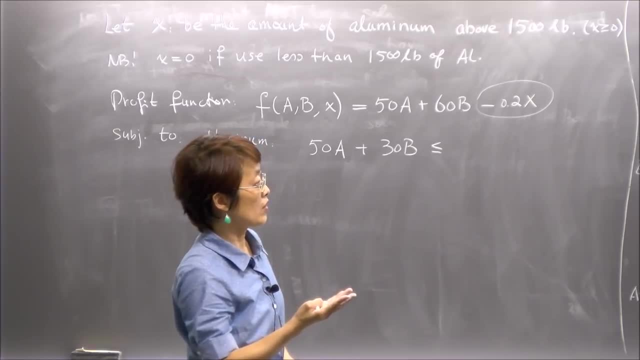 the earlier is 2000. but now i have to make a distinction of if it is above 1500, make a distinction of if it is above 1500. make a distinction of if it is above 1500 or not, or not or not. is that right? so 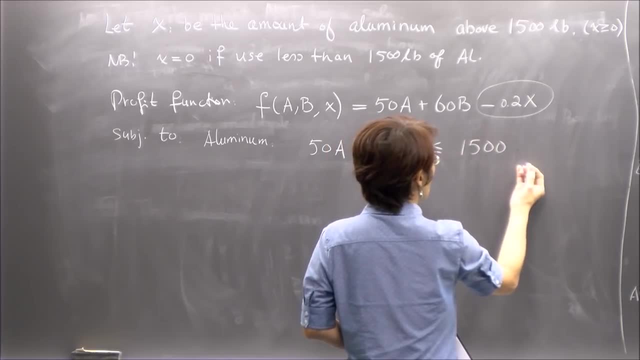 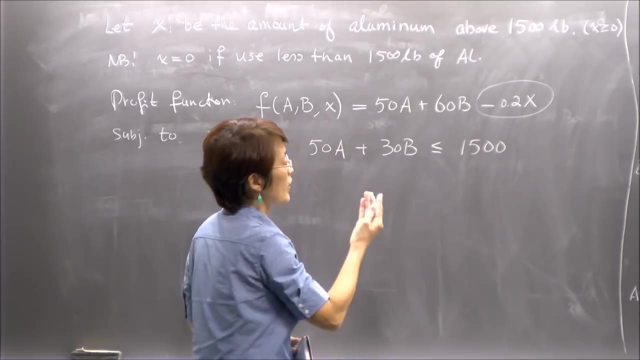 is that right? so, is that right? so let me say, let me say, let me say, this is less than 1500. if x is zero, if i don't go above it, if x is zero, if i don't go above it, But if I go above it, then x is positive, then this should be equal to 1,500 plus x. 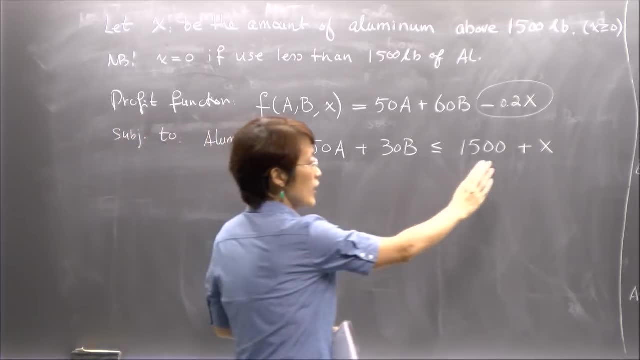 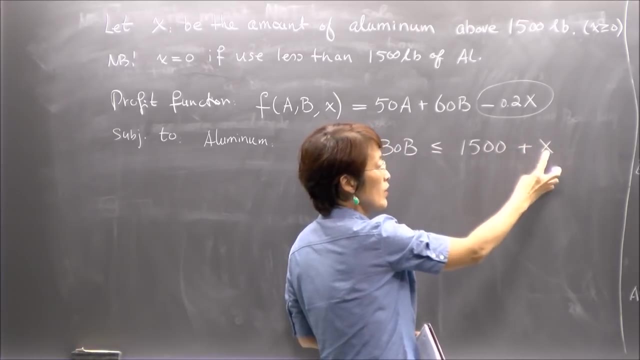 Is that right? Does that make sense? So think again. If x is 0, I will have less than or equal sine. right. If x is positive, so I'm using more than that and I will have an equal sine. 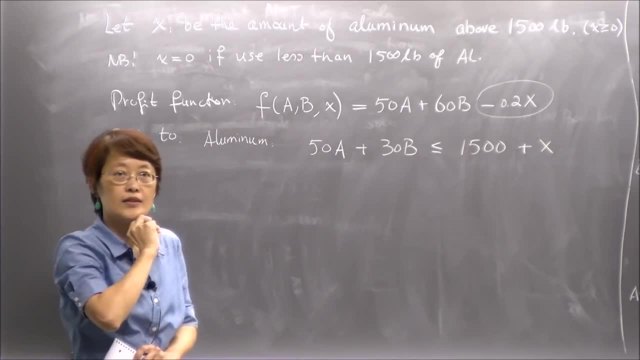 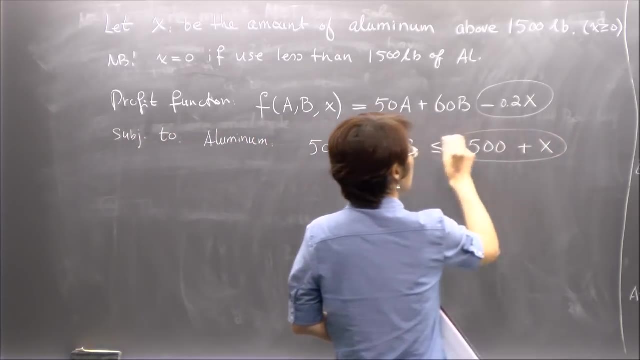 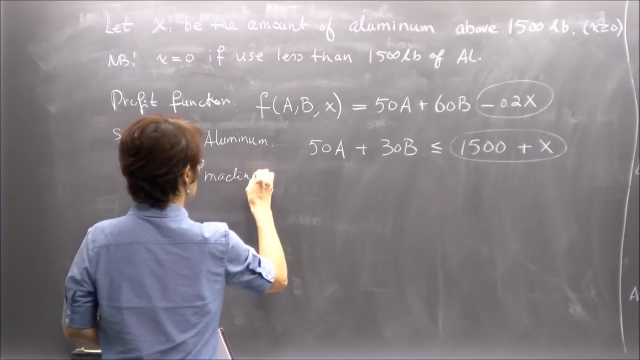 But that's included in the less than or equal sine. So this will be the final constraint. Is that okay? So this is different. Let me circle. This is different from the previous model, the simple one. Okay, and then I have machine hour and labor. 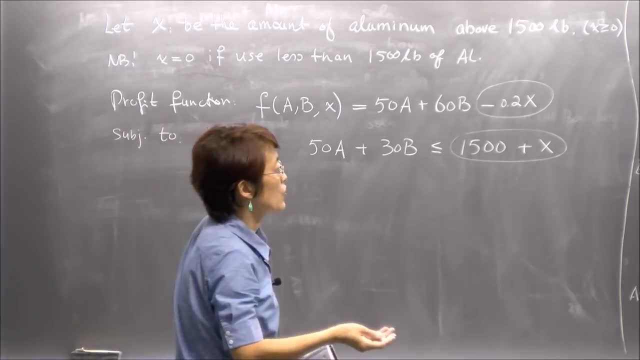 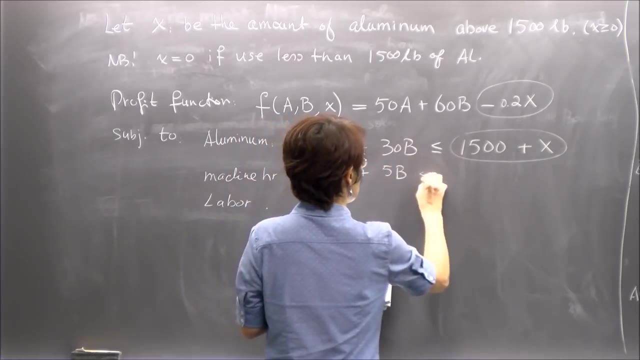 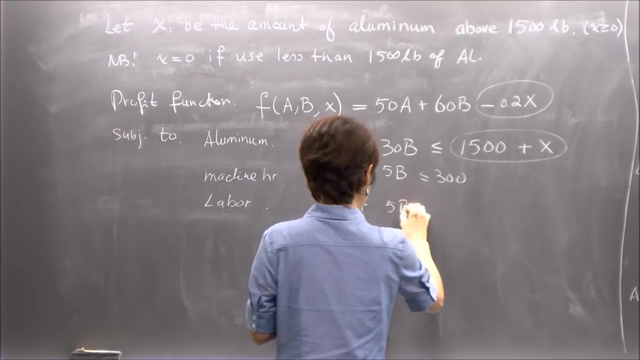 And those two constraints are not touched, so they are the same. So let me copy: 6a plus 5b less than 300. And 3a plus 5b- 5b less than 200. So I will say these two are the same, unchanged, because it didn't do anything. 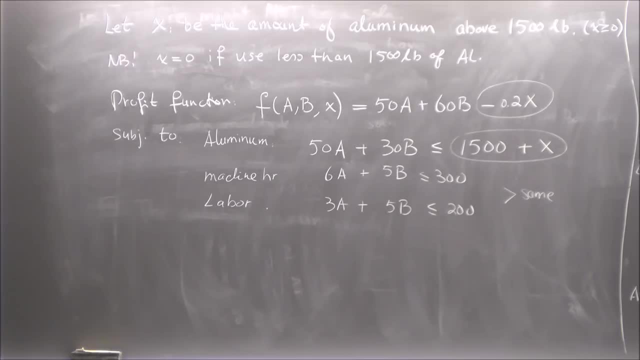 What more should I add into this picture? Mm-hmm, Do we have a? We did not take into consideration that the total aluminum is 2,000 pounds. Is that right? So what does that say to my variable x Louder? 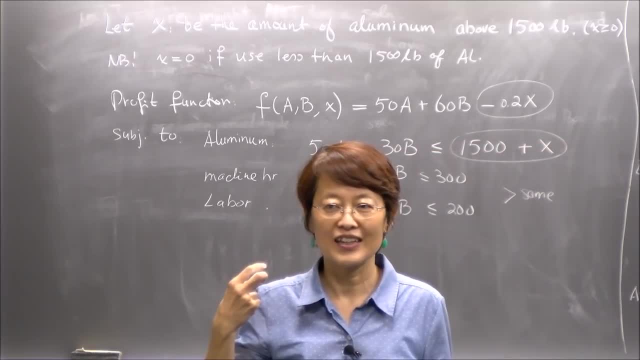 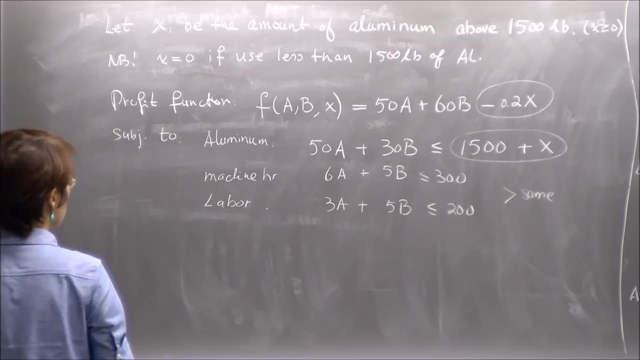 Someone whispered here, Can I hear it again? x has to be Yeah, Is that clear? Whatever, you can go above 1,500.. 1,500?, 1,500?, 1,500?, 1,500?. 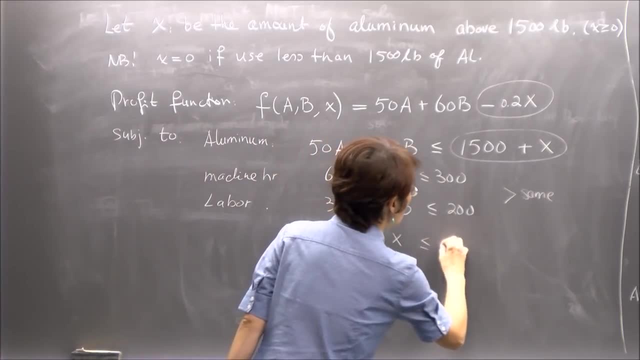 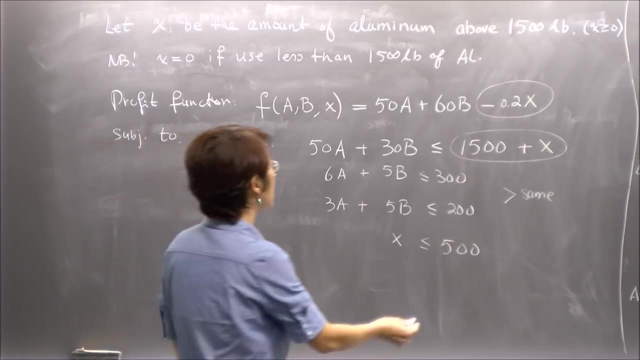 1,500? 1,500? That's fine, but the total has to be less than 500 pounds, That's above 1,500.. Is that clear? So this is also a new part coming in this model. All right. 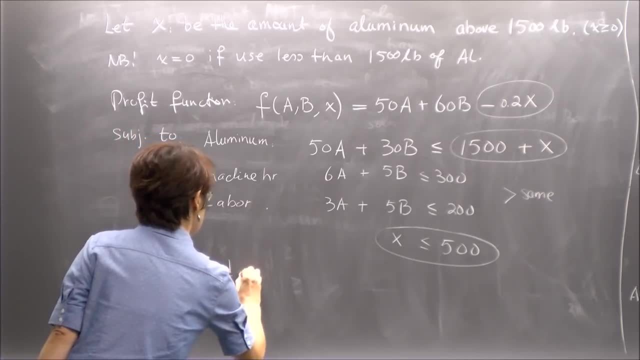 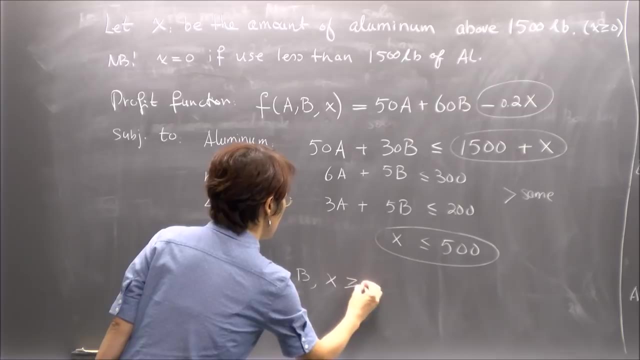 And then, of course, always, always, don't forget the non-negativity. So a, b and x, they are all non-negative variables, Is that okay? Okay, So, do we have the textbook? Have we bought it? 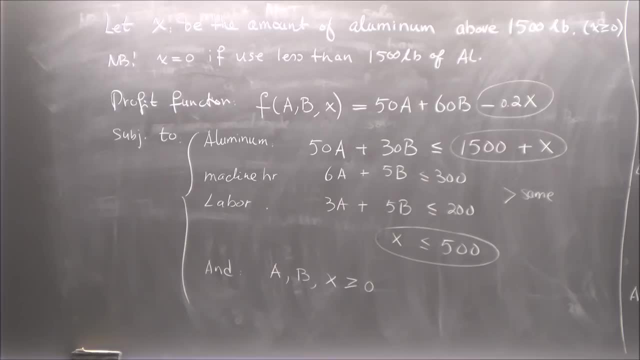 Have we got a hold on it Now? the textbook has so many many examples and I don't think I will go through all of them. some of them I would just assign as like homework and you go and read it. will that be okay? they're kind of a similar, but you might benefit from reading more.